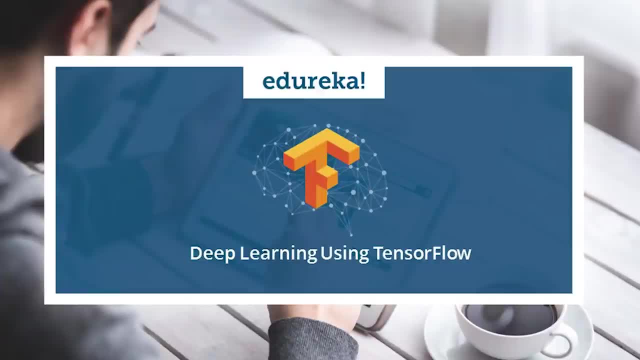 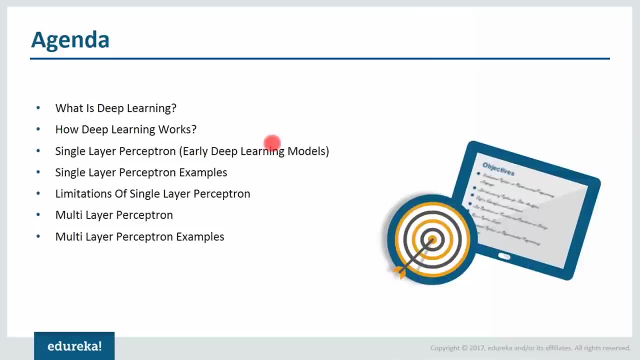 Hello everyone, this is Saurabh from Edureka and welcome to today's session on deep learning tutorial with TensorFlow. So let us move forward and have a look at the agenda for today. So this is the agenda for today. guys will understand what exactly is deep learning. 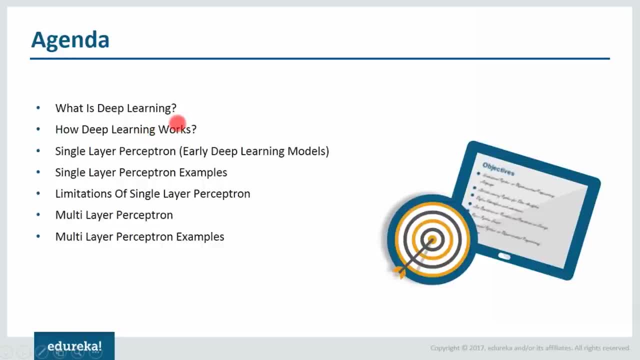 and how it works. So we'll look at the motivation behind deep learning and how it actually evolved. then we'll focus on single layer perceptron, which are nothing but the early deep learning models. We'll also look at various examples of single layer perception. and, guys, when I talk about perception, these are nothing. 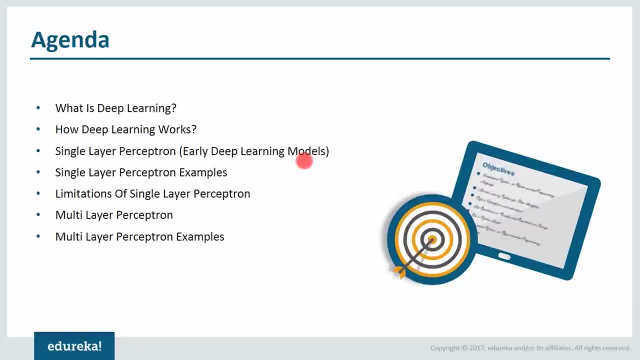 but the artificial neurons. and what are neurons? neurons or your brain cells? then we'll also understand the limitations of single layer perception that led to the evolution of multi-layer perception, will understand how multi-layer perception overcame those limitations and will also look at various examples of multi-layer perception. in the beginning. 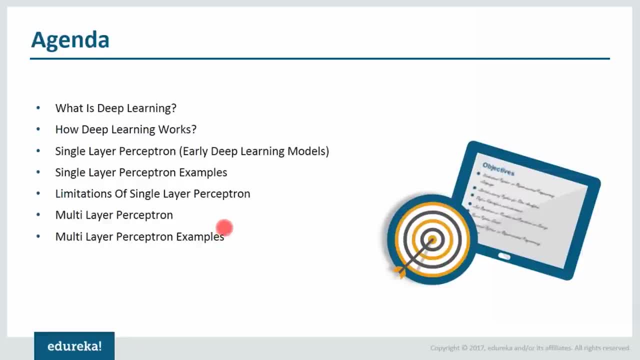 I'll be also talking about the core structure, how the course is structured, What all topics will be covered in, what all modules. so I hope you all are clear with the agenda. Just give me a quick confirmation by writing down in your chat box or if you have any questions. 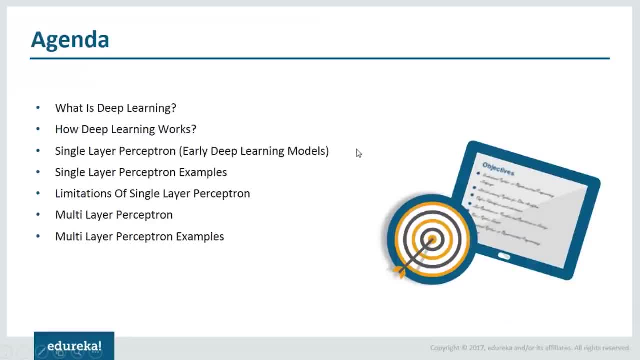 Questions or doubts you can ask me. Akshay says he's clear. So does Emma, Imran, Neha, Pragati, Pooja, Jack or a fine guys. So everyone's clear. So let us move forward and see how the course is structured. 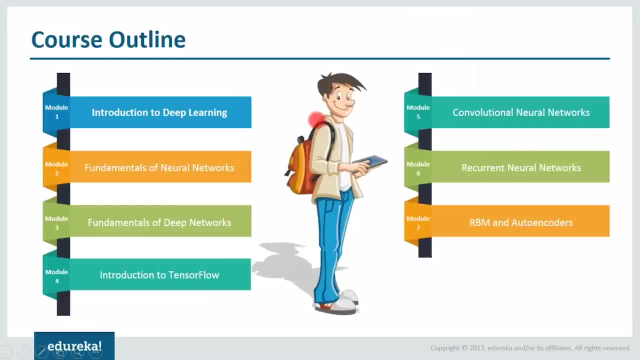 What are the various modules? So this is how our course looks like. we'll start with the introduction to deep learning. That is how deep learning evolved. What were the algorithms that were present before deep learning? then we'll understand the fundamentals of a neural networks. neural networks. 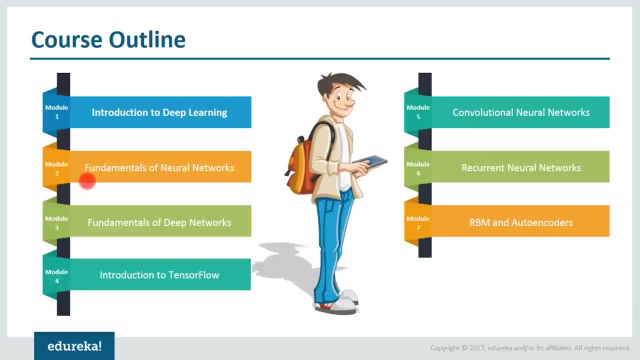 are nothing but the networks that try to mimic your brain. then will understand the fundamentals of deep networks: deep networks and nothing but complex neural networks, or you can even say that these are subsets of neural networks. then will introduce you to tensorflow, which is nothing but a library of python that is used for deep learning. 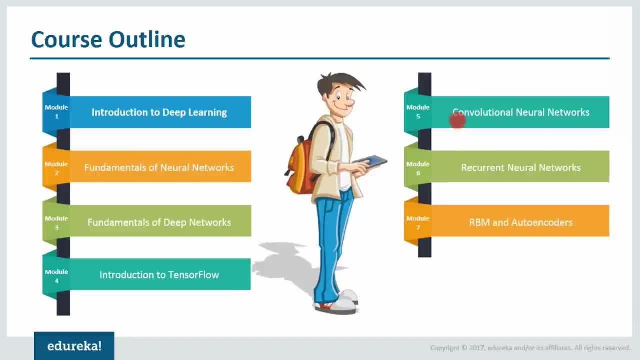 then will focus on various types of neural networks versus convolutional neural networks. that is used for image recognition, then will focus on recurrent neural networks and then, finally, RBM and auto encoders. So this is how our course will be structured. fine guys, Let us move forward and understand what all things we have understood so far. 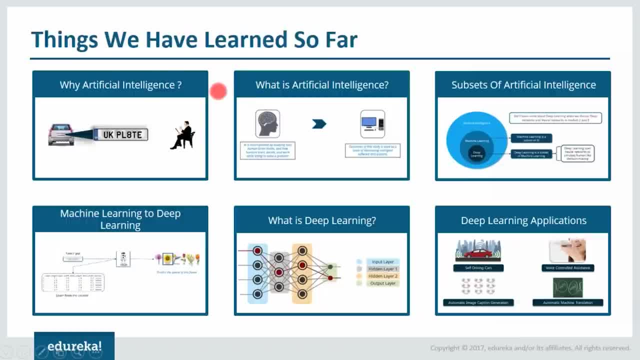 So, guys, these are the things that we have studied in the previous session. We first understood why artificial intelligence, What is the need of artificial intelligence. Then we saw what exactly it is, and we also focused on various subsets of artificial intelligence, That is, machine learning and deep learning. 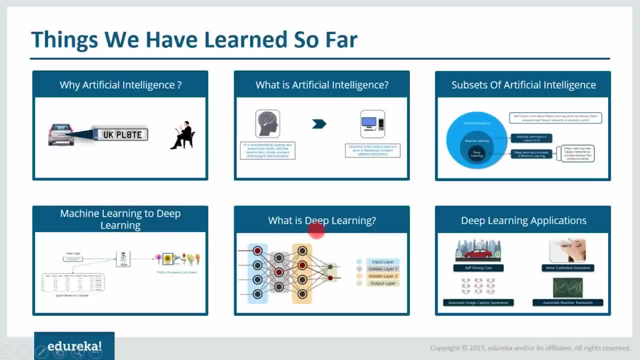 Then we understood how we came from machine learning to deep learning and we saw what exactly is deep learning, along with various applications of deep learning. So guys will move forward now and understand what exactly is deep learning and how it works. So, guys, let us understand deep learning with an analogy. 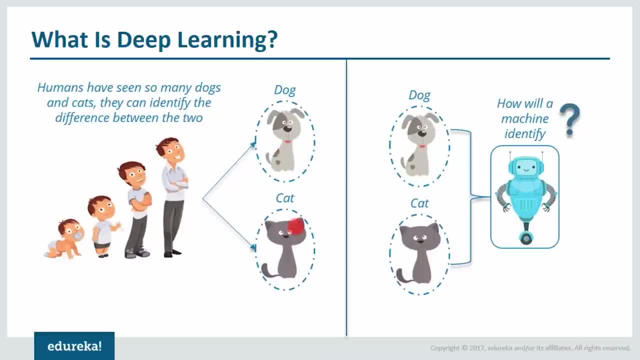 So how do you think our brain is able to identify the difference between a dog and a cat? The reason is, since the day we are born, we are actually seeing different types of cats and dogs in a day-to-day life, and because of that we are able to identify the difference. 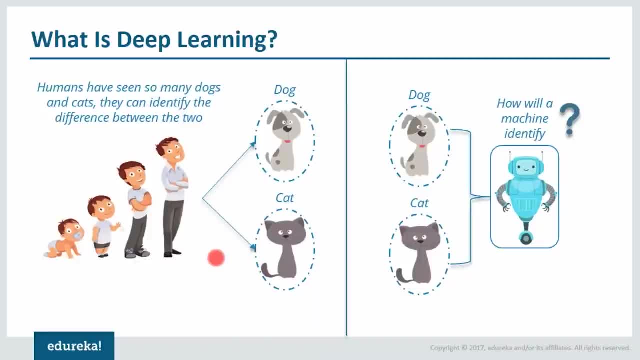 or spot the difference between the two, that is, dog and a cat. Even if we see different types of cats and dogs, we still know which is a cat and which is a dog. So this is because we have seen a lot of cats and dogs in our entire life. 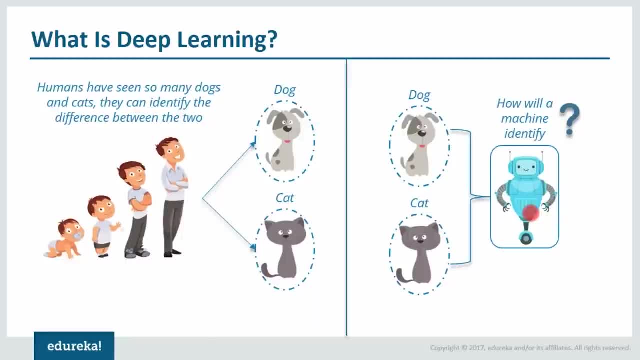 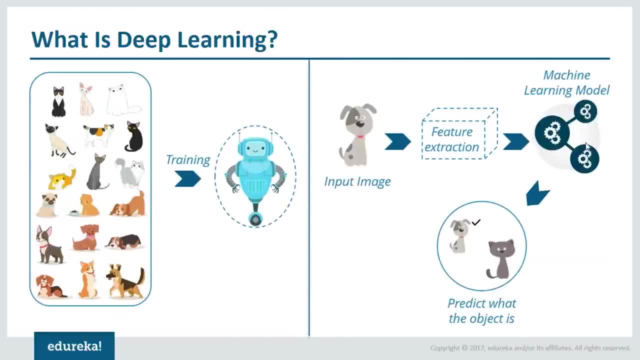 But what if I want a machine to do that task for me? So how will a machine identify whether the given image is of a dog or a cat? So one way of doing that is, we can train our machine to a lot of images, a lot of images of different cats and dogs. 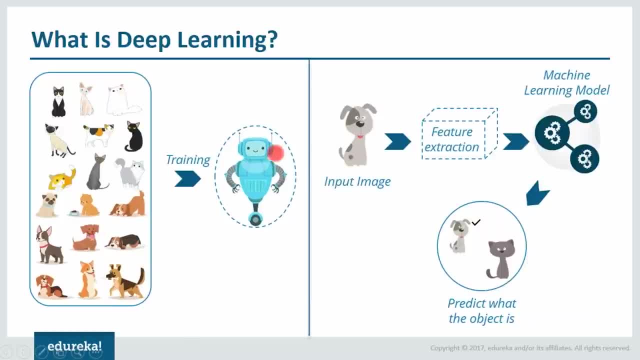 that is, different breeds of cats and dogs. and then what will happen once our training is done? We can provide it with an input image, then will manually extract certain features, Features like nose, whiskers, colors, edges- It can be anything- the important features, which actually helps us in classifying. 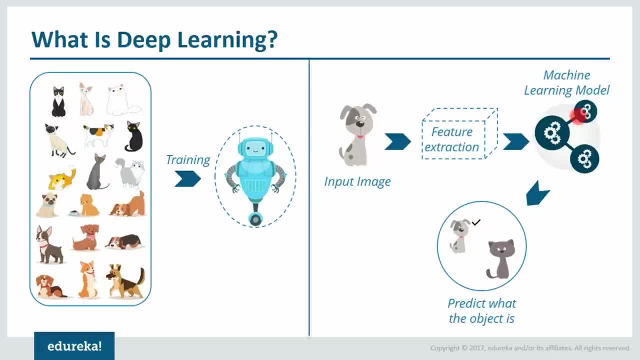 whether the input image is a cat or a dog, Then we make a machine learning model with that and once it is done our machine learning model is able to predict whether the input image is of a cat or a dog. But if you notice here, one very big disadvantage with this is 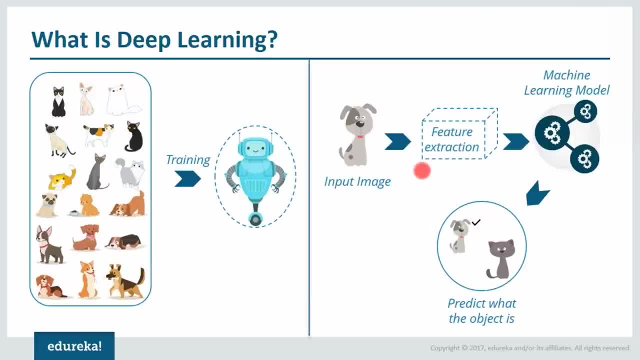 we have to manually extract features, features such as nose whiskers, All those features. We have to manually extract it and provide it to our machine learning model and trust me guys, in every scenario It is not possible If you have large number of inputs. 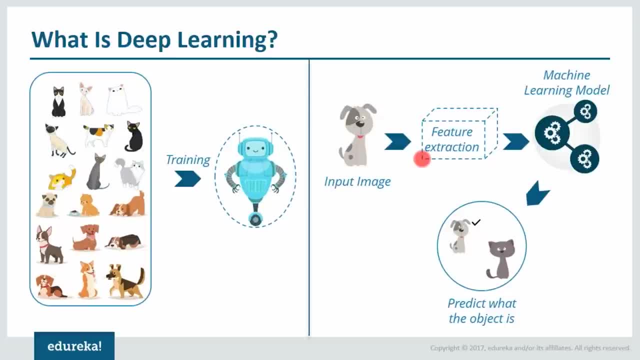 you cannot do that. You cannot manually extract the features or basically, you can say columns which are important for you in order to predict what the object is right, and that led to the evolution of deep learning. So what happens in deep learning? we skip the manual step of feature extraction. 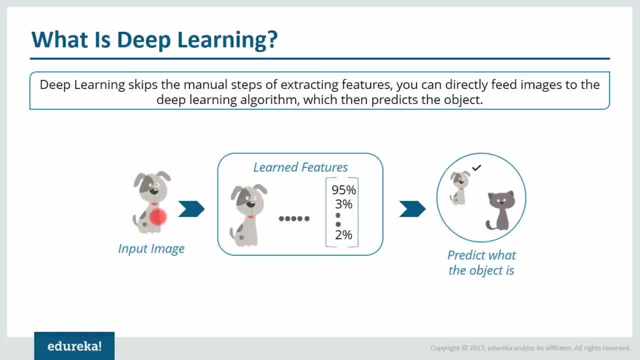 So what we do? we directly take the input image and feed it to our deep learning algorithm and because of that, what happens? whatever features are we already manually provided. apart from that, there might be many other features which are important, For example, if our features don't include the length of the neck. 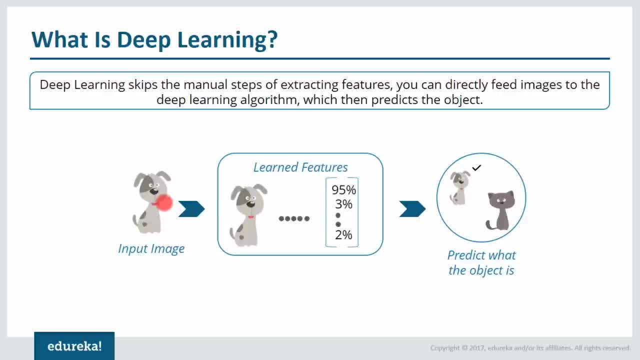 and that is one of the major feature- in order to identify or classify whether it is a cat or a dog. now what will happen? our algorithm will automatically determine that feature and will take into consideration, and then it will classify whether the input image is a cat or a dog. 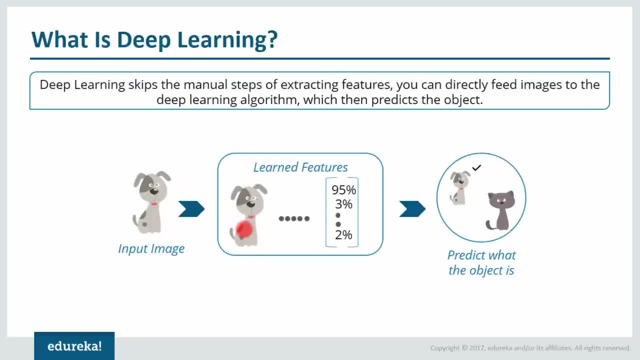 So what happens here? we provide an input image of a dog And then it will automatically learn certain features, even if we don't provide it with those features, and after that it will give us the probability and according to this particular scenario, it says: 95% chances of being a dog, 3% chances of some other animals. 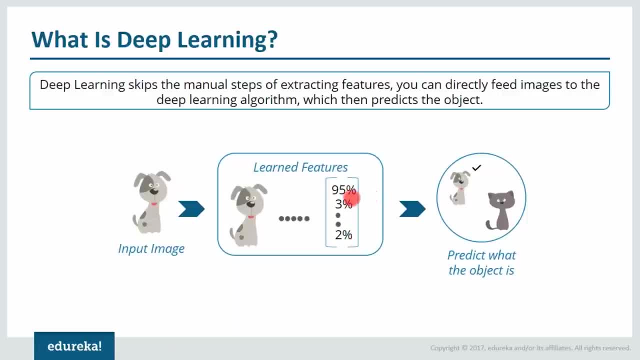 Similarly, 2% chances of some other animals. So since the highest probability goes with the dog, so the prediction says that the object or the input image is nothing but a dog. So I have a question popped in my screen. It is by Siddharth. 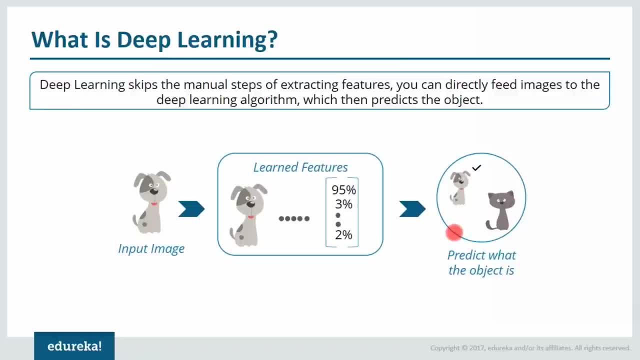 He's asking, deep learning algorithms are different than machine learning algorithms. No, so that not always. even in deep learning We have supervised and unsupervised learning algorithms. but the major difference is in deep learning We have more number of hidden layers, or you can say we have a more number of inputs. 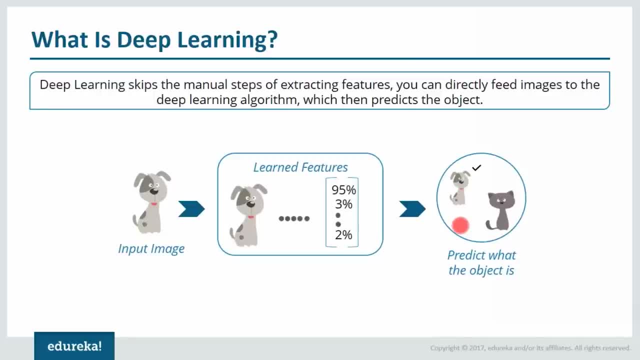 and because of those inputs, there's a very important concept that is called feature extraction, which allows the algorithm to learn certain features even if we don't explicitly provide it. So this is what the difference is: the algorithms are same, supervised, unsupervised, even in deep learning. 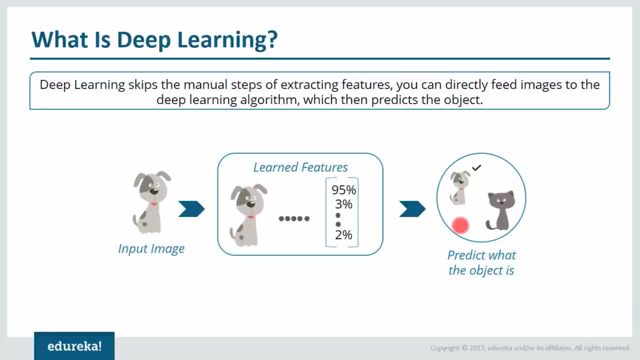 We use those kind of algorithms. I hope this answers your question. So that says yes, And we have one more question. So is it a better version of machine learning? Yes, it is definitely a better version of machine learning. Now, always there are two sides of a coin when I say it is a better version. 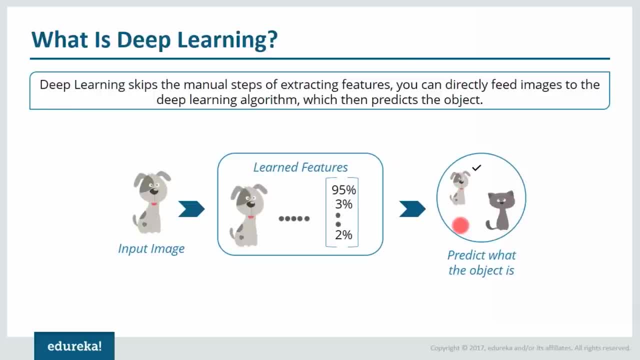 of machine learning is because if you have that much amount of computational power, then definitely deep learning is a better option And at the same time if you have large number of inputs, then also deep learning is a better option than machine learning. But if you have small, 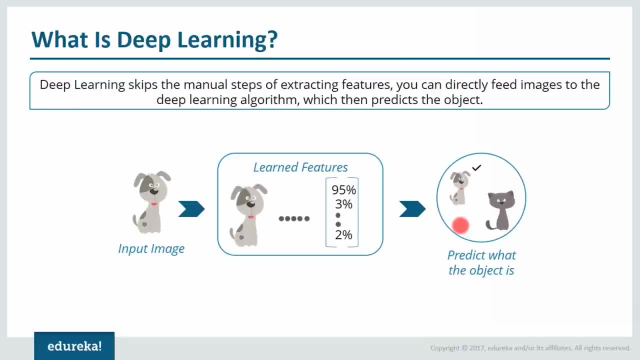 small amount of inputs and with less computational power, then definitely go with machine learning, All right. So any other questions, any other doubts, guys, you can ask me. All right, so everyone's clear. I have one more question. This is from Neha. 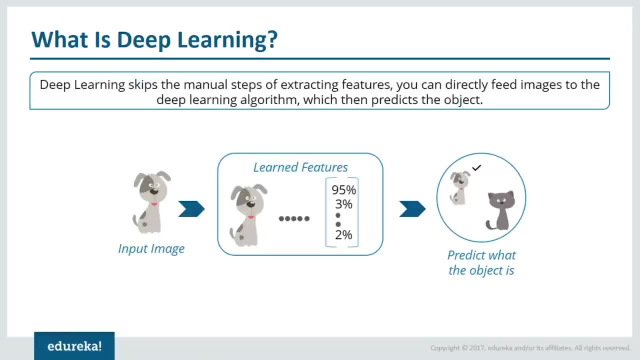 She's asking: what do you exactly mean by feature extraction? All right, Fine, Yeah, I'll explain it to you. Now we'll leave this example and I'll explain it to you with a different example. Suppose I have image of a human being itself. 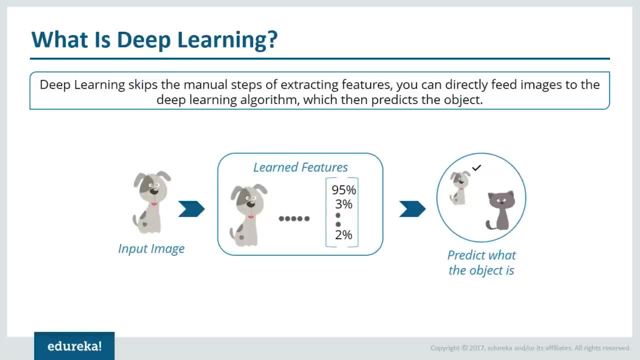 right, And I want my algorithm to predict or identify that particular image. Now, what happens in machine learning? You have to train your model with all possible features of that particular humans face, For example, edges, sharpness, colors, all those things. You have to provide all those features in order to make prediction. 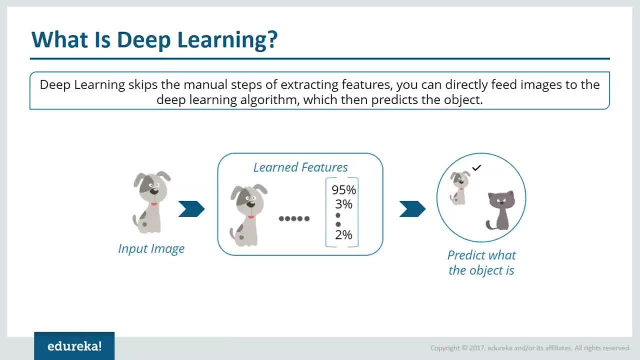 or in order to identify that particular image in machine learning. but when I talk about deep learning, the deep learning algorithm itself generates those features- for example, sharpness and things that I've discussed- And then it'll give you the output, because many times you are not able to provide all the features right. 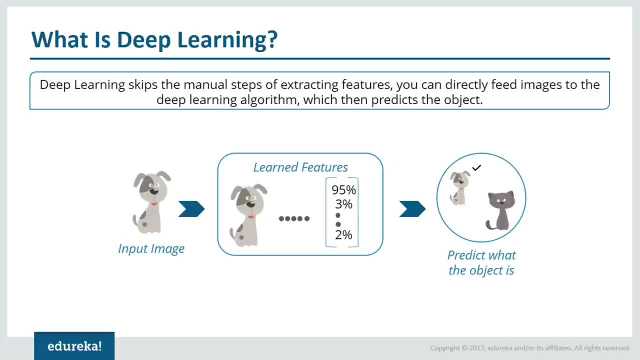 if I want a model that can predict any sort of image, that can identify any image that is there in the whole world, So I cannot provide it with all the images that are there in the whole world. I cannot train that model with all the images that are present everywhere, right? 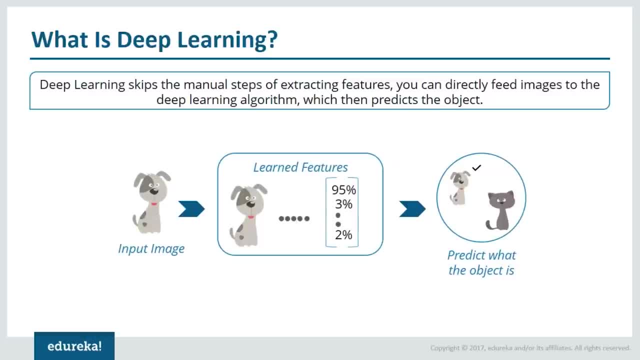 that is next to impossible. I cannot load in all the features at once, So that's when we use deep learning to learn certain features on its own, with a little bit guidance as well. This is what feature extraction is. I hope this answers your question. 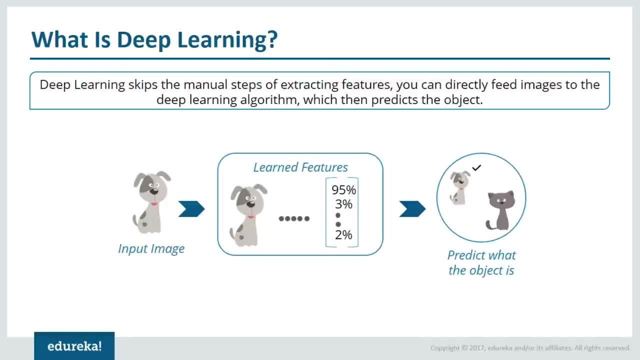 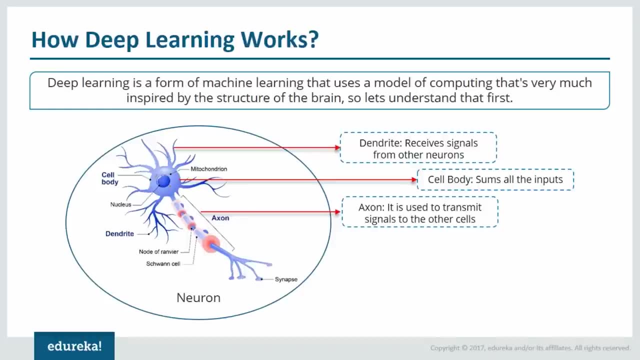 All right, She's happy with the answer. fine guys, So we'll move forward and we'll understand how exactly deep learning works. So the motivation behind deep learning is nothing but the human brain, as we have seen in the previous analogy as well What we are trying to do. 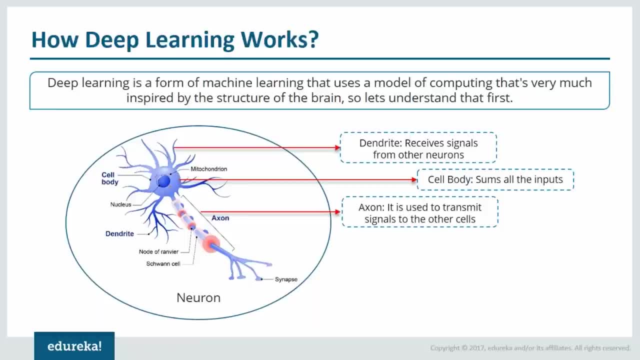 We are trying to mimic the human brain. We are trying to mimic the way we think, the way we take decisions, the way we solve problems. We are trying to make sure that we have a system that can mimic our own brain. So obviously the motivation for deep learning has to be our brain. 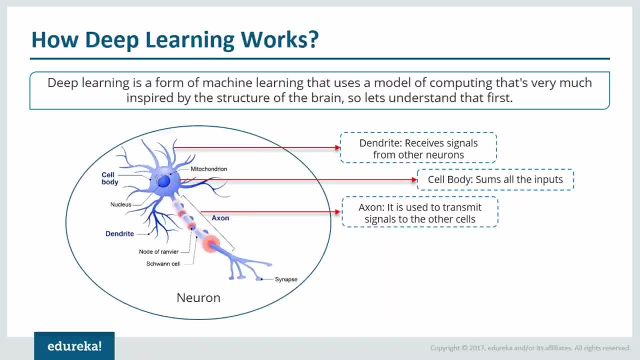 and how our brain work with the help of our brain cells, Which we call a neuron. now let us understand how a neuron works and let me tell you guys- This is what we think- how a neuron works. This is what our studies tell us. 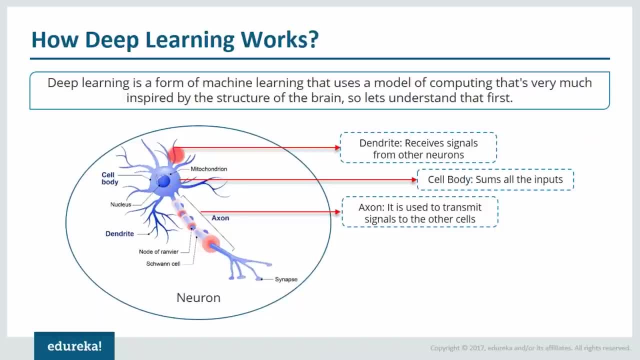 So yeah, so these are called dendrites. So dendrites receive signals from other neurons and then it passes those signals to the cell body. Now this cell body is where we perform certain function. It can be a Sigma function. That's what we believe. we believe it performs Sigma function. 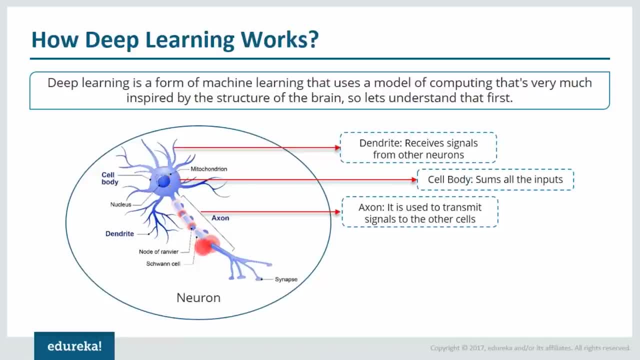 That is nothing but sums all the inputs. then, through Exxon, What happens? these signals are fired to the next neuron, And the next neuron is present at some distance, and that distance is nothing but synapse. So it fires only when the signals coming from the cell body exceeds a particular limit. 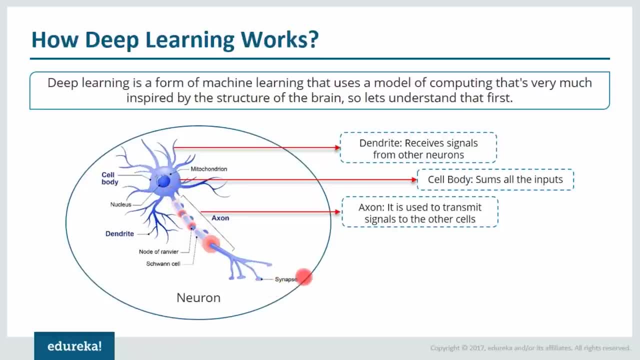 then only the cell or this neuron will fire the signals to the next neuron, and this is how the neuron at the brain cell works, and we take the same process forward and we try to create artificial neurons. So let us understand why we need artificial neurons with an example. 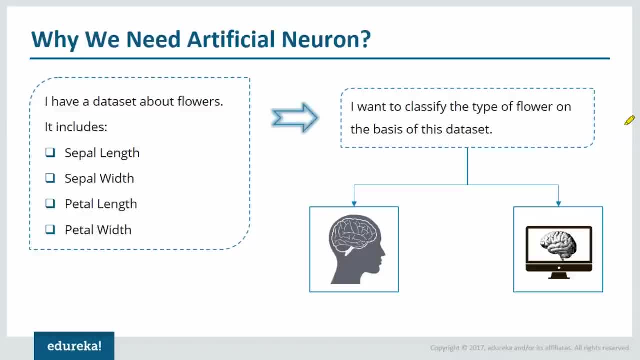 So I have a data set of flowers, say, and that data set includes sepal length, sepal width, petal length and petal width. now what I want to do, I want to classify the type of flower on the basis of this data set. Now there are two options: either I can do it manually. 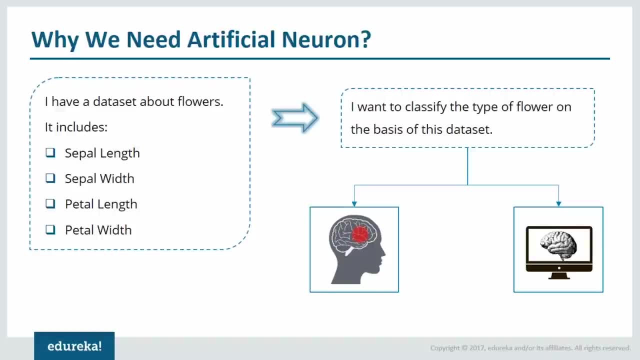 I can look at the flower manually and determine by its color or any means, and I can identify what sort of a flower it is, or I can train a machine to do that. Now let me tell you the problem with doing this process manually. First of all, there might be millions of inputs that will be given to you. 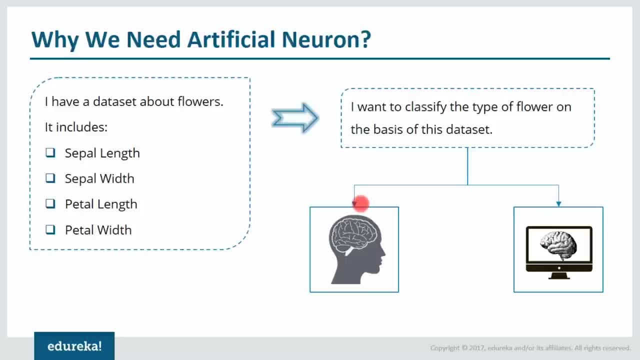 and for a human brain to perform that particular task is next to impossible. and at the same time we always get tired at some point of time, right? So we cannot just continue working for a long period of time in single stretch. and the third point is human error risk. 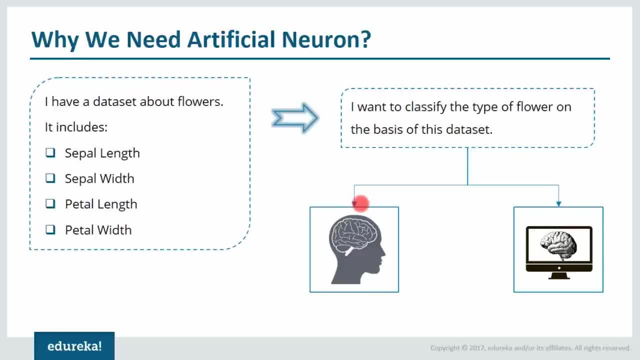 which is always there. So these are a few limitations with the human brain. So what we can do, we can train a machine to do that task for us, or we can put our brain inside a machine so that it can classify the flowers for us. 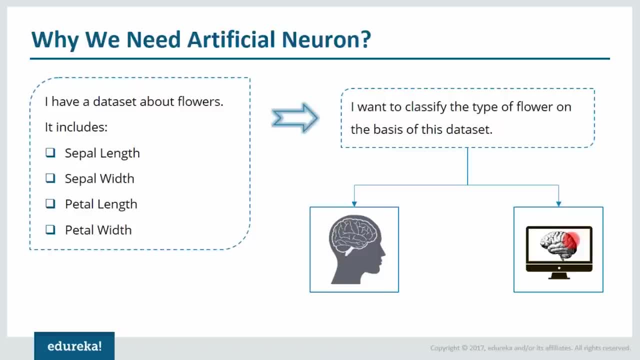 So with this, what will happen? the machine will never get tired and and will make better predictions as well. So this is why we create artificial neurons, so that there's a system present that can mimic our brain, and this is how this is what exactly happens. 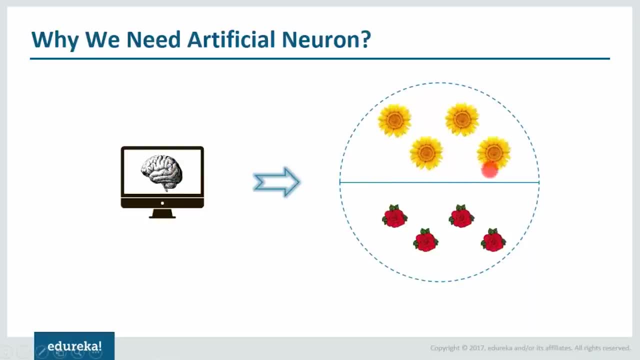 So this particular artificial neuron can actually classify the flowers, or you can say, can divide the flowers on the basis of certain features. in our case It is sepal length, sepal width, petal length and petal width. So on that basis it can classify the two flowers. 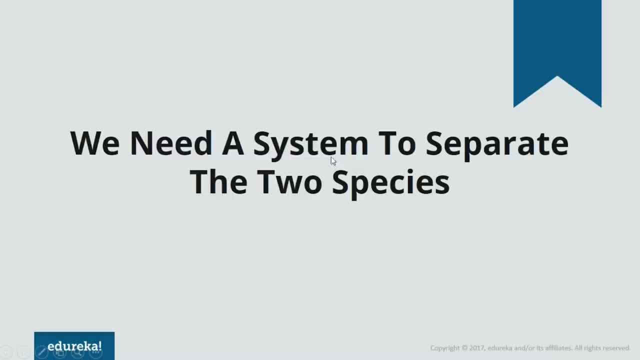 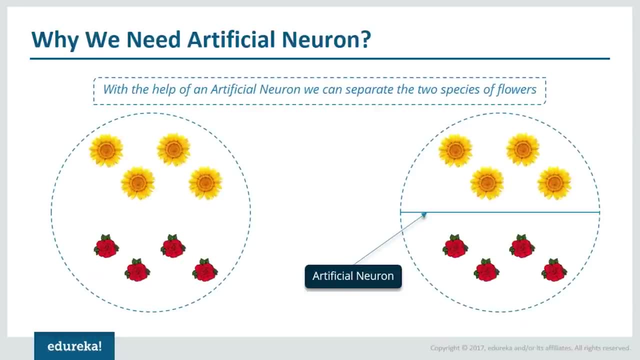 So what we need here, we need some sort of a system that can actually separate the two species. And what is that system is nothing but an artificial neuron. So we need artificial neuron, and one type of artificial neuron is a perception. Now let me explain you perception with the flow diagram. 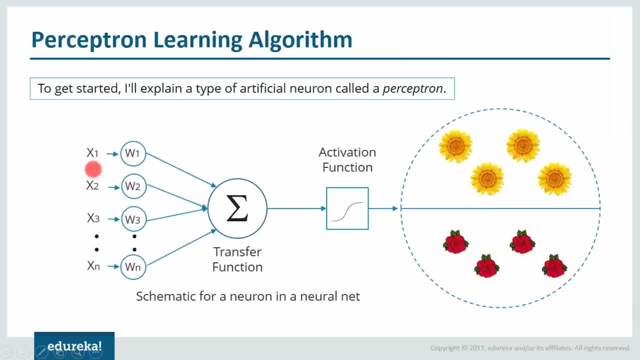 that is there in front of your screen. now, over here, What happens? we have set of inputs like X 1, X 2, dash, dash, dash till. except now, these inputs will be multiplied with their corresponding weights, which is W 1, W 2, W 3 till WN in our case. 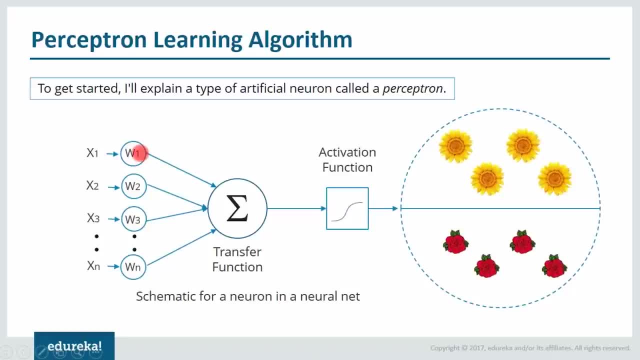 Now these weights actually define how important our input is. So the value of weight is high. We know that this particular input is very, very important for us. after multiplication, All of these are sum together and then it is fed to an activation function. Now the reason of using activation function is: 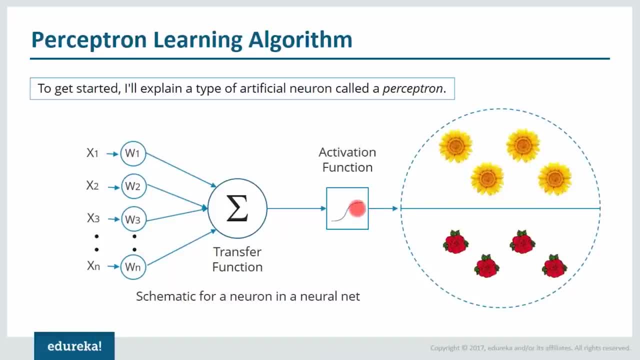 to provide a threshold value. So if our signal is above that threshold value, a neuron, or you can say our perceptron, will fire, else it won't fire. So that is the reason why we use an activation function. There can be different types of activation function. 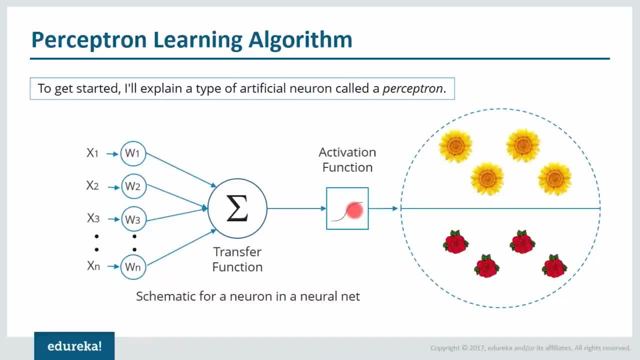 There can be sigmoid, They can be step function, sign function, depending on our use case. We define the activation Function now. the main idea was to define an algorithm in order to learn the values of the weights, which are W 1, W 2, W 3 in our case. to learn the values. 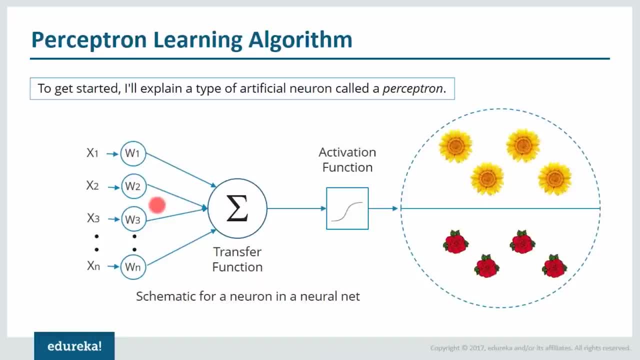 of the weights that are then multiplied with the input features in order to make a decision whether a neuron fires or not. in context of pattern classification, which is, in our case, flowers. So we are trying to classify the two species of flowers, such an algorithm could be useful to determine. 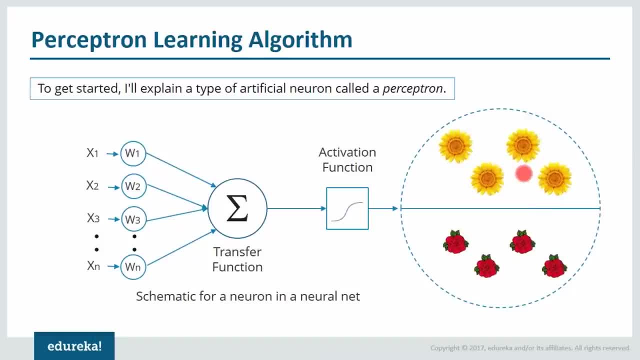 if a sample belongs to one class or one type of a species, or another class or another class, Another type of the flower. we can even call perceptron, as a single layer binary linear classifier to be more specific, because it is able to classify inputs which are linearly separable. 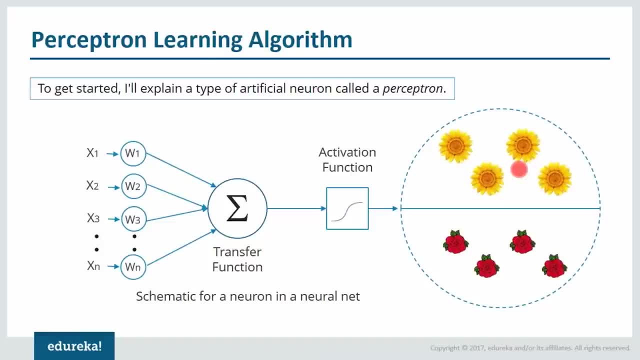 and our main task here is to predict to which of the two possible categories a certain data point belongs, based on a set of input variables. Now there's an algorithm on which it works, So let me explain you that. So the first thing we do is we initialize the weights. 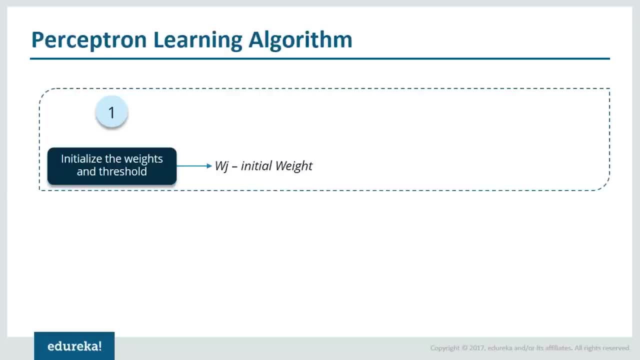 and the threshold. now, These weights can actually be a small number or a random number, and it can even be 0, so it depends on the use case that we have. then what we do: we provide the input and then we calculate the output. now, when we are training our model, 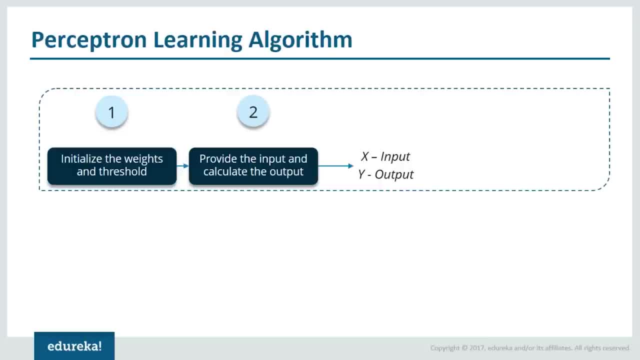 or we are training our artificial neuron. We have the output values for a particular set of inputs. So we know the output value. but what we do, we give the input and we see what will be the output of our particular neuron and accordingly we need to update the weights. 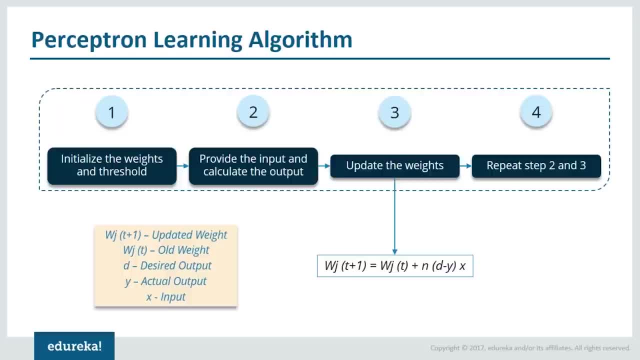 in order to reduce the loss, or you can say, in order to reduce the difference between the actual output and the desired output. So what happens? Let me tell you that. so we need to update the weight. So how we are going to update the weights is we can say: 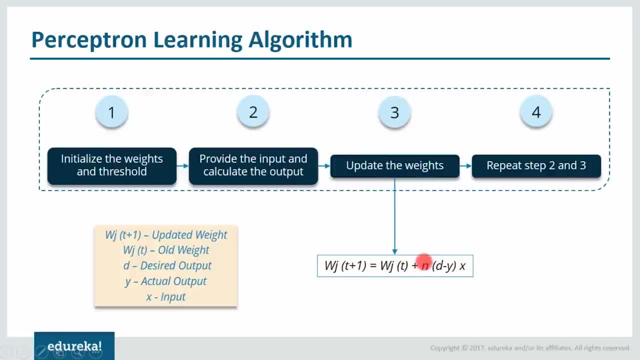 the new weight is equal to the old weight plus the learning rate. learning rate will discuss about it later in the session, but generally we choose learning rate somewhere between 0.5 to 0.01. after that, what happens? we find the difference between the desired output and the actual output. 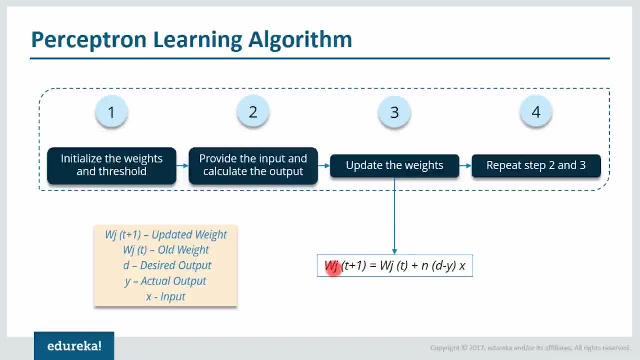 and then we multiply it with the input. So on that basis we get a new weight. So this is how we update the weights and then what happens? we repeat the steps 2 and 3.. So we are going to repeat the steps 2 and 3. that is, we are going. 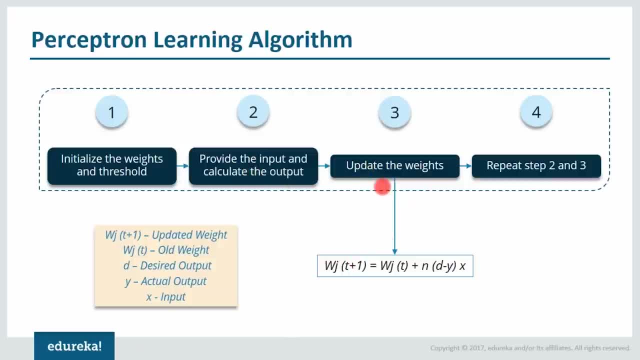 to apply this new weight again. We are going to calculate the output again, We are going to compare it with the desired output and if it matches, then it's fine. Otherwise we are going to update it again. So this is how the whole perceptron learning algorithm works. 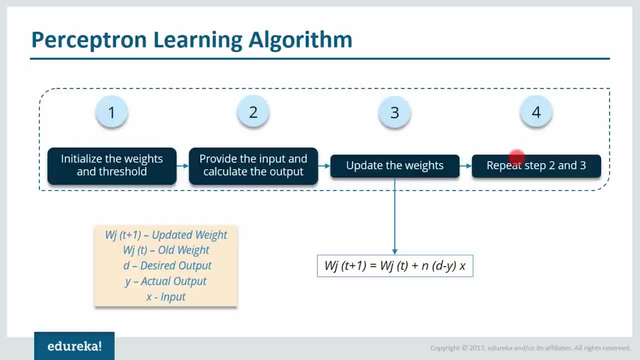 and don't worry guys, I'm going to show it to you practically how it actually works in my pie chart. any questions, any doubts till here, you can ask me. So we have a question from Emma. She's asking how the artificial neuron is similar. 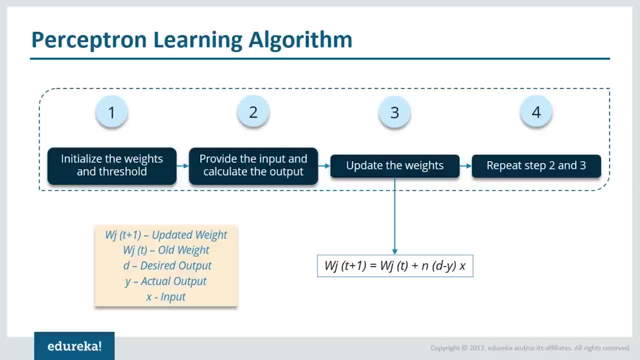 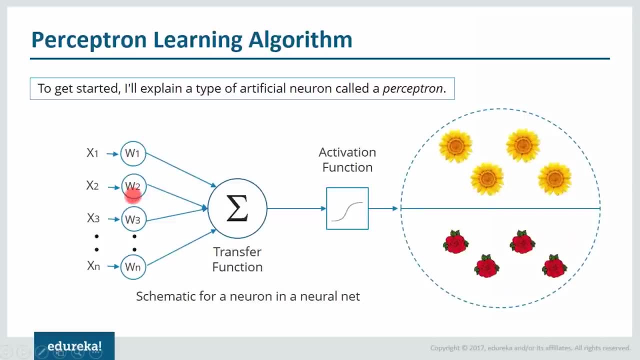 to the neuron that we have in our brain. All right, So that's a very interesting question. So let me go back to the perceptron structure that we have. So yeah, so over here, what happens? you can consider these points, as your dendrites say, similar to your neuron, the brain cells. 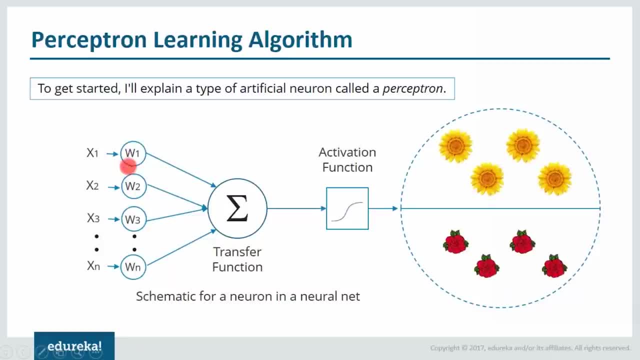 what we have? we have multiple dendrites through which we receive multiple inputs, so you can consider these as dendrites, and through dendrites it reaches to a cell body. So this transfer function can be considered as a cell body. So in this cell body what happens? some function is performed. 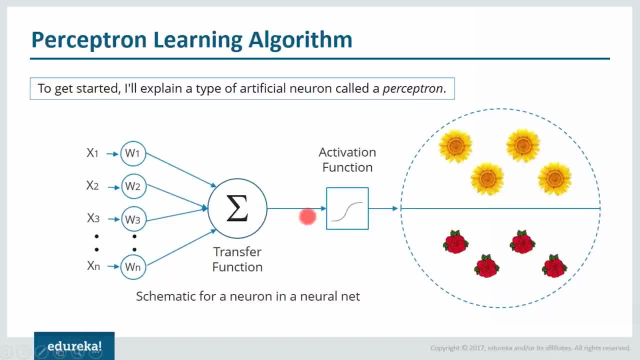 in our case It is a Sigma function. then what happens? it travels through the exon. if it reaches to a particular value or it exceeds that particular value or the threshold value, then only our artificial neuron will fire, or you can say our perceptron will fire. 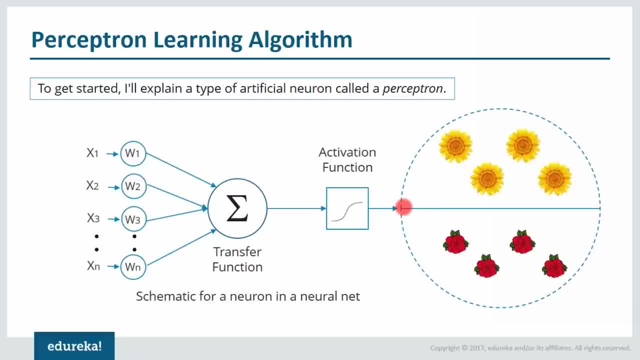 So this is how we can actually relate it with the neuron or the brain cell that we have, and obviously we don't use any of these terms. So yeah, this is how we are trying to relate it with the actual neuron. So I hope this answers your question, Emma. 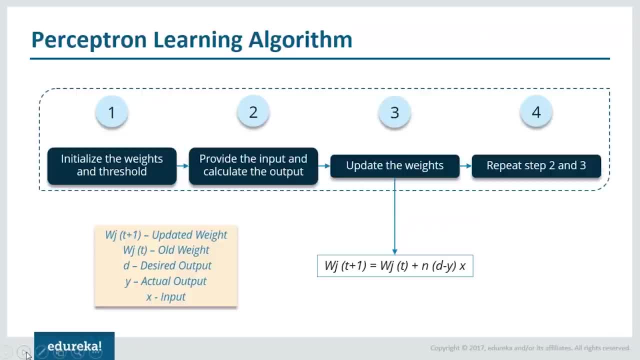 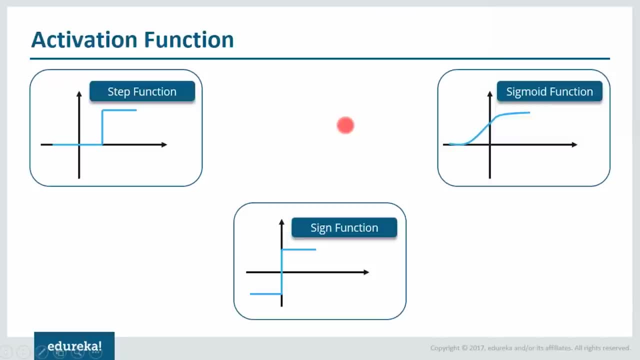 All right, Happy with the answer? fine guys. So we'll move forward and we'll see the various types of activation functions. So these are the various types of activation functions that we use, although there can be many more activation functions. again, I'm telling, it depends on your use case. 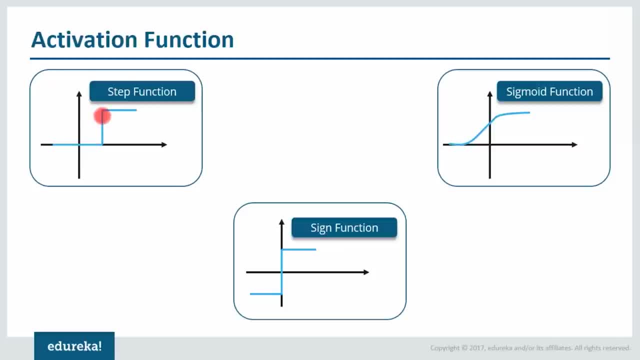 So we have a step function. So if our output is actually above this particular value, then only a neuron will fire, or you can say the output will be plus one, or if it's less than this particular value, then we'll have no output, or we'll say zero output. similarly for the sigmoid function. 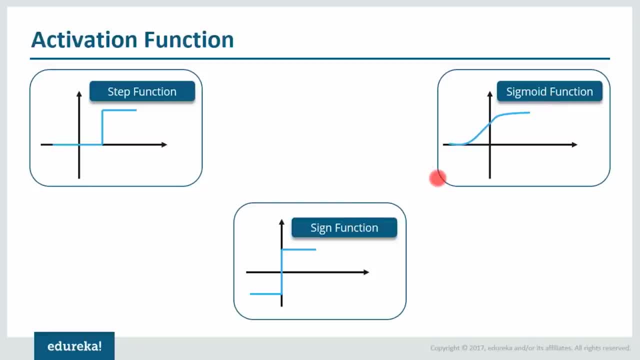 as well, and same goes for sine function. So I have a very interesting question from Emilia. She's asking why we choose only these sort of activation functions. All right, That's a very good question. Now Let me tell you what happens. 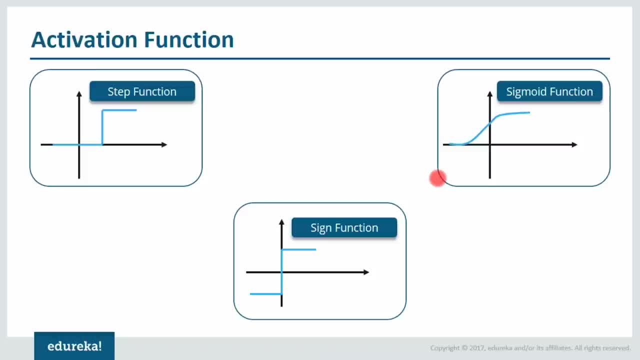 We are actually, since we are trying to mimic our brain, and our studies tell us that the same activation function is actually used in our brain as well, especially the sigmoid function. So our studies, or the doctors who have done the studies, they tell that the sigmoid function is what is there present? 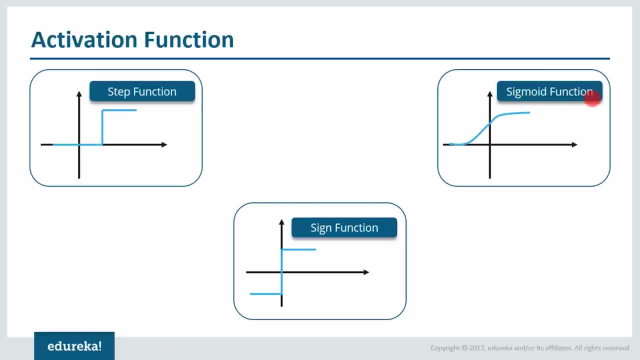 in our neuron, in our brain. So we try to mimic that same thing and at the same time. the reason for choosing sigmoid function is that it is easily differentiable, and if you differentiate it twice you'll get back the same sigmoid function. I hope this answers your question, Emilia. 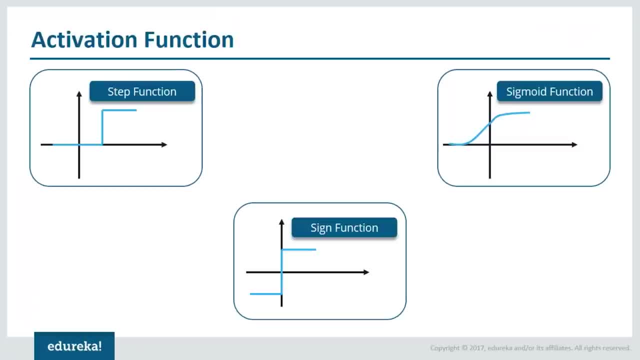 All right, she's happy with the answer. fine, Any other questions? any other doubts, guys, you can write it down in a chat box and I'll be happy to help you. any questions? All right? fine, There are no questions. So let us move forward and we'll focus on various applications. 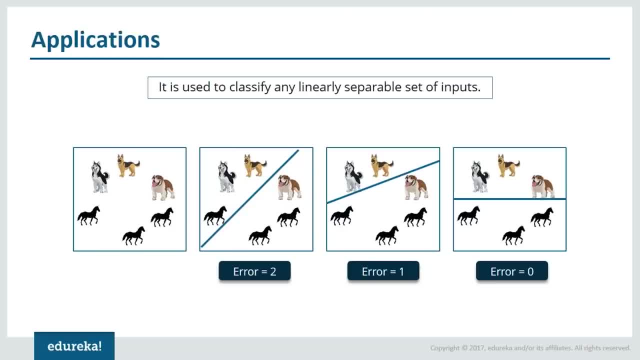 of this perceptron. Now, as I've told you earlier as well, it can be used to classify any linearly separable set Of inputs. now let me explain to you with the diagram that is there in front of your screen. So we have different types of dogs and we have horses. 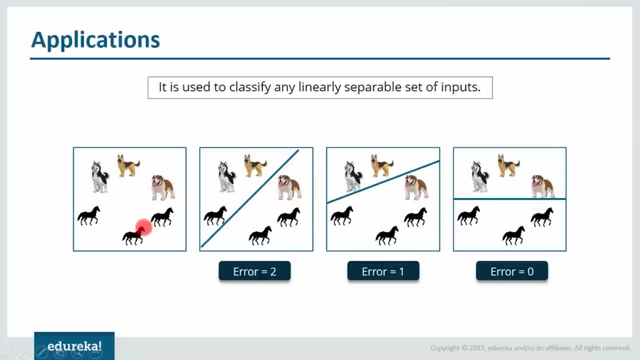 and we want a line that can separate these two. So our first iteration will produce this sort of a line. but here we can notice that we have error here, as we have classified horse one of the horses as a dog and a dog as a horse. 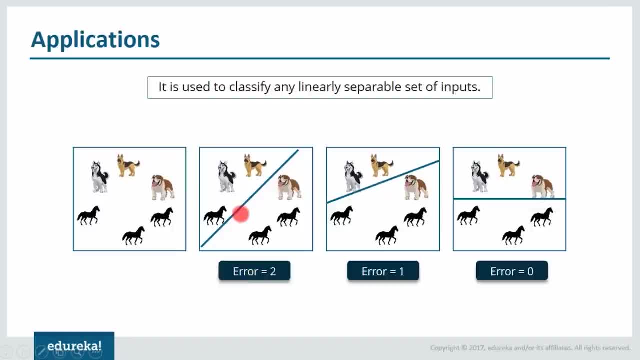 So error is two here. Similarly, we now what happens? we have updated the weight. now, after updating the weight, what happens? our error has reduced. So what happens now? We have Actually classified all the horses correctly, but one dog we have classified wrong and we have considered it as a horse. 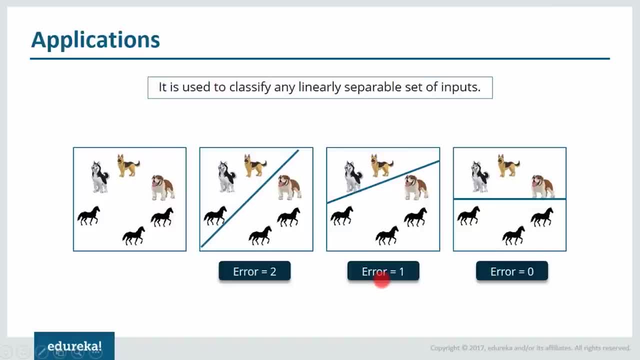 So our error becomes one once again. what will happen? if you can remember, the step two and three of a perceptron learning algorithm will be done, and then, after that, our weights will be updated and our desired output will become equal to our actual output, and we get a line something like this: 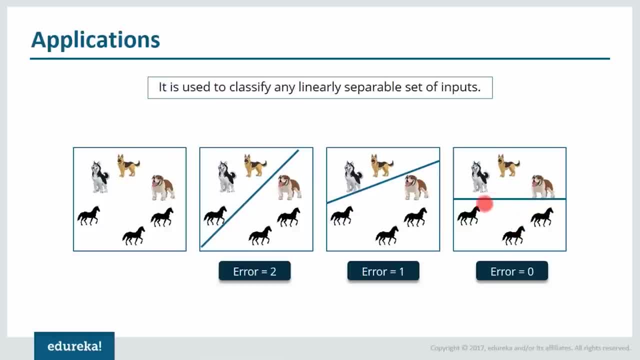 So what we have now? we have properly classified dogs and horses, So this line separates both of them. This is how we can actually use a single-year perceptron In order to classify any linearly separable set of inputs. Now we can even use it in order to implement a logic gates. 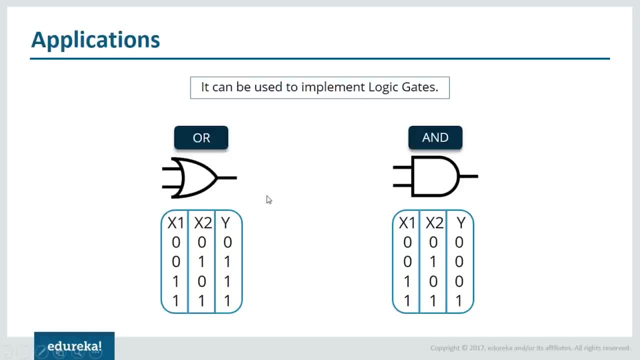 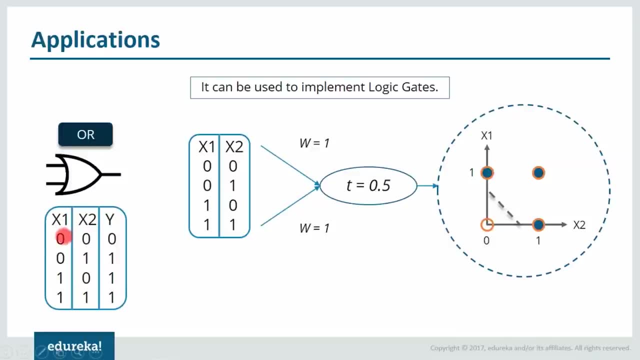 that is, or, and, and. now let me tell you how you can do that. First, We'll look at our gate. now, in our gate, What happens here is the truth table. truth table. According to that, we have two inputs, x1 and x2.. 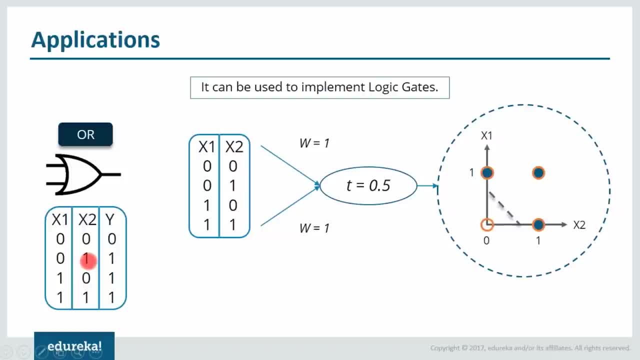 So if both are 0, we get a 0. if any one of the input is high, or any one of the input is one, we get the output as one. So what we need to do is we need to make sure that our weights are present in such a way. 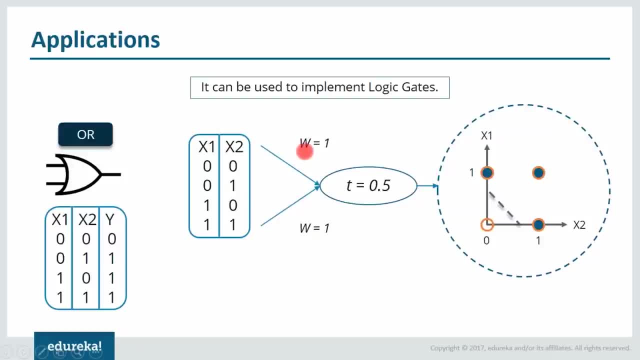 that we get the same output. So how we have done that, when the value of weight is equal to 1, and then we provide the input x1 and x2, after passing through this activation function, We get this sort of a graph, which is the graph for our order: a gate. 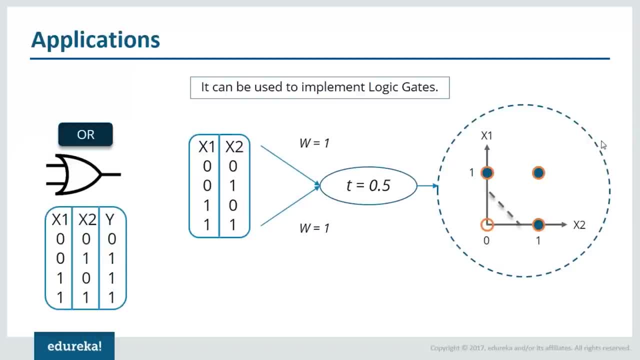 Now, if you want, I could use a pen and I can explain it to you. Now we have x1 and x2 as inputs, So we provide first input as 0, x1, and this also has 0.. So 0 into 0 is again 0, 0 into 0 is 0. 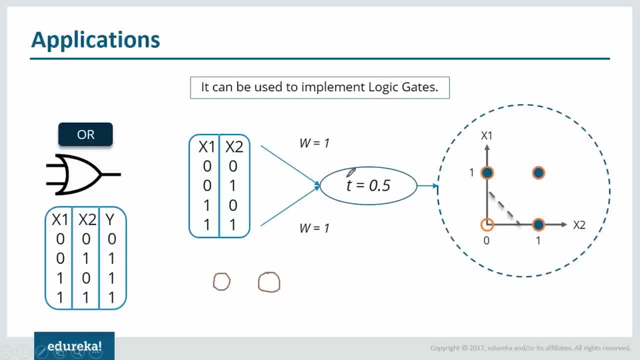 And then we passes through this activation function. Now we need to make sure that whatever value that comes here should be greater than 0.5. then only our neuron or the perception will fire, but since this value is actually less than 0.5.. 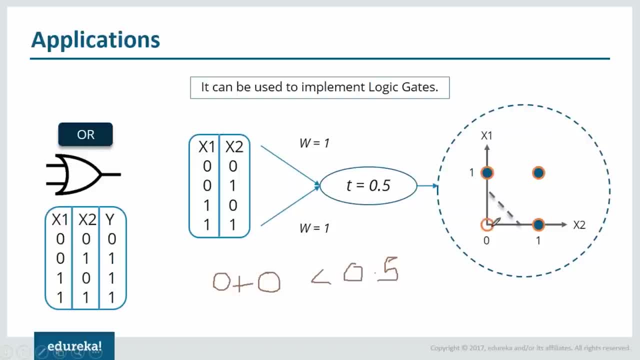 So the neuron won't fire and our output will be 0, as you can see it over here. Now let's take the other set of inputs. Now our x1 is 0 and our x2 is 1.. So 1 into 1 will what will be obviously 1.. 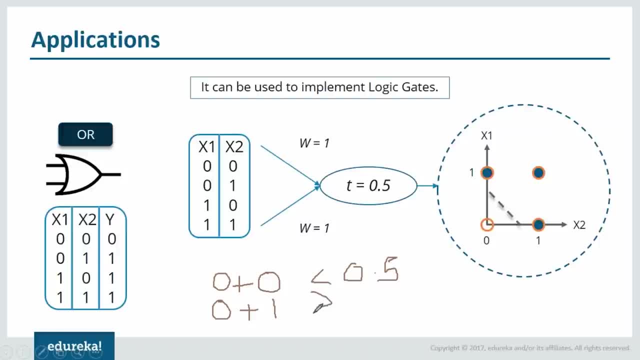 In this case, our output is bigger than 0.5.. Then what will happen? our neuron will fire and we'll get 1, the output 1 here, as you can see it in the graph. Similarly, when my x1 is 1 and x2 is 0, in that case also, our output is. 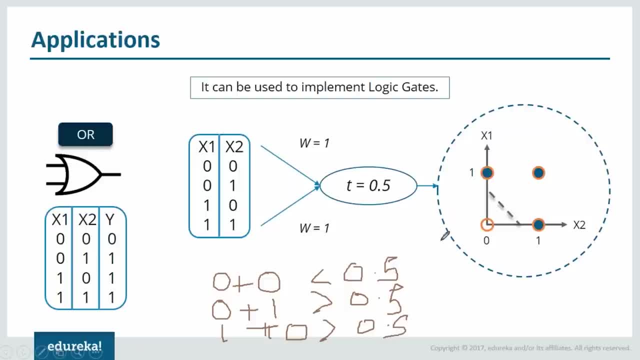 greater than 0.5 and neuron will fire and we'll get this sort of a graph. when I talk about 1- 1, then our output will be 2, which is greater than 0.5.. So we get an output that is 1, and this is how we get the graph. 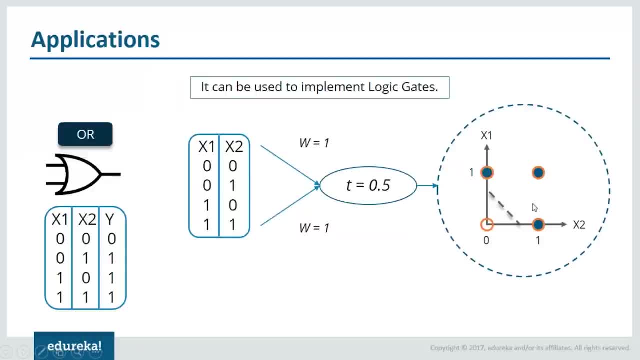 So I hope you all are clear. All right, so this is how we get this graph. and now, if you notice, with the help of the single-layer perceptron, we are able to classify the ones and zeros. So this line, anything above this line, is actually one and anything. 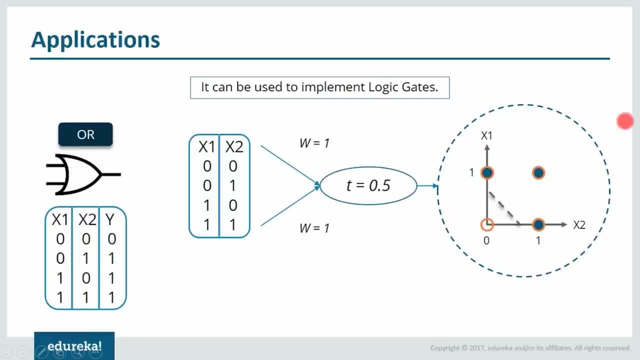 below this line, We have zeros. So this is how we are able to classify or able to implement or gate, similarly, when I talk about and gate as well. So there's a difference in the truth table of and gate in and gate what happens. we need to make sure that both of our inputs are high. 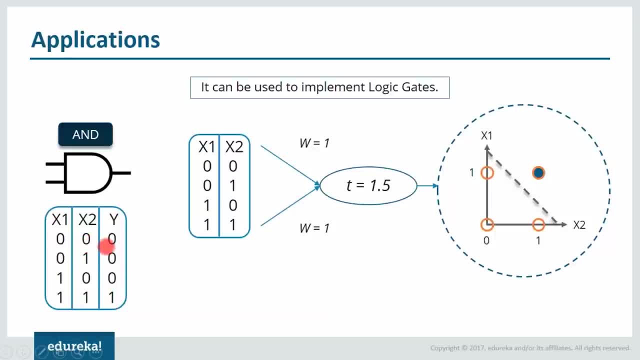 in order to get a high output. If any of the input is low, we get a low output, and that's the reason we choose an activation function that is 1.5, which means that if our value or the output is about 1.5, then only our neuron will fire and 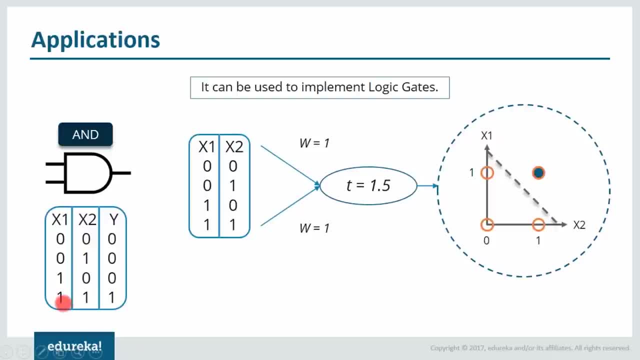 we'll get one here, and there's only one case. that is when both the inputs are high. So when both the inputs are, I let me just use my pen again and I'll explain to you. So X 1 is 1, X 2 is 1, we get something which is 2, which is obviously. 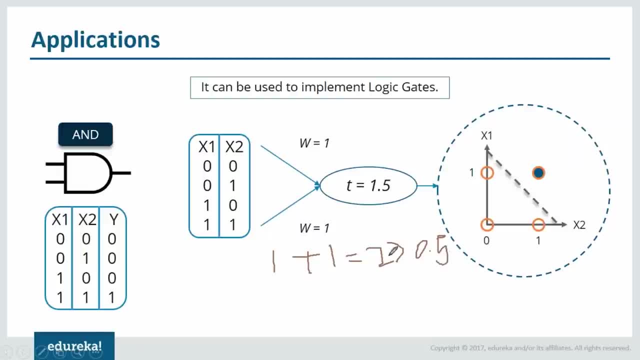 greater than 0.5.. Pardon me for my writing, But yeah, This is how it is. Yeah, so 1 plus 1, 2, which is obviously greater than 0.5.. So what we get, we are neuron fires and we get one here. but for the rest, 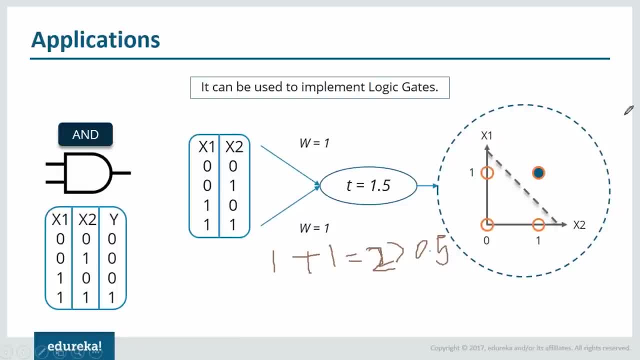 of the inputs, all will be less than 1.5.. So that is why our neuron doesn't fire and we get a 0 output. Don't worry, guys, I'll actually tell you how to implement it. I'll open my pie charm and I'll be showing it to you practically how. 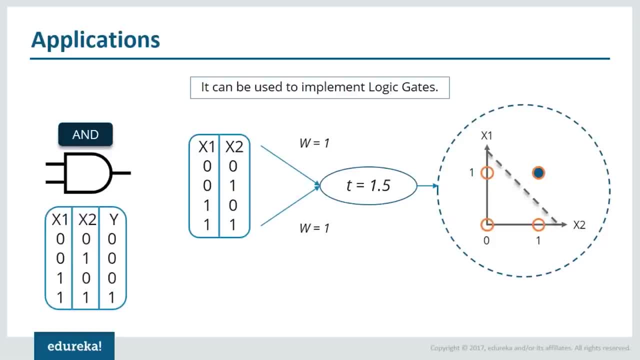 to implement these gates. So for that, what I'm going to do is I'm going to first import a python library called tensorflow. the installation guide of this particular library is present in an LMS For both Windows as well as for Linux, so you can just go through it. 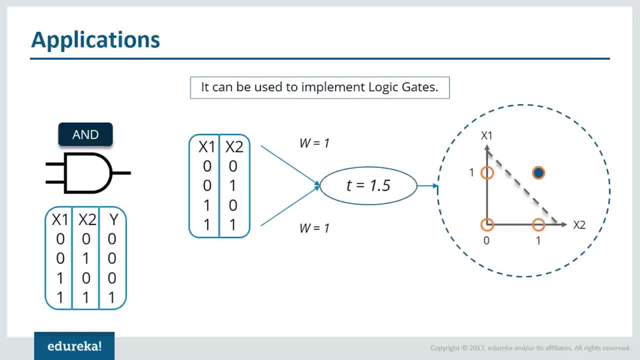 and it's very easy to install that, and I'll actually execute this practically later in the session. You don't need to worry about it. This is how we can implement and and or get. I have a question popped in my screen by Imran. 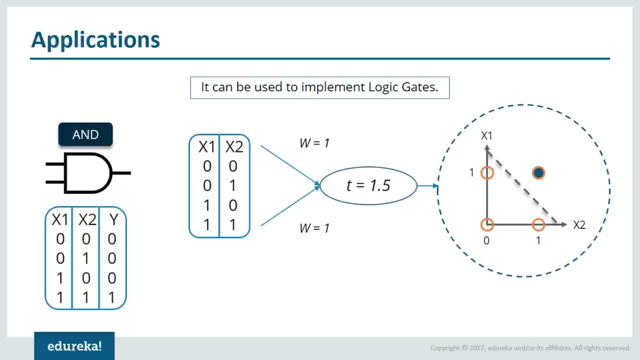 He's asking: why aren't we implementing XOR gate with the help of single-layer perceptron? All right, Imran, I'm very impressed with your question, because we cannot implement an XOR gate with a single neuron. will actually discuss that later in the session. 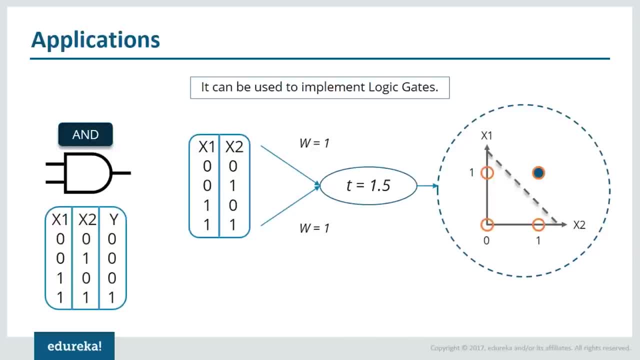 I'll tell you why we cannot do it: because it is not linearly separable. and why it is not linearly separable will also see that that's a very good question, Imran, but just be patient and it'll be covered in us today's session. 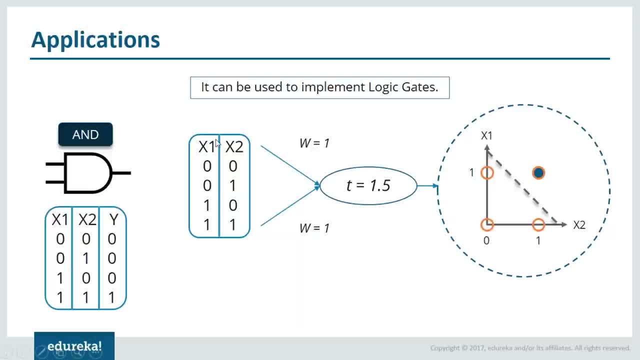 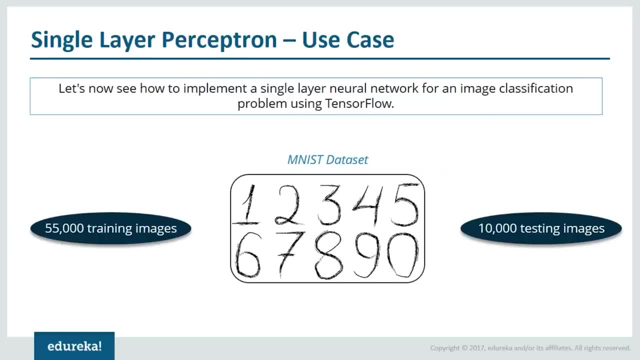 Any other questions, any other doubts, guys? So let's move forward, guys, and we'll actually understand a use case, that is, of MNIST data set. the reason for using MNIST data set is because it is already clean and will be a perfect example for this. 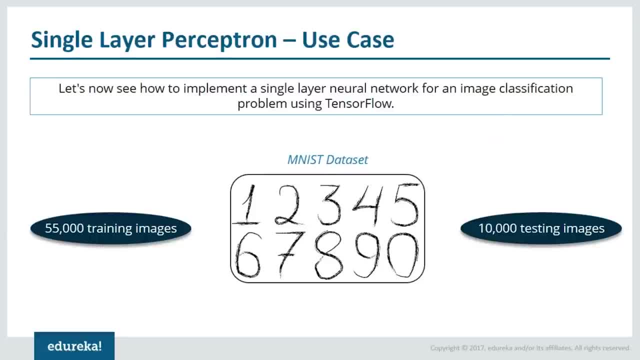 Now what this MNIST data set contains. it basically contains hand written digits from 0 to 9, and in that data set We have 50,000 training images along with 10,000 testing images. So we will train our model with those 55,000 training images. 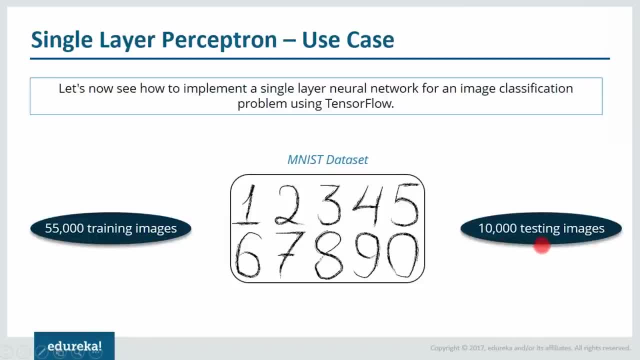 and then we are going to test the accuracy of a model with the help of those are 10,000 testing images, and for all of this we need to understand first What exactly is tensorflow. So let us move forward, guys, and will understand tensorflow, and then we are going to implement all these things that we have discussed. 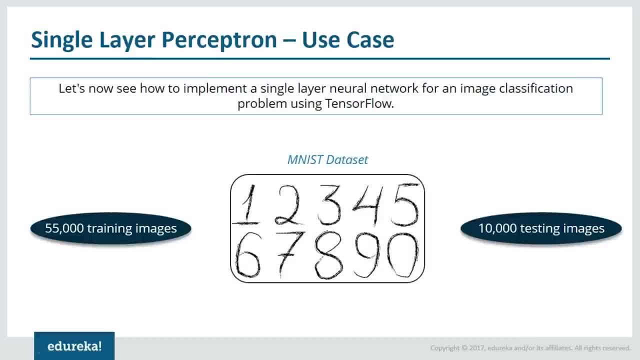 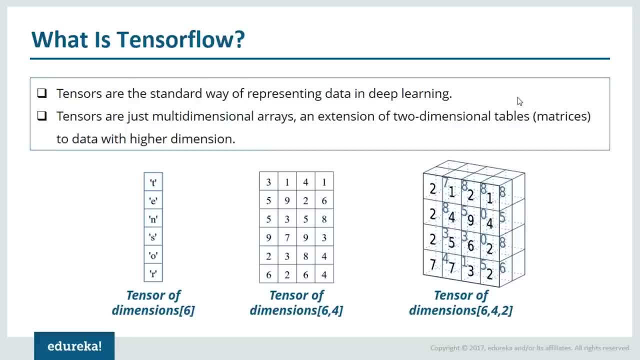 that is, and gate or gate, And the MNIST data set that I'm talking about. So let's move forward, guys, and understand what exactly is tensorflow. Now, what is tensorflow? as I've told you earlier as well, We use this tensorflow library in order to implement deep learning models. 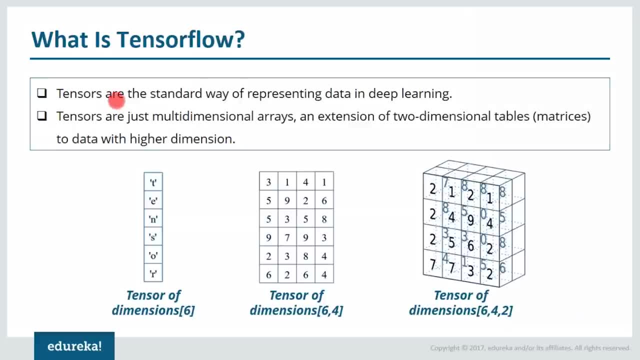 and the way the data is represented in the deep learning model is called a tensors. Now, what are tensors? now, tensors are just the multi-dimensional arrays, or you can say an extension of two-dimensional tables, matrices, to data with higher dimension. Now let me explain to you with the example. 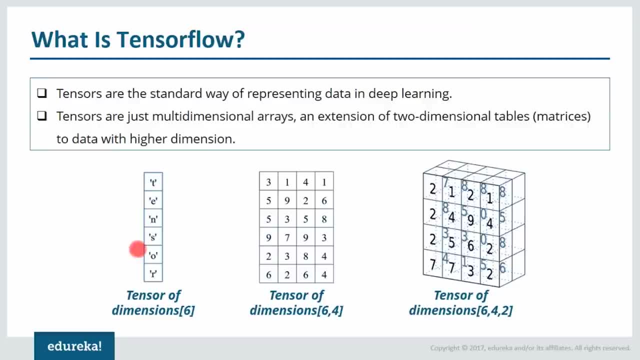 Is that are there in front of your screen. So this particular data is nothing but a tensor of dimension 6, because we have six rows and we have only one single column. now, over here, We have four columns as well as six rows, So this becomes a tensor of dimension 6, comma 4, similarly over here as well. 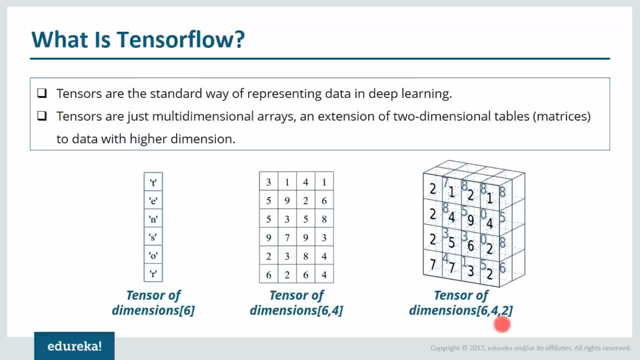 So we have another dimension, that is, the third dimension, in which we have two values. So we consider this as a tensor of dimension 6, 4 and 2.. So this is nothing but a way of representing data in tensorflow. Now, if you consider the tensorflow, 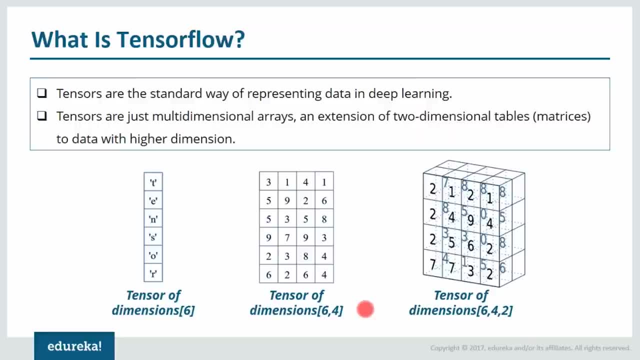 library at its core, it is nothing but a library that performs Matrix manipulation. That is what tensorflow is. Now let us move forward and understand tensorflow in a bit detail. So, as the name tells that, it consists of two words, tensor as well as flow. 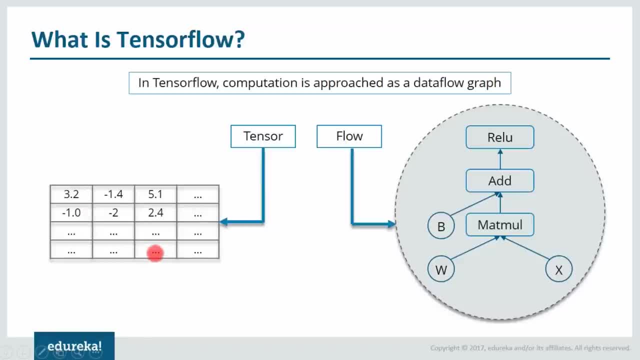 Now we understood what exactly tensor is. We saw it in the previous slide as well. Now, when I talk about flow, it is nothing but a data flow graph, So let me just give you an example. that is there in front of your screen. 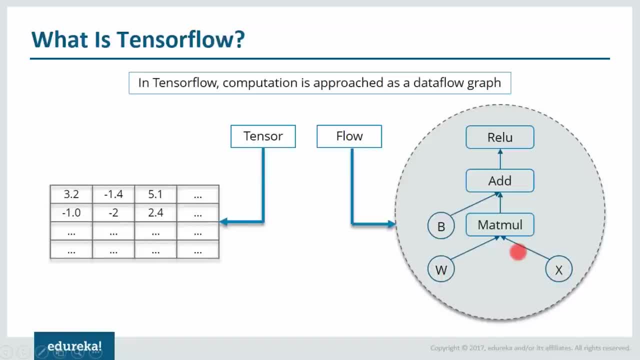 So we talked about weights and inputs. So we provide these weights And inputs and we perform a Matrix multiplication. So the weight is one tensor, X input is one tensor. Then we perform Matrix multiplication. after that We add a bias which will actually see it later in the session. 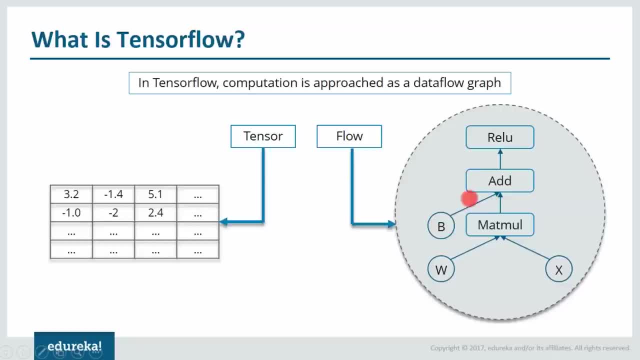 You don't need to worry about this term. Then what we do? we add all of these. So what is this? This is nothing but the Sigma function in this perceptron that we have seen. Then we pass it through an activation function and the name of that activation function is RELU, or RELU, what you can say it. 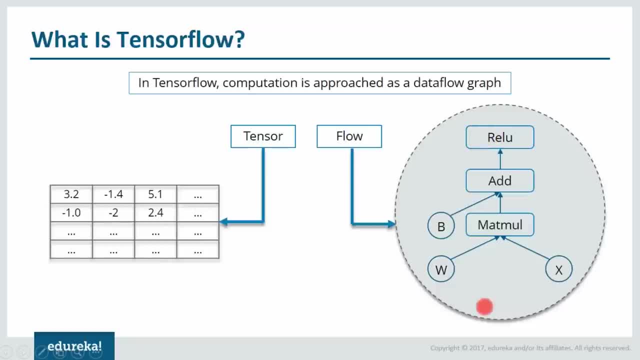 and then our neuron will fire. So this is nothing but a flow, or you can say a data flow graph. Now let us understand few code basics of tensor flow. And before that, if you have any questions, any doubts, you can write it down your chart box and I'll be happy to help you. 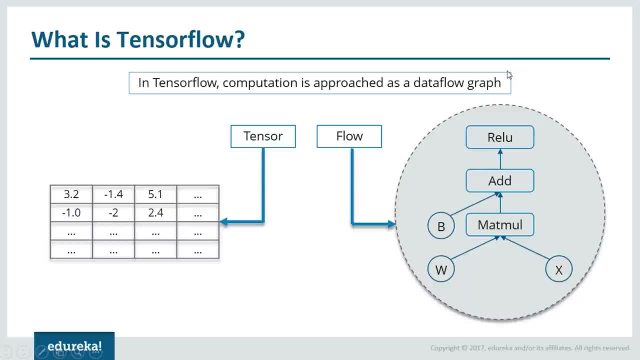 We have a question from Jack. He's asking: a tensor flow is a library for python only. Well, Jack, tensor flow is available in R as well, but we are going to use Python in our course, All right, so he's happy with answer. fine, guys. 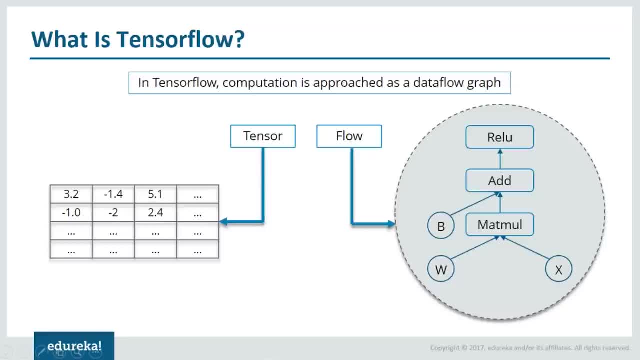 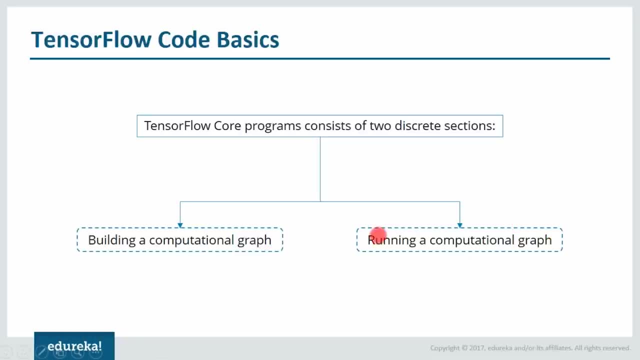 So there are no more questions. We'll move forward and understand the code basics of tensor flow. Now the tensor flow program Actually consists of two parts. one is building a computational graph and another is running a computational graph. So we'll first understand how to build a computational graph. 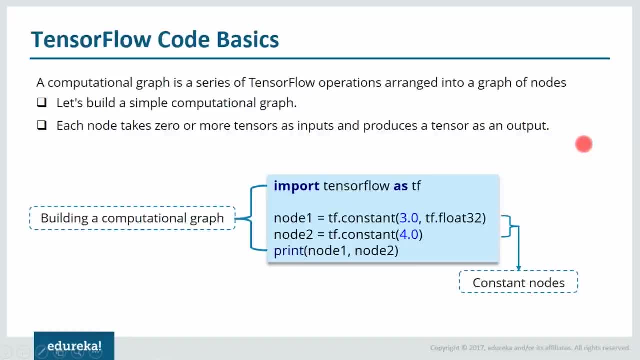 Now you can think of a computational graph as a network of nodes and with each node known as an operation and running some function. that can be as simple as addition or subtraction, or it can be as complex as, say, some multivariate equation. Now let me explain it to you with the code that is there in front of your screen. 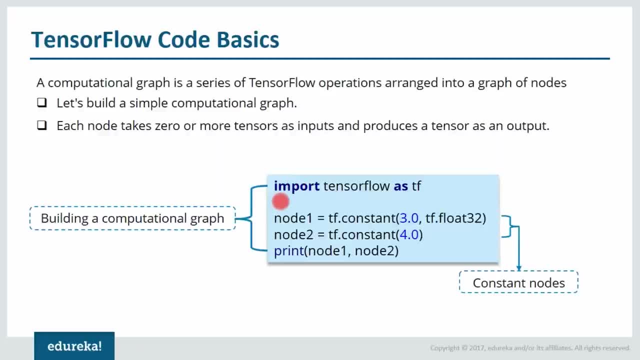 So the first thing you do, you import the tensor flow library. Then what do you do? You define two nodes and these nodes are constants. So we'll call that function, will call it as TF dot constant and will provide a value that is three. 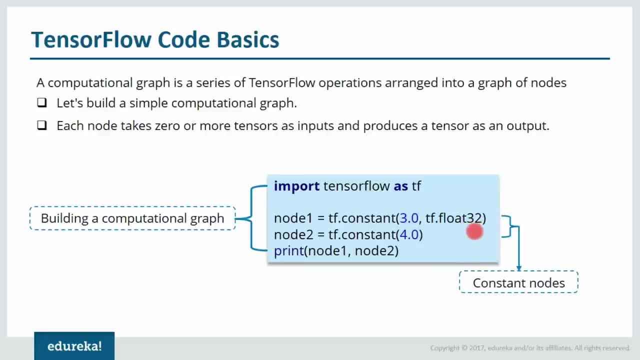 and it is nothing but a float number of 32 bits. Similarly, we defined one more node, which is a constant, and it contains value for. so these are nothing but your constant nodes. This is basically what computational graph is. So, basically, we have built a computational graph. 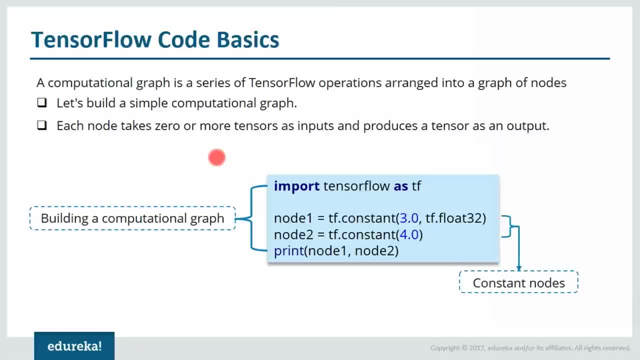 and in this graph, each node takes zero or more tensors as inputs and produces a tensor as an output. and one type of node is a constant that I've told you earlier as well, and these tensor flow constants. it takes no inputs and it outputs a value which is stored internally. 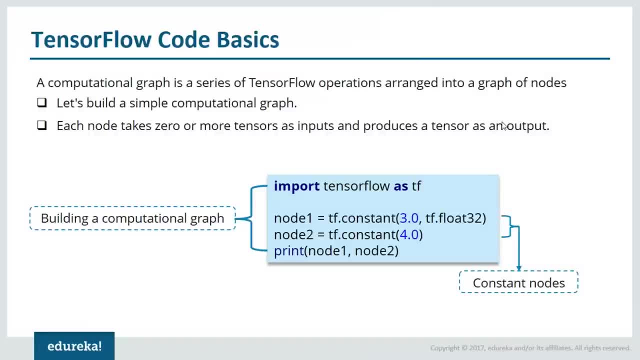 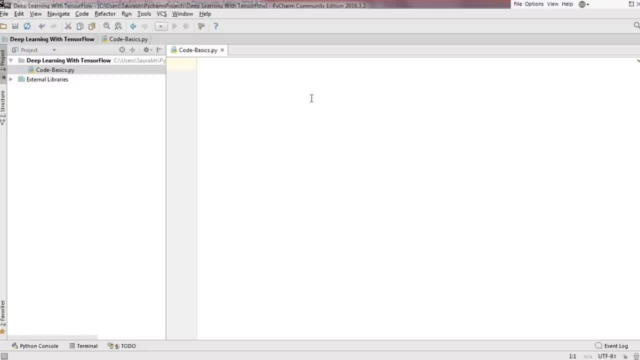 Now what I'll do. I'll actually execute this in my pie charm, So for that I'll open it. So this is my pie charm, guys, and I've already installed tensor flow, and I'm telling it to you again that the installation guide for your tensor flow in Windows, as well as Linux, is present in your LMS. 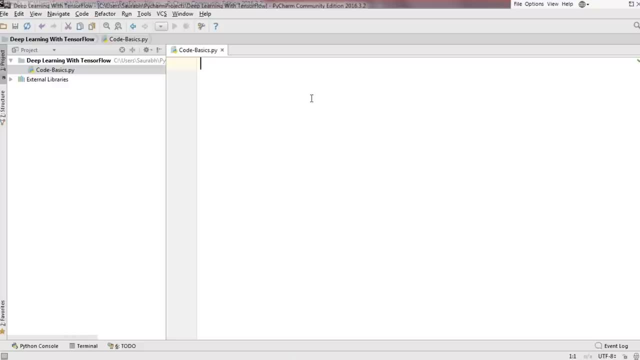 Just go through it and it's pretty easy. If you have still any doubts, you can contact our 24-7 support team. So the first thing that I need to do is import the tensor flow library. for that I'm going to type in here: import. 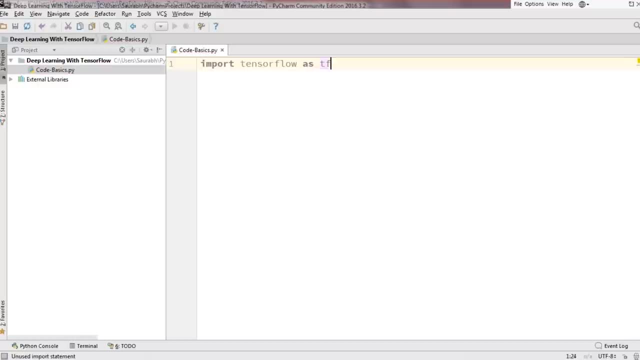 TensorFlow as TF. So if you are familiar with the python basics, you know what it means actually. So I am importing tensor flow library and in order to call that, I'm going to use the word TF. So after that, I'm going to define my node 1 and node 2, which are constant nodes. 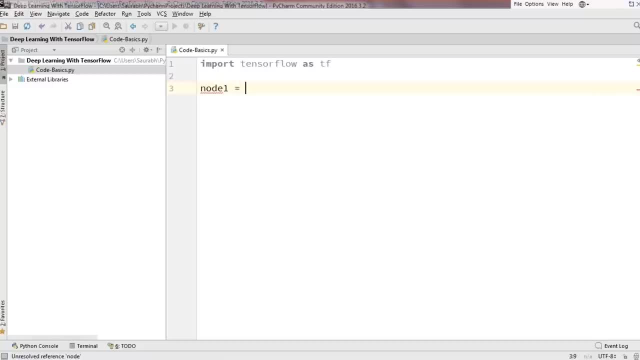 So for that I'm going to type in here Node 1, equal to TF dot constant, And then I'm going to define the constant value in this. So it will be 3 and it will be a float value of TF dot float of 32-bit. 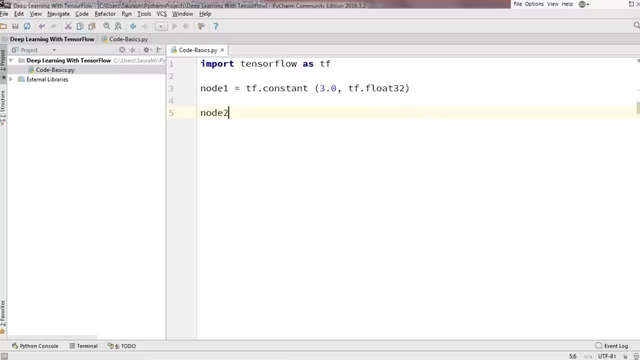 All right, and now I'm going to find my second constant node, So I'll type in here node 2: TF dot constant. I'll put 4 in here and 4, that's it. And so the TF dot float 32 will be present implicitly. 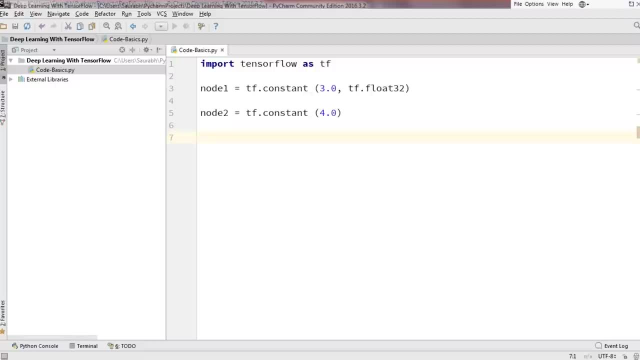 I don't need to do that again and again. So I have created a computational graph here. So what if I print it now? So let us see what will be the output. node 1: comma. node 2.. Let's go ahead and run this and see what happens. 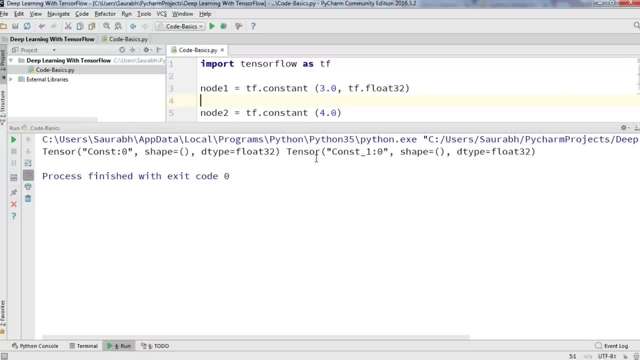 If you notice here that printing the nodes does not output the values 3 and 4, you might be expecting that right, that it should print 3 and 4.. For instance, they are nodes that, when evaluated, would produce 3 and 4 respectively. 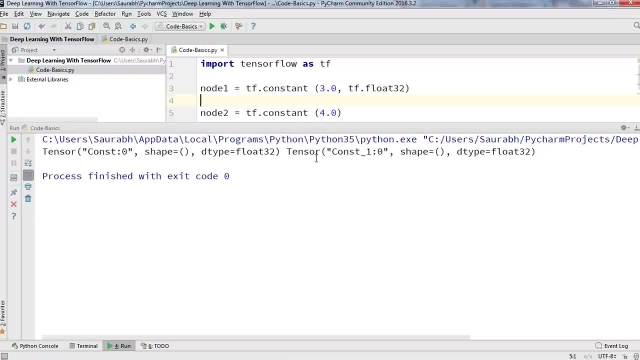 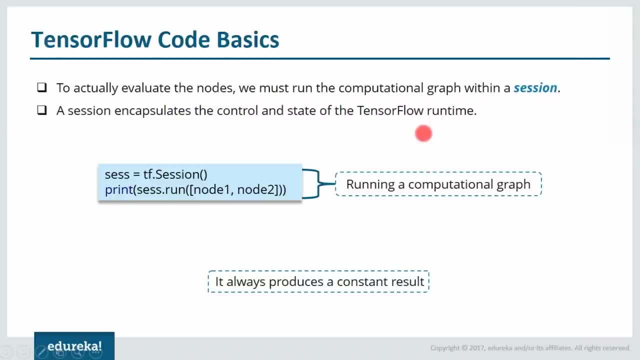 So, to actually evaluate the nodes, what we need to do is we need to run this computational graph. So let me show you that. for that I'm again going to open the slides. So, since I've told you earlier as well, we need to actually run this computational graph within a session. 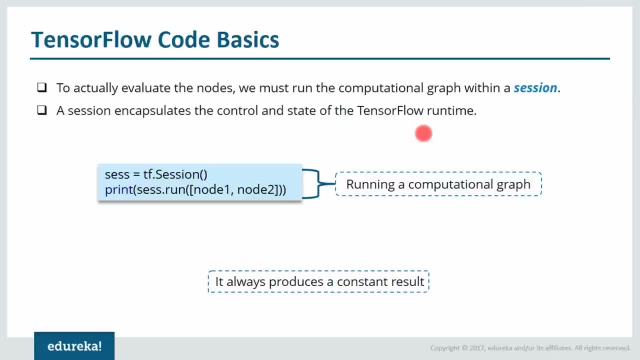 And what is this session? It's session actually encapsulates the control and state of the tensorflow runtime. Now the code that is there in front of your screen. what it will do: it will actually create A session object and then it invokes its run method to run enough of the computational graph. 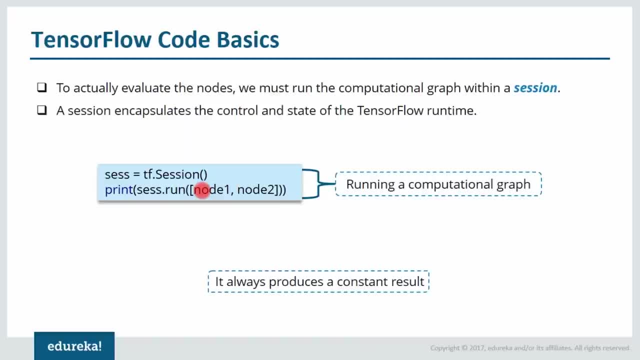 in order to evaluate node 1 and node 2, and how it does that by running the computational graph in a session. So now let me show it to you practically how it happens. So again, I'm going to open my pie charm. This is my pie charm, guys. 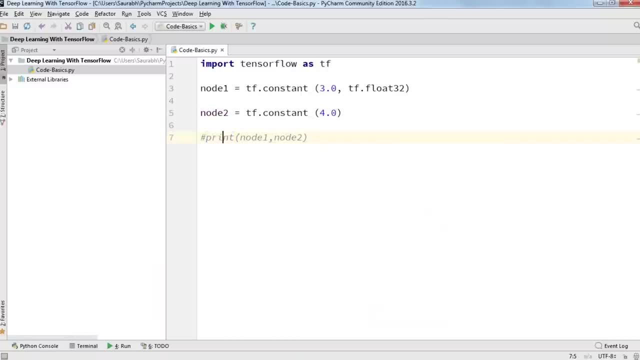 So let me first comment this print statement- and now I'm going to run a session, So for that I'm going to type in here: says equal to TF dot Session. and now I'm going to print it, So for that I'm going to type in print: says dot run and what I want to run. 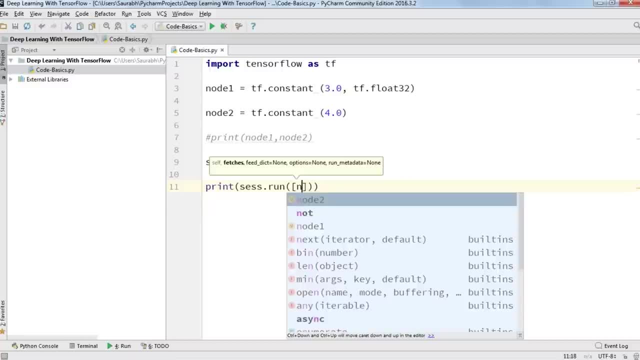 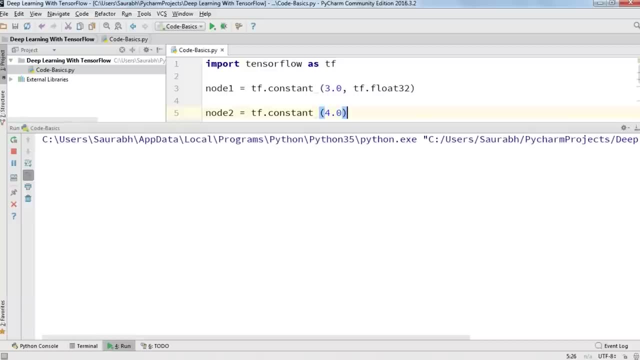 I want to run node 1 and node 2.. So I'm going to type in here: node 1, comma node 2.. That's all. and now, when I run this, it will actually give me the value 3 and 4.. And yup. 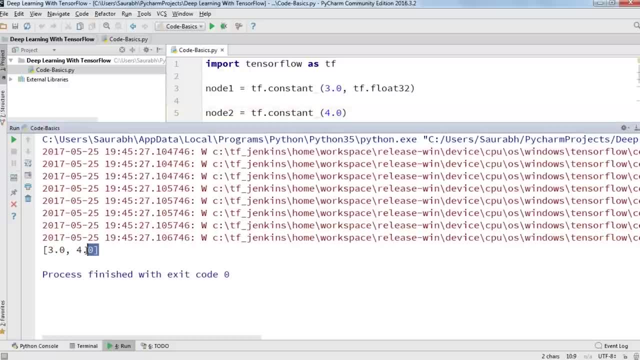 it does? it gives me the value 3 and 4.. So what we did? we first build a computational graph. we first saw how to build a, basically a computational graph, and then we understood that these all are nodes. So in order to get their value, we need to evaluate those nodes. 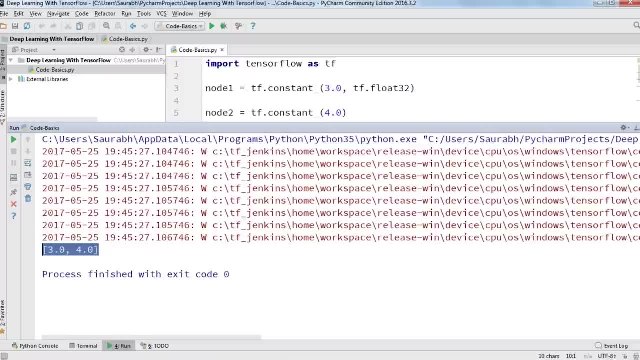 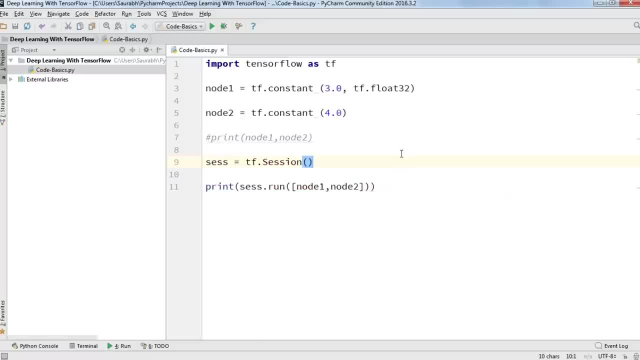 and how we can do that? by running the computational graph inside a session and then, finally, when we run that session, we get the output 3 and 4, which is nothing but the values of those nodes. So any questions, any doubts till here, guys, how to build a computational graph. 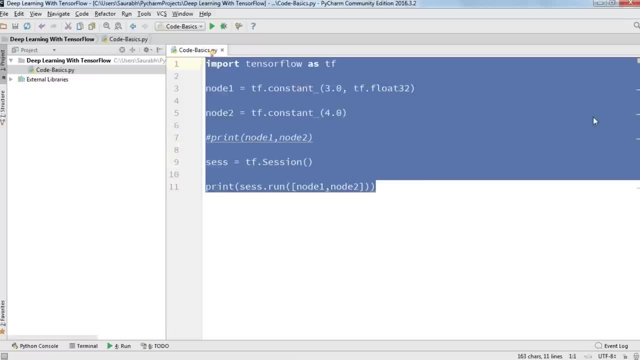 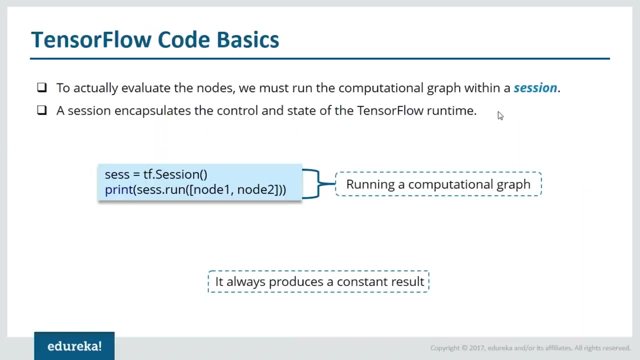 and how to actually run the session. any questions, any doubts? you can ask me straight away. Any questions, guys. Fine, So I've got a confirmation From everyone and no one has any doubts till here. fine, So I'll again open my slides, and the one thing that you must have noticed here is that it will always produce a constant result. 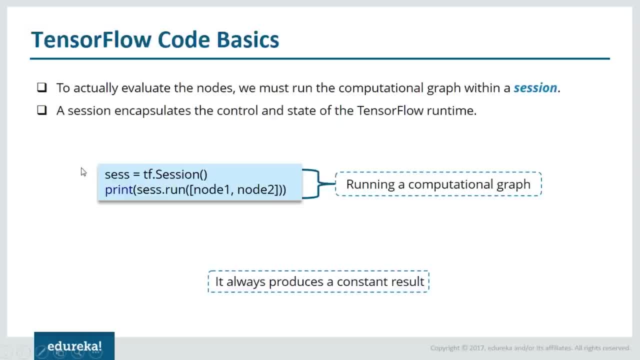 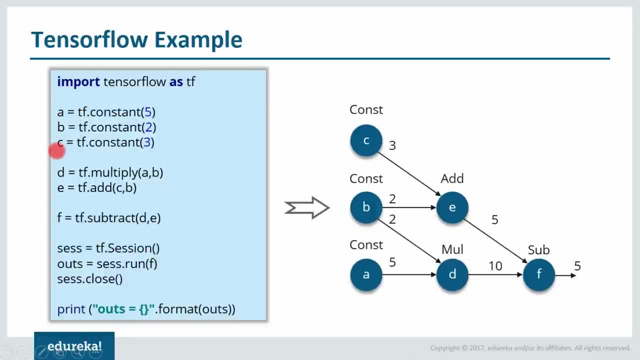 right. So how to actually avoid that? So we saw how to run a computational graph as well. Now let me explain it to you with one more example. So this is one example in which we take three constant nodes- a, b and c- and we perform certain operations like multiplication, addition and subtraction. 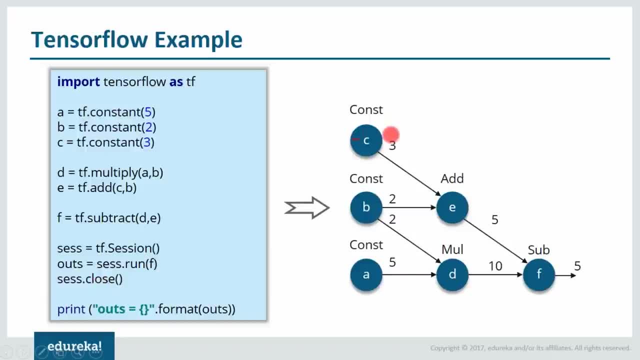 and then we run the session and then we finally close it. and this is the diagram how it looks like. So we have three constant nodes: c, b, a. a contains value 5, b contains 2, similarly c contains 3.. First we add c and b, then we add b and a, then we get two other nodes, that is e and d. 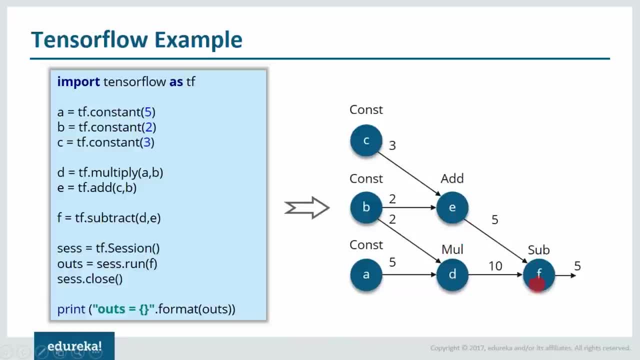 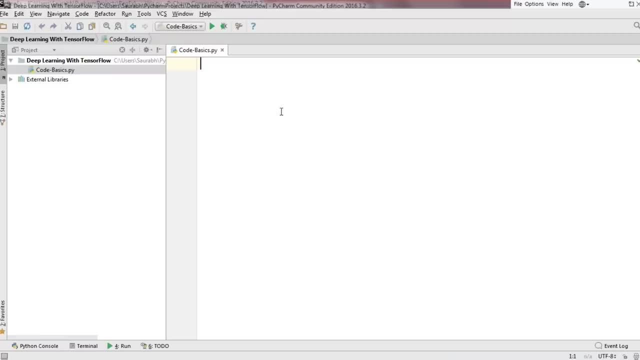 and then from that e and d, what we are going to do is we are going to subtract both of them and then we get the final output. Now let me go ahead and execute this practically in my pie charm. So this is my pie charm again, guys. 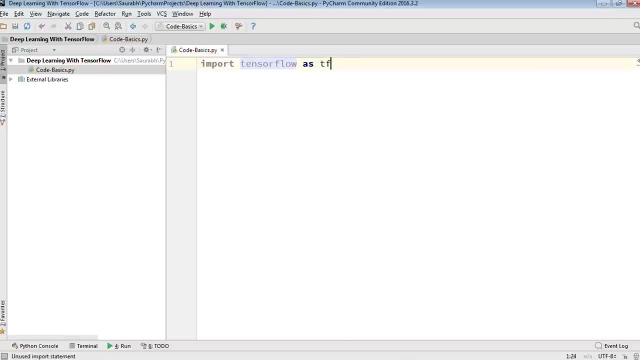 First thing I need to do is import Tenser flow as tf. Then we are going to find the three constant nodes. So first is a, a equals to tf, dot constant, and the value that will be there in a will be 5.. Then I'm going to find one more constant node. 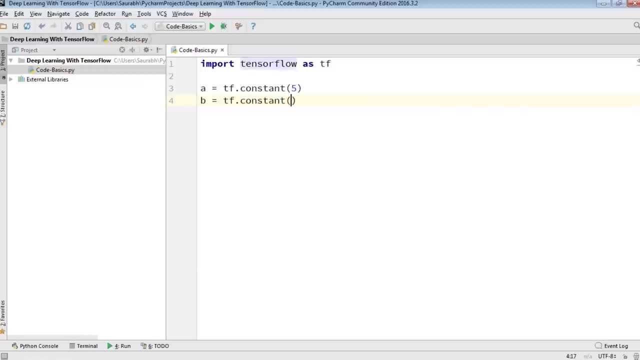 That will be b, tf dot constant and the value that will be there in it will be 2.. And then I'm going to find the last constant node and tf dot constant. The value that will be there is 3.. All right, so we have three constant nodes and now we are going to perform certain operations in them. for that, 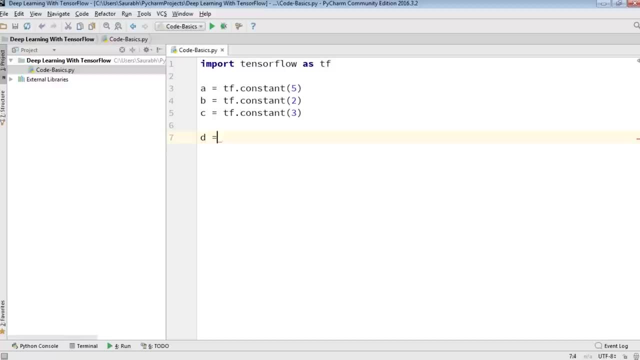 I'm going to find one node, Let it be d, which will be equal to tf dot, multiply So the two nodes that we want to multiply, so that will be a comma b, And then there will be one more node in order to perform some operation that is addition to tf dot. 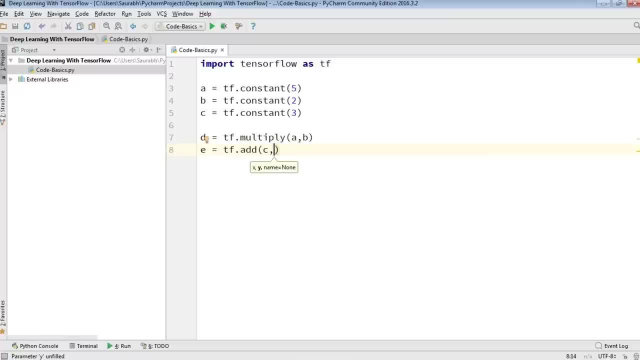 Add, add c and b, And then we're going to find one more node- Let be f- and inside that node We're going to perform the subtraction operation: tf dot subtract D and E. So we have built a computational graph. Now we need to run it, and you know the process of doing. that says is equals to tf dot session. 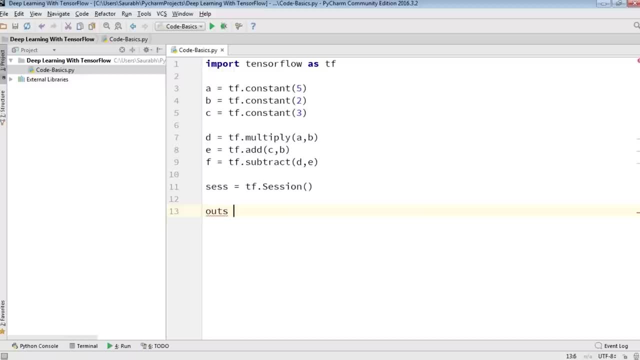 And we are going to define a variable. Let it be O, U T S outs, whatever name that you want to give in, and just type in a says a dot, run F. Let's see if that happens or not, And then we're going to print it for that. 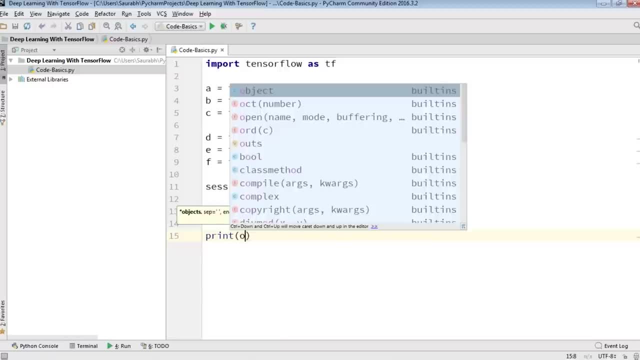 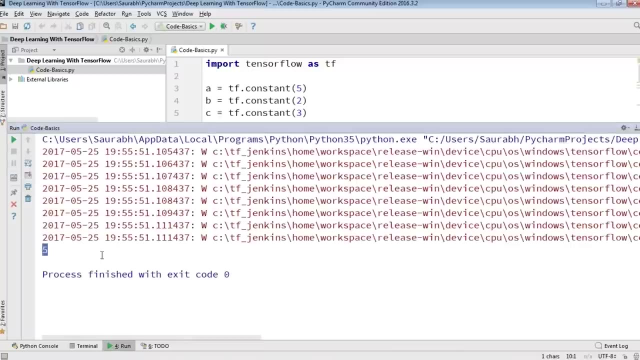 I'm going to type in here, print Out. Let's go ahead and run this and see what happens. So we have got the value 5, which is correct, because if you notice our presentation as well, let me open it for you Over here. 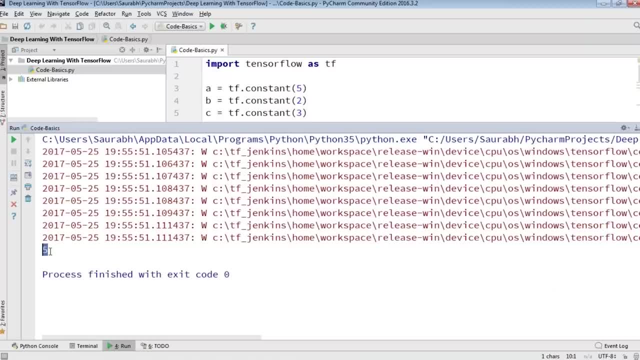 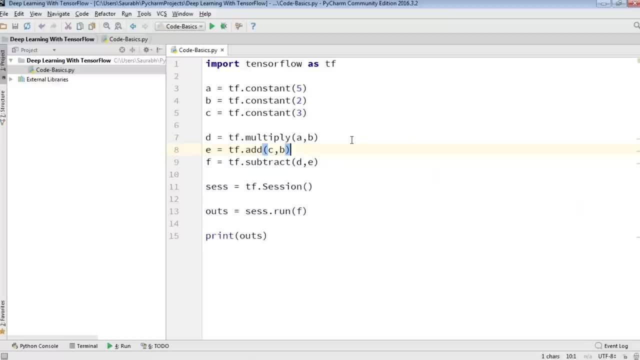 We also. we get the value 5, similar to our implementation, and pie charm as well. So this is how you can actually build a computational graph and run a computational graph. I've given you an example. now, guys, let us move forward, because these are all the constant nodes. 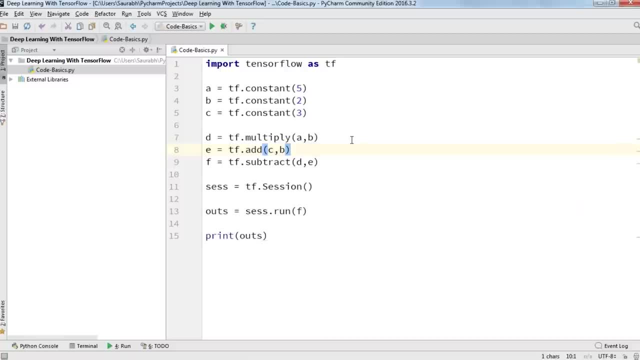 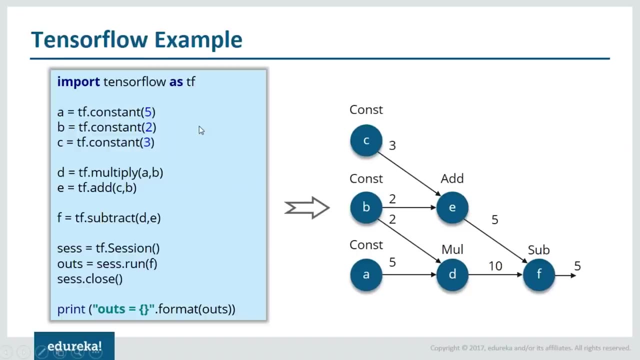 What if I want to change the value that is there in the node? So for that we don't use a constant nodes, for that We use placeholders and variables. Let me explain it to you first. I'll open my slides. So, since these are all constant nodes, 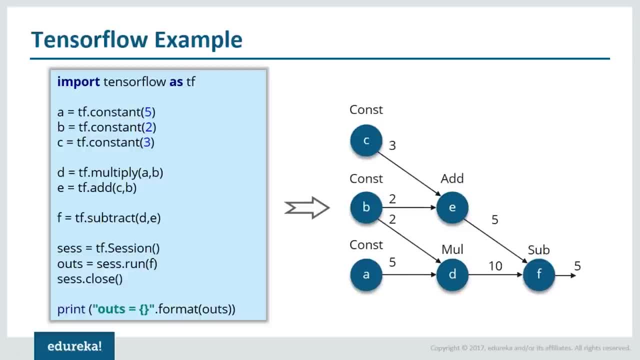 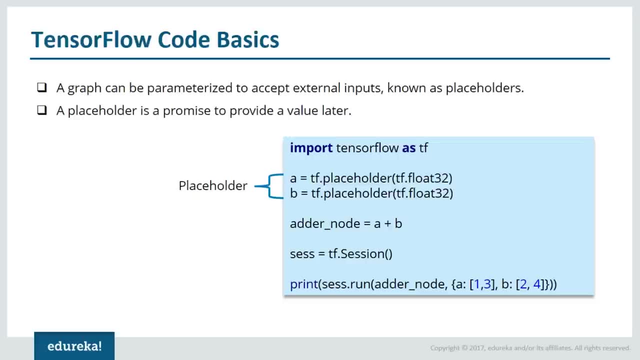 we cannot perform any operation. Once we have provided a value, it will remain constant. So, basically, a graph can be parameterized, except external inputs as well. And what are these? these are nothing but your placeholders, and these placeholders is basically a promise to provide values later. 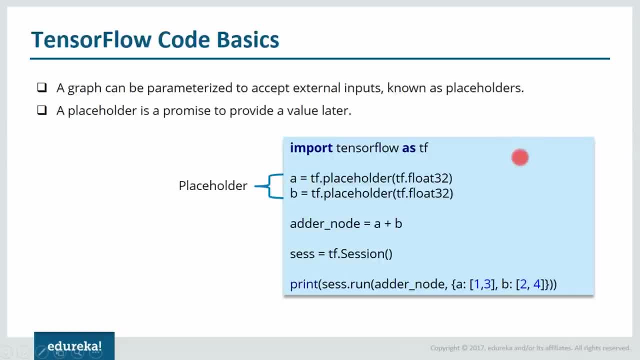 So there's an example that is there in front of your screen Over here. These three lines are bit like a function or a lambda, in which we define a, two input parameters- a and b- and then an operation possible in them. So we are actually performing addition, so we can evaluate this graph with multiple inputs. 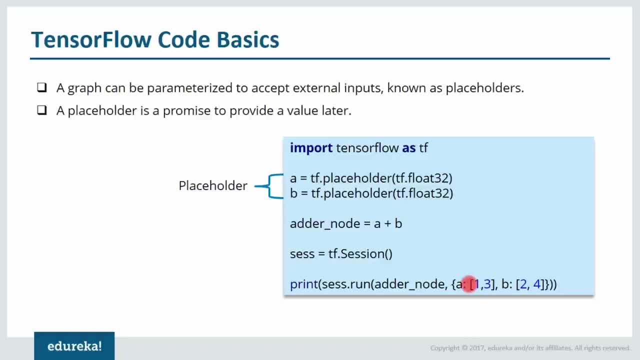 By using feed underscore dict parameter. as you can see, we are doing it here, So we are actually passing all these values to our placeholders here. So these all values will be passed and accordingly, will get the output. So let me show you practically how it happens. 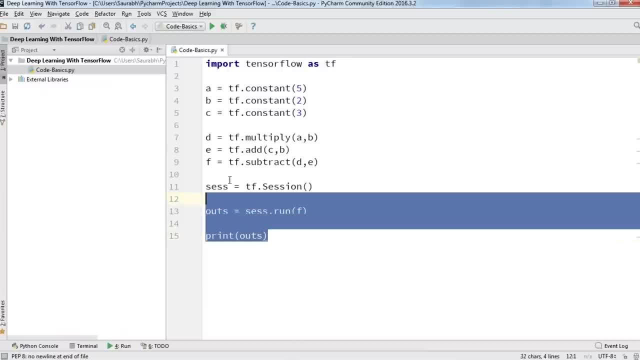 So I'm going to open my pie charm once more. I'll remove all of this. and yeah, so the first placeholder, I'm going to name it as a TF dot placeholder, And what sort of a placeholder It'll be? so I'll consider it as float number of 32 bits. 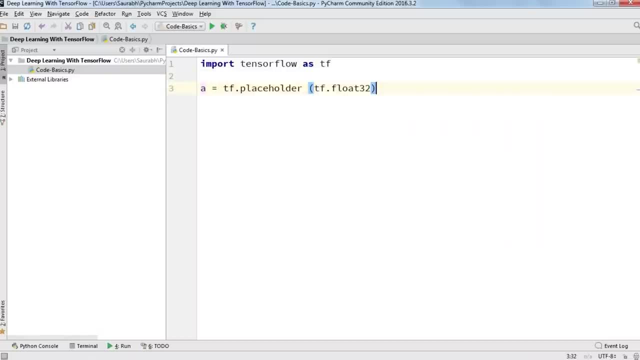 Similarly, I'm going to define one more variable as well. I'm going to name it as B, Then I'm going to define an operation that I'm going to perform them. So I'm just going to type in here: adder underscore node equals to a plus B. 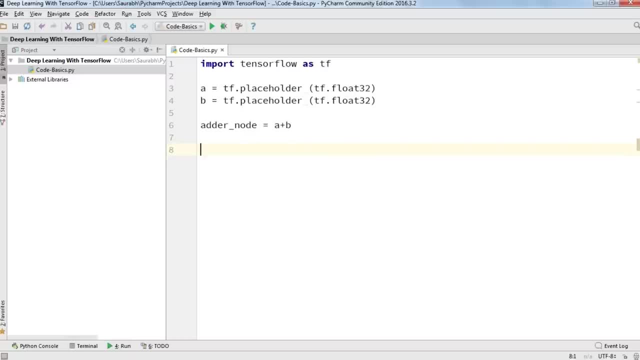 And now our placeholders are currently empty. So that, totally earlier as well, placeholders are nothing but a promise in order to feed values later. So this is how we have built a computational graph. Now Our next step is to start a session. So for that. 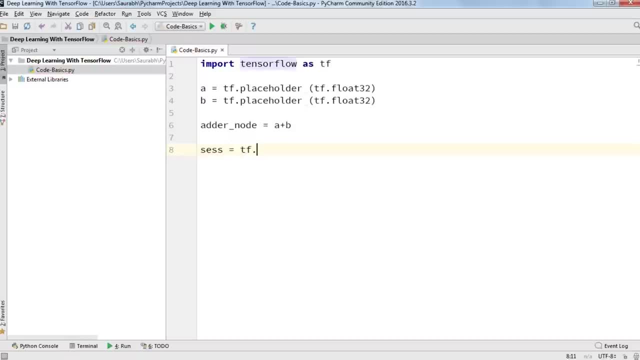 I'm going to type in a assess equals to TF dot session Right, Since these placeholders are currently empty and we know that these placeholders are nothing but a promise, in order to provide them with certain values later. So let's go ahead and provide the values, or you can say a list of values. 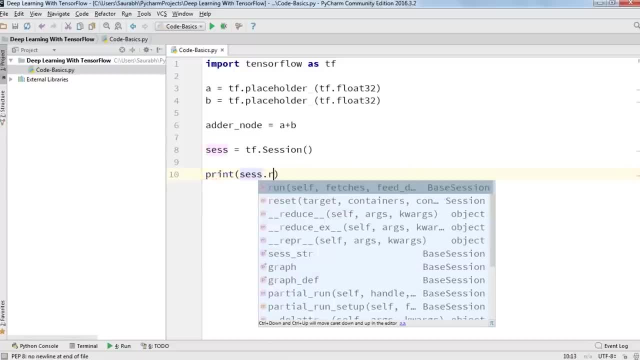 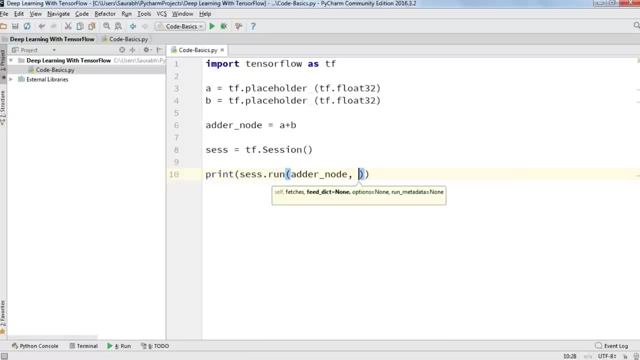 So I'm going to type in here: print says dot, run, Adder, underscore, node, And then the values that I'm going to feed in. So basically I'm going to feed in a dictionary, A colon, 3, a colon- a list of integer values between 1 to 3, and one more will be B colon, a list of integer values between 2 and 4.. 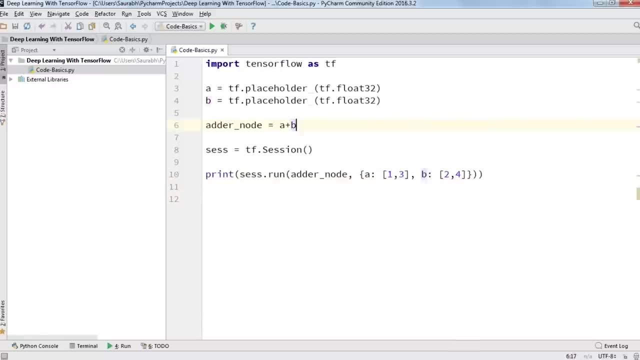 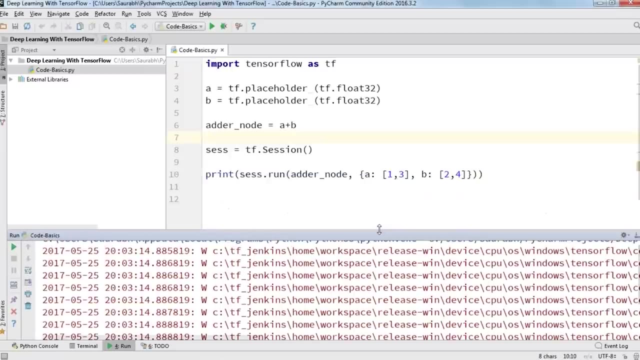 All right, so this is done. now Let us go ahead and execute this and see what happens. So we have got the output of 3 and 7.. So basically, if you add 1 and 2, you get 3. similarly, you add 3 and 4, you get 7.. 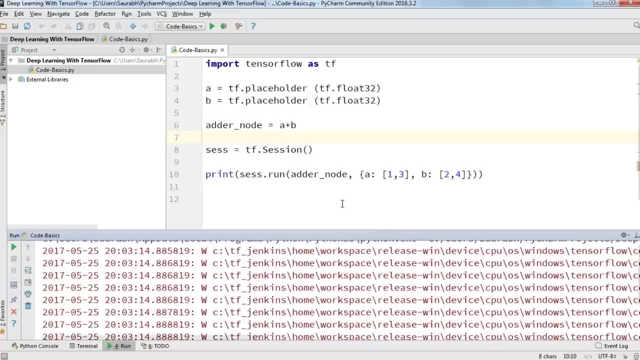 It's pretty easy mathematics, but my main focus was to make sure that you understand what our placeholders. So I hope you have got the concept. If you have any questions, any doubts, you can write it down in the chat box. Any questions, guys? 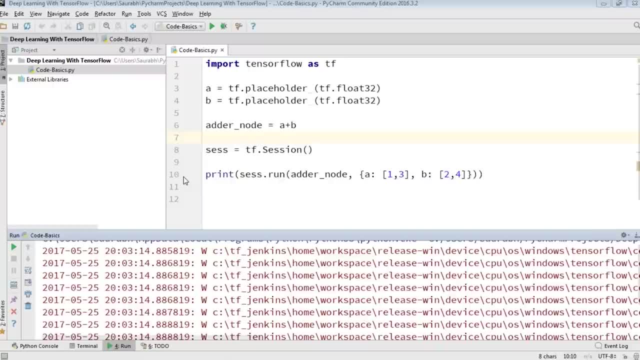 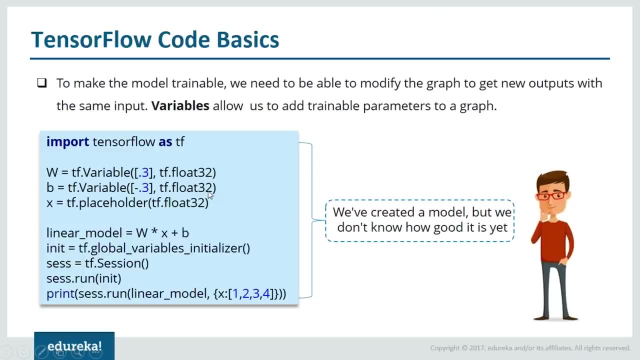 Fine guys, So we have no questions here. So I'm again going to open my slides and we'll see what's up next. So we understood what exactly our placeholders. now the time to understand what our variables. So basically, in deep learning, we typically want a model that can take arbitrary inputs. now, in order to make the model trainable. 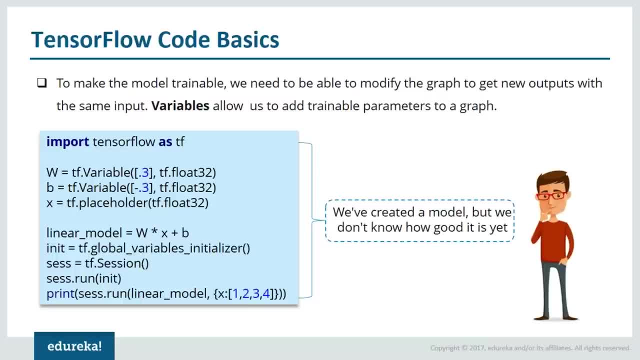 We do able to modify the graph to get new outputs with the same input, and what helps us to do that? variables basically allows us to add a trainable parameters to our graph. So, in order to declare variables, what we do is you can refer the code that is there in front of your screen. 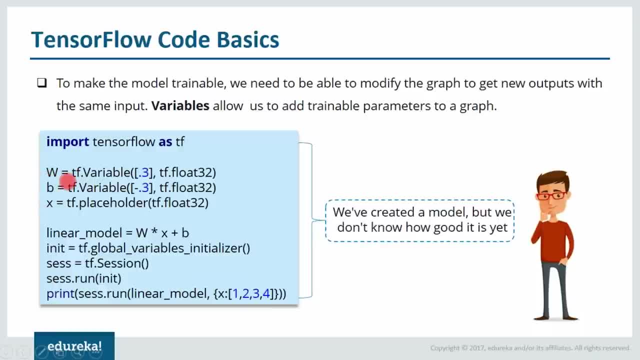 So we have taken two variables in one placeholder and the first variable has a value, point Three. the other variable has minus 0.3 and the placeholder, obviously it will remain empty and then later on we feed in some values to it. Then we create a linear model. 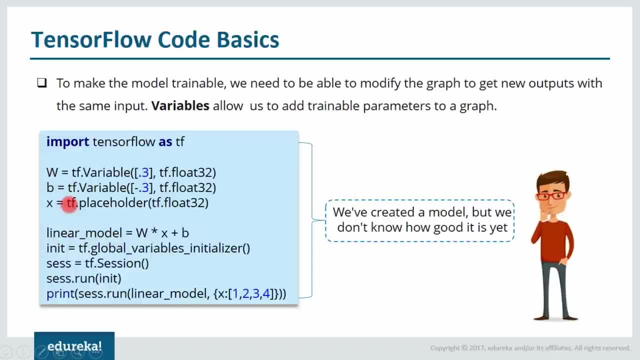 or you can say some operation in which we are going to multiply this W with X and then we are going to add a bias or a B value to it. Then what we need to do is we need to initialize all the variables in the tensorflow program. 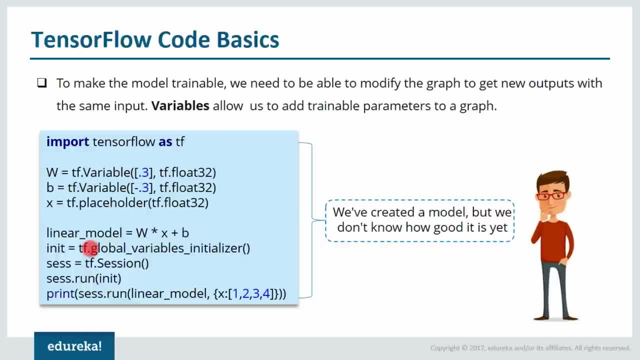 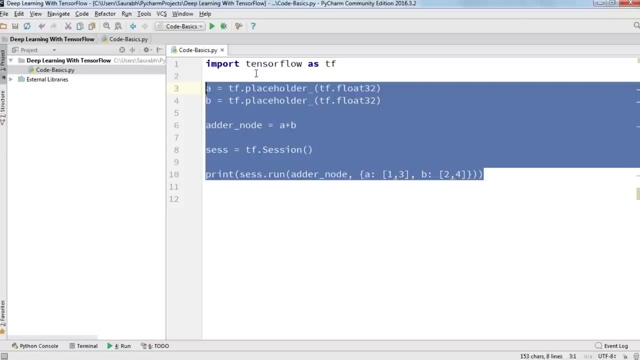 So for that you must explicitly called a special operation, which is a TF dot- global variable initializer, and then just directly run the session. Now let us go ahead and execute this practically, guys. Let me remove all of this. Yeah, so our first variable will be a W and we are going to call in a TF dot variable. 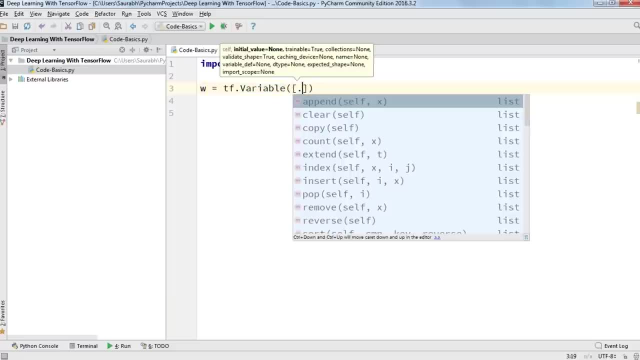 And in that variable we are going to store a value which is 0.3.. And it is of a flow type 32 bit. So just type in here: TF, dot, flow 32.. Yeah, then we're going to define one more variable. 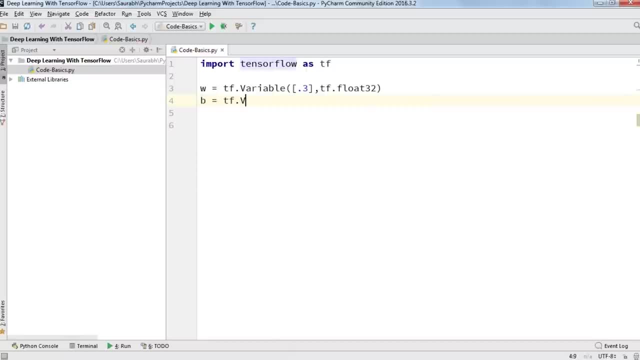 Let it be B. So I'm going to type in a TF dot variable And the value of this variable will be minus of 0.3.. Again, it is float type of 32 bit, So just type in that TF dot, float 32.. 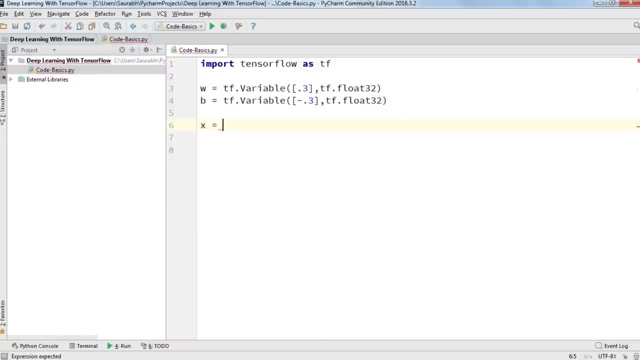 Now I'm going to define a placeholder that is X- X is equals to TF- a dot place holder and it is again a float type 32 bit And then some operation that we are going to perform. So I'm going to type in here: linear underscore model. 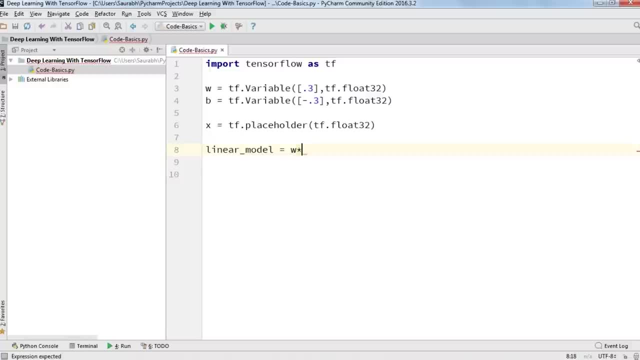 equal to W multiplied by our X value. That is a placeholder, and then we want to add bias to it or B value to it. All right, Now, as we have seen earlier as well, in order to initialize constants, we call TF dot constant, and their value will never change. 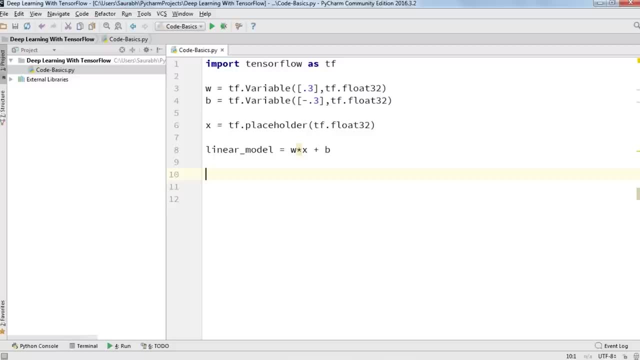 But, by contrast, variables are not initialized when you call TF, dot variable. So to initialize all the variables in the tensorflow program, what you need to do is you need to explicitly call a special operation. and how you're going to do it, Just type in here: 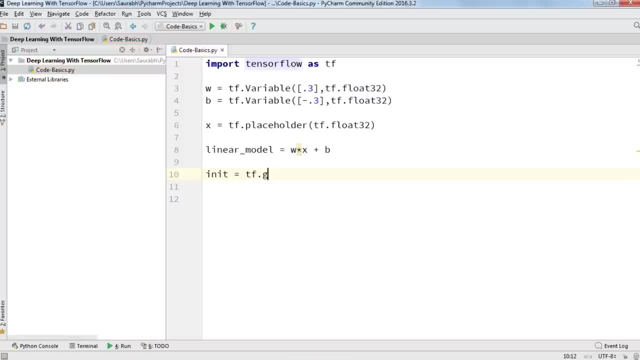 I net. equal to TF. a dot: global Underscore variables, Underscore initializer. That's all and then, and then we're going to run a session. So you know the process says is equals to TF: dot session. I net. 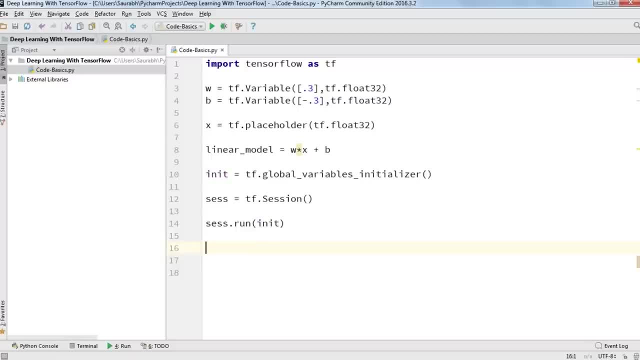 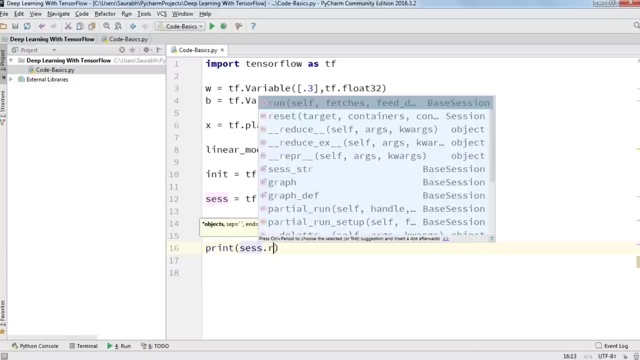 Now let's print it, And before that, what we need to do is need to provide the X placeholder with some values. will actually going to do that at the print statement itself, So I'm going to type. it says: dot run, Run what run a linear model. 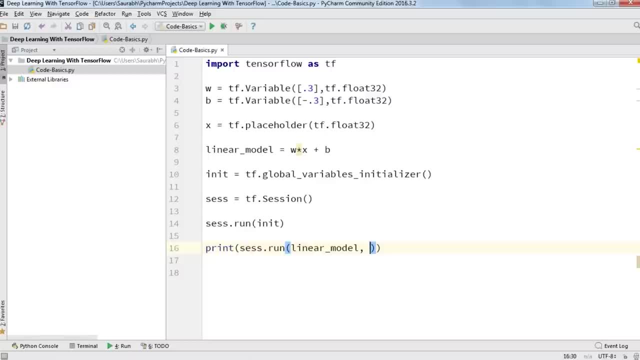 And the values that we are going to pass in. X will be a dictionary again And let me show you how you can do that. So X colon and it will be a list of values from 1 comma, 2 comma, 3 comma, 4.. 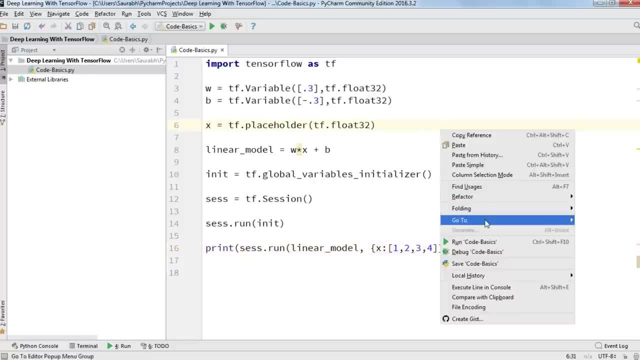 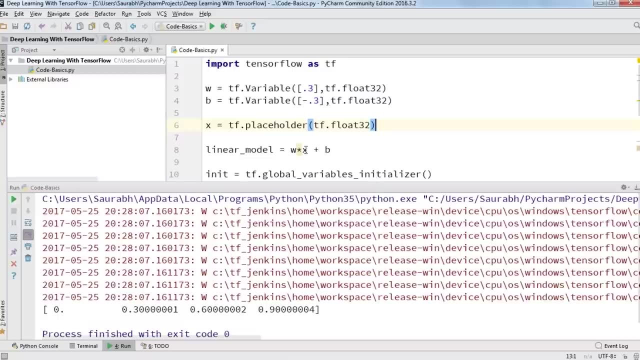 Yeah, that's all, and we are going to run it now. So this is how we get the output. It's simple mathematics, What we have. the first value of W will be 0.3 and the first value of a, B, will be a minus 0.3. 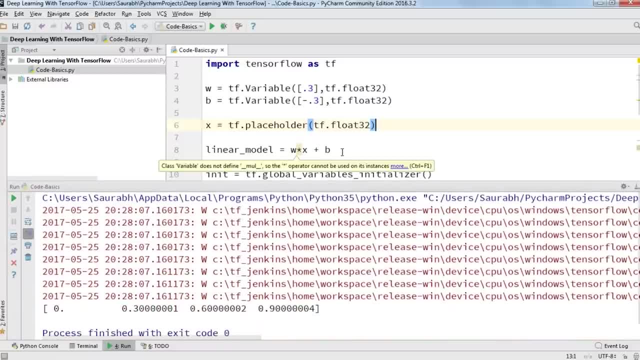 and the first value of X will be 1, so it will be 3 minus 3, which is again 0. similarly For other values as well. You can calculate it. It's absolutely correct. So what we have done? we have created a model. 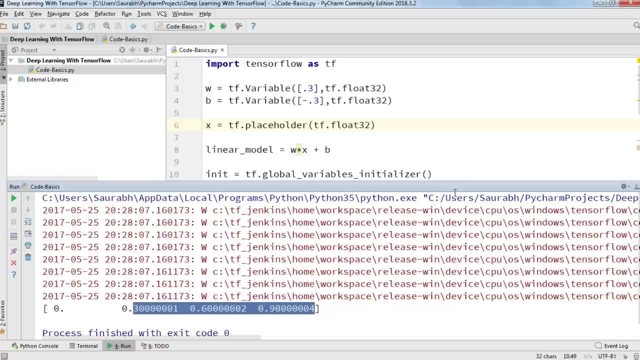 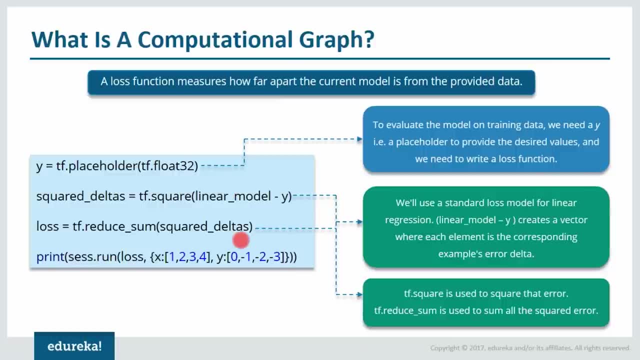 but we don't know how good it is yet, So let's see how we can actually evaluate that. for that I'm again going to open my slides. So now, in order to evaluate the model on the training data, we need a placeholder. 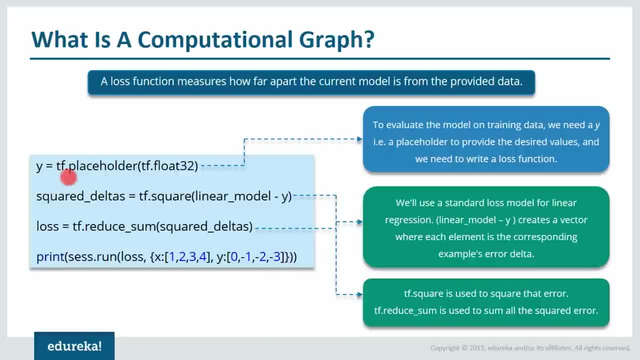 Why, as you can see in front of your screen, to provide the desired values and we need to write a loss function. So this placeholder Y will actually be provided with the desired values for each set of inputs and then we're going to Calculate the loss function. 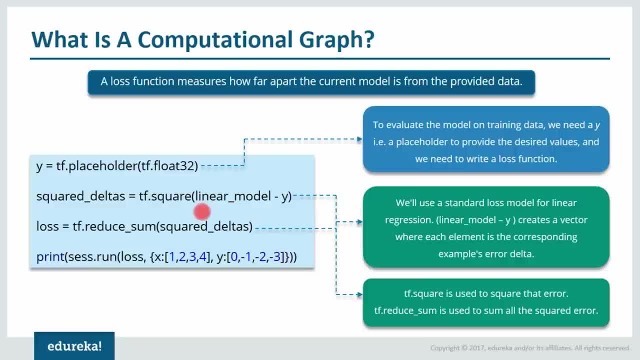 And how are we going to do that? We're going to minus the actual output with the desired output, and then we're going to do the square of it. after that, We're going to sum all of these square deltas and then we're going to define one single scalar as loss. 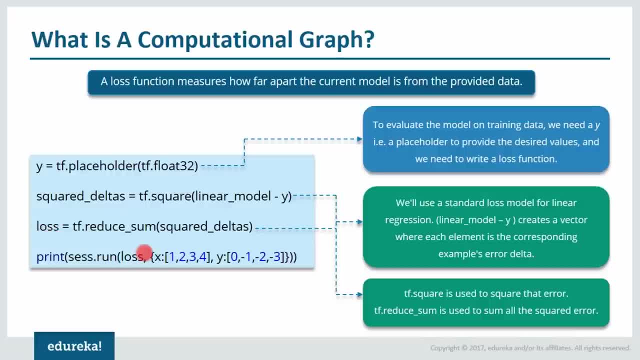 So this is how we are actually going to calculate the loss, and then, after that, we need to provide the values to X and Y placeholders. So what I'm going to do, I'm going to open my pie charm and then I'm going to show you how correct our model is on the basis of the values. 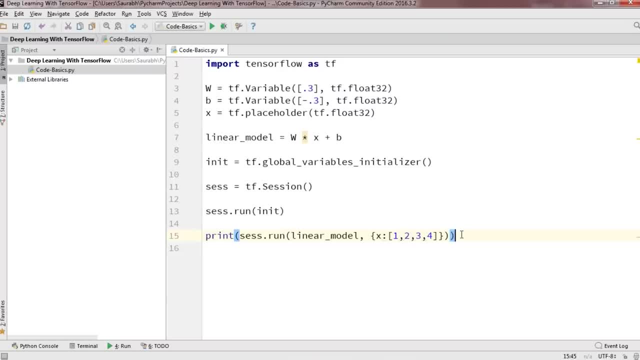 That we provide to Y placeholder. So, guys, this is my pie charm again. And since here I what I'm going to do is I'm going to define a placeholder first. Y is equals to TF dot, placeholder, TF dot- float 32.. So I'm going to type in a TF dot, float 32, square Delta. 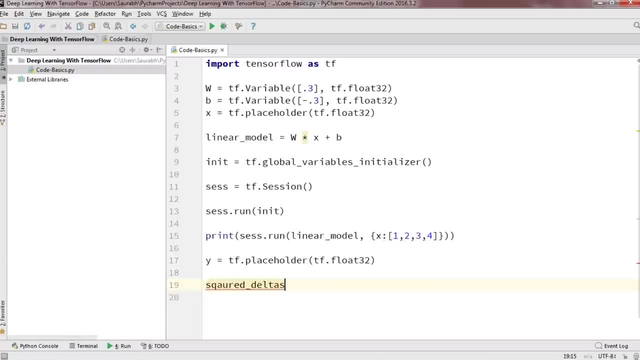 I've explained you all these things, but yeah, I'm going to tell it to you again as well, Don't worry about it. TF, dot, square, The actual output minus the desired output, And then I'm going to sum all those losses, or you can say square deltas. 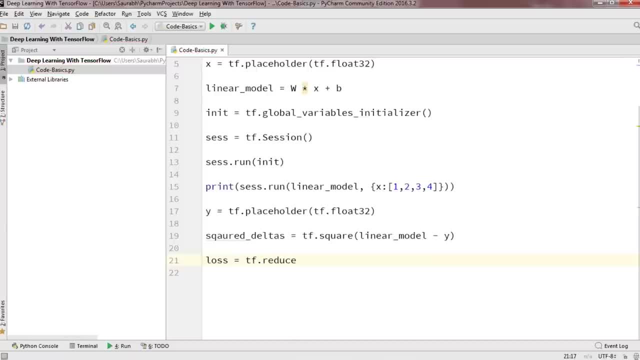 TF dot reduce Underscore sum. So I'm going to type in here: square deltas. Then finally print it. So I'm going to type in: cess dot run Loss X colon 1 comma, 2 comma, 3 comma 4.. 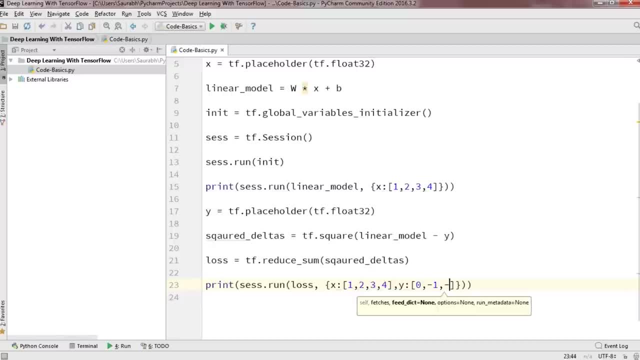 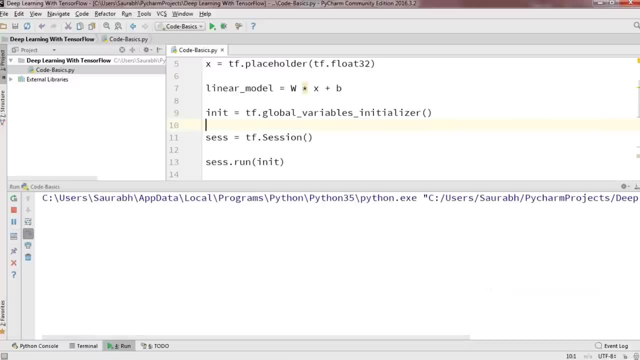 0 comma minus 1 comma, minus 2 comma minus 3.. And that's all, and we are good to go. Let's run it and see what will be the loss. So the loss is 23.66,, which is very, very bad. 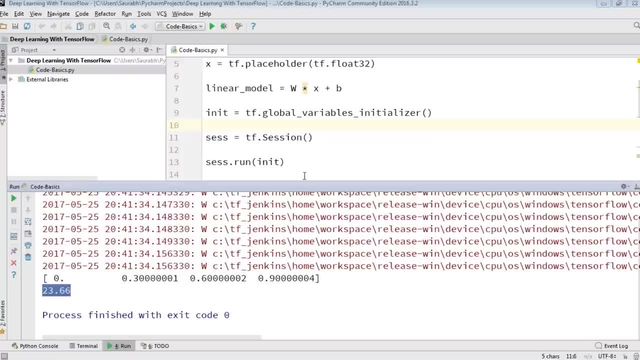 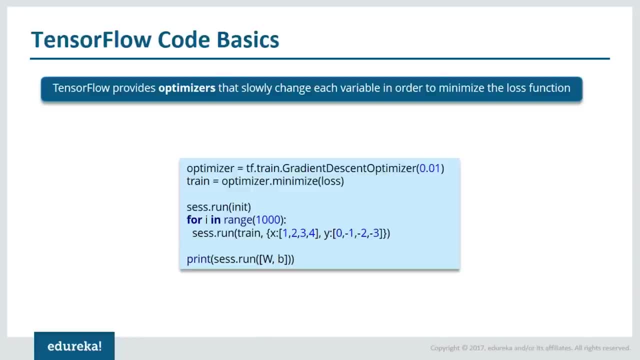 Now our next step is to realize how to actually reduce this loss. So let's go ahead with that. I'm going to open my Slides once more. So, in order to minimize the error, Now in order to reduce this loss, TensorFlow provides optimizers that slowly change each variable in order to minimize a loss function. 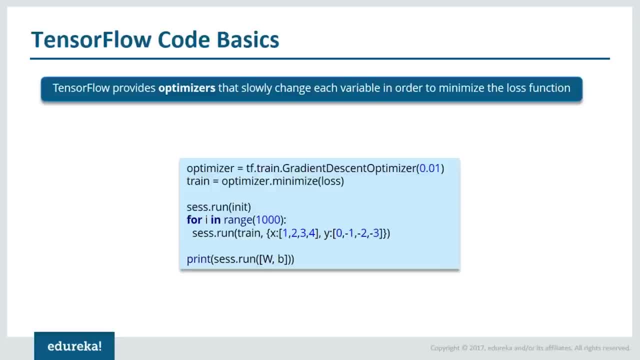 And the simplest optimizer is gradient descent. In order to do that, we have to call the function called TF dot gradients. So, as you can see it in the code itself, so we have a TF dot train dot gradient descent optimizer, and this is nothing but the learning rate 0.01.. 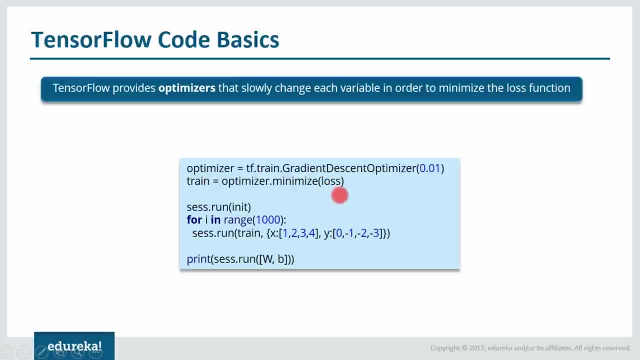 Then train equals to optimize, Dot, minimize the loss. So we're going to call this optimizer, which is nothing but the gradient descent optimizer, in order to minimize the loss, And then we are going to run it. So let's see if that happens or not. 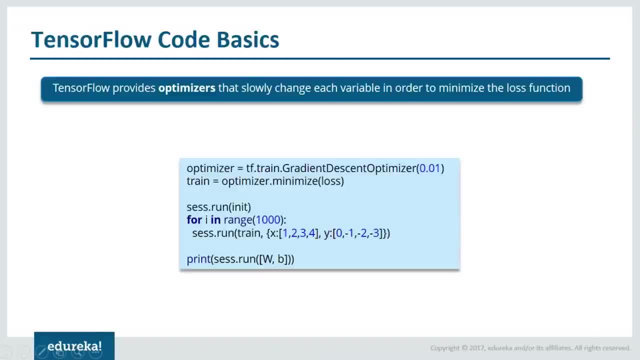 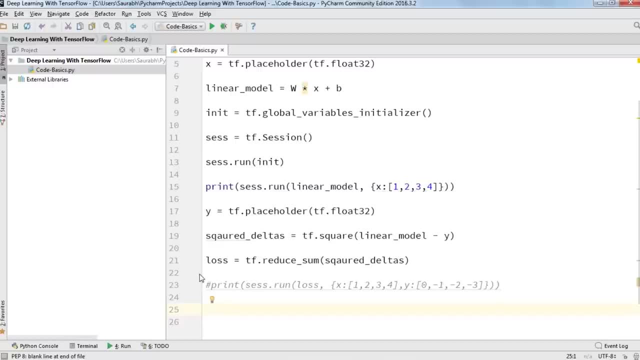 So for that again I'm going to open my pie charm, And over here let me first comment this print statement And now I'm going to type in here: optimizer equals to TF, dot train Gradient descent optimizer And the learning rate will be 0.01. and guys, 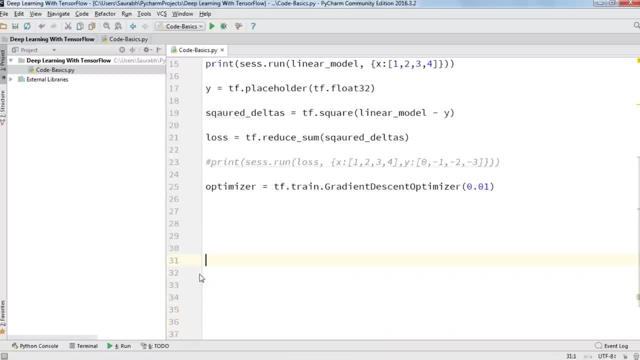 let me tell you this is just an introductory session to TensorFlow and deep learning. So all the modules that we have discussed in the beginning will be covered in detail. So whatever topics are there in those modules will be covered in detail, So you don't need to worry about it. 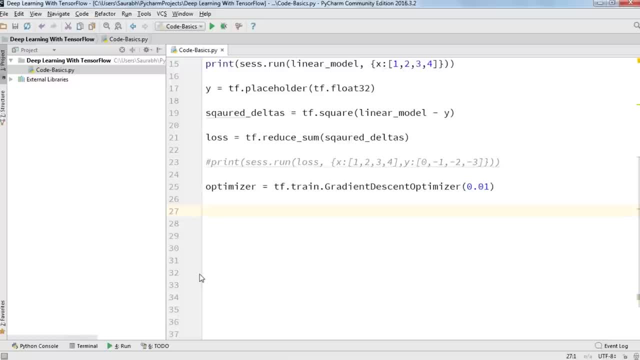 So I'm just giving you a general introduction and overview of how things work in TensorFlow. All these things, all these gradient descent optimizers, all these things will be discussed in detail In the upcoming sessions. Now I'm going to type in here: train equal to optimizer dot minimize loss. 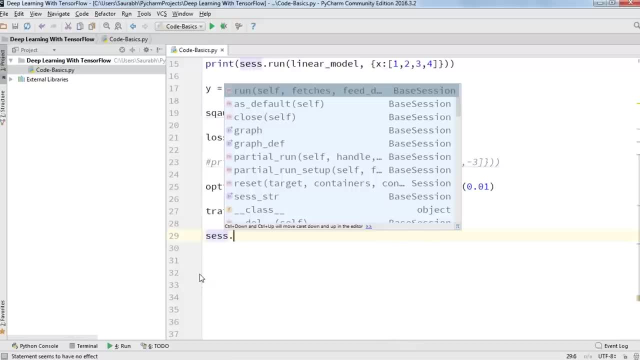 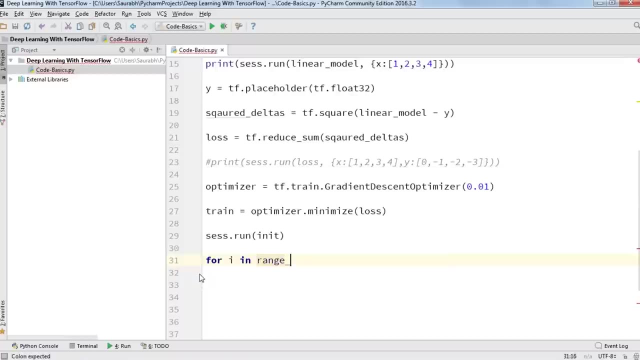 And then now let's go ahead and run. this says dot run, I in. it Says dot run, and we're going to feed in values to our X and Y placeholders. Train comma X will have values 1, 2, 3, 4.. 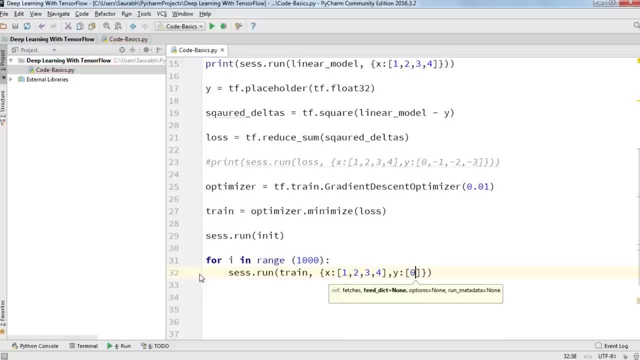 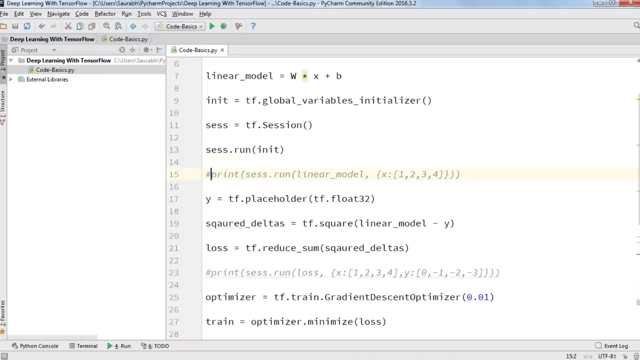 And Y will have values 0 comma minus 1 comma minus 2 comma minus 3.. Print says: dot run W comma P. Now let me first go ahead and comment these lines. All right, so I've just made a mistake here. 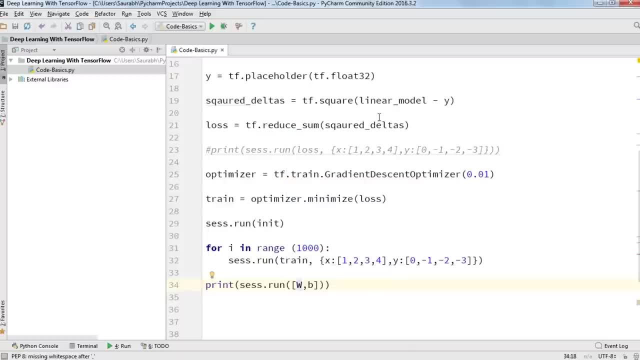 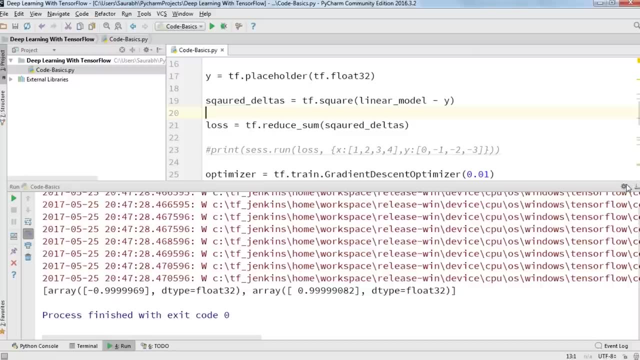 This is in uppercase W and yeah. so now we are good to go and let's run this and see what happens. So these are our final model parameters. So the value of a W will be around the point nine, nine, nine, nine, six, nine, and the value of our B 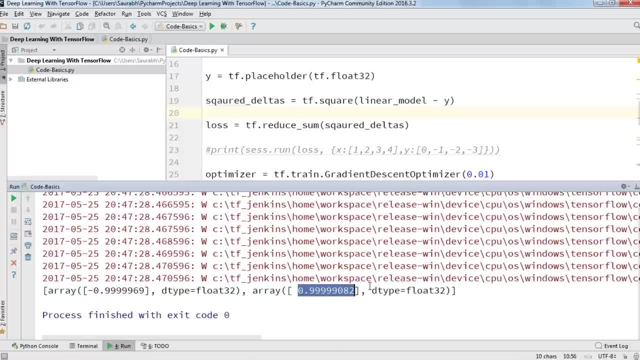 Will be around a point nine, nine, nine, nine, zero, eight, two. So this is how we actually build a model, and then we evaluate how good it is And then we try to optimize it in the best way possible. So I've just given you a general overview of how things works in tensorflow. 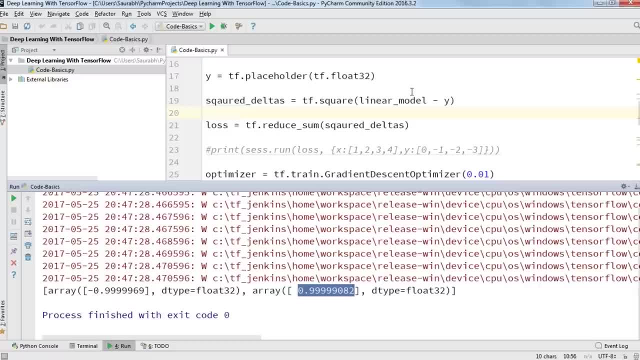 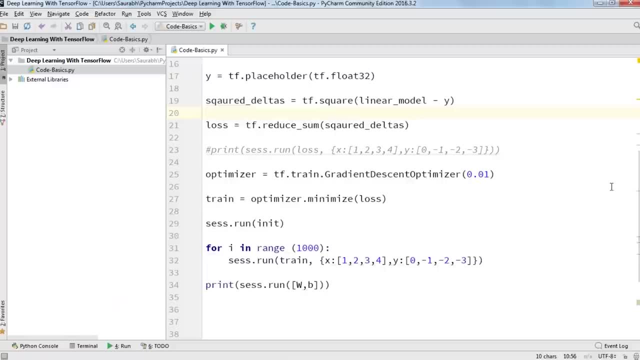 and in the later modules on the upcoming sessions, We are actually going to discuss tensorflow in much more detail. So now is the time to actually implement the and and or gate that I was talking about at the beginning of the session. So for that, let me first remove all of this. 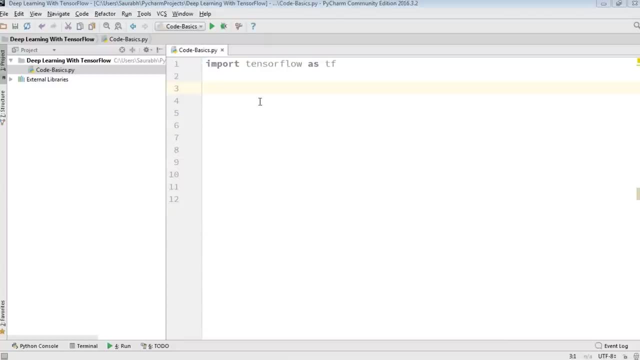 Yeah, Now, in order to implement and gate our training, data should consist of the truth table for and gate, and we know that root table and we know that if any of the input is low, then the output will be low, and and if both the inputs are high, then output will be high. 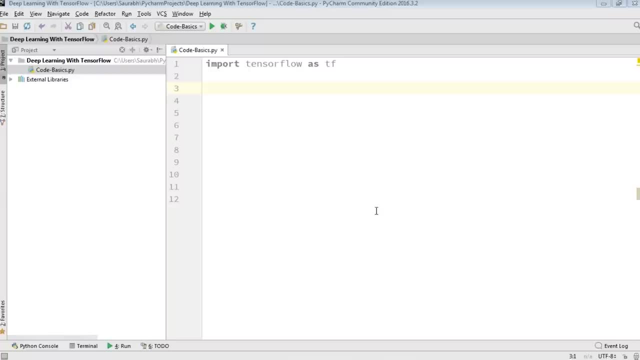 One thing to note here, guys, is that the bias is implemented by adding an extra value of one to all the training examples. So yeah, enough of the explanation, Let's go ahead and code it. So I'm going to type in here: T comma F equal to one point. 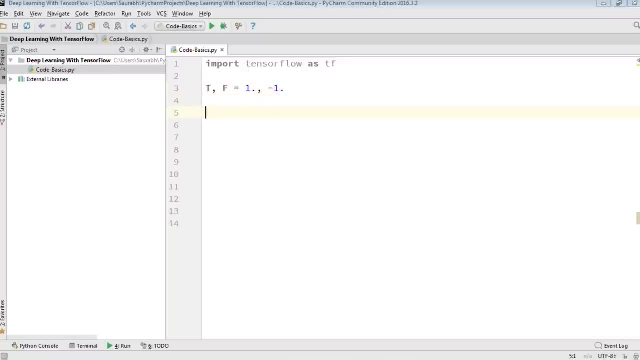 Comma minus one point and bias will always be one. So I'm going to type in here: bias is equals to one point zero, and now I'm going to provide the training data. So for that I'm going to type in train, underscore in equal to: if one input is true and the another input is also true. 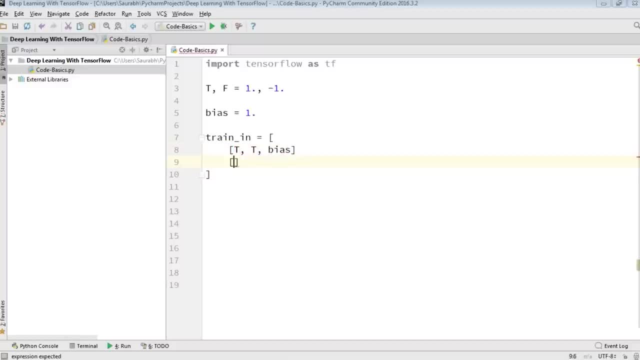 Then we have bias. Then again, if one input is true, the other input is false, Then also we have bias. Similarly, one input is false, Another input is true, Then we have bias. And then finally, when both the inputs are false or zero, 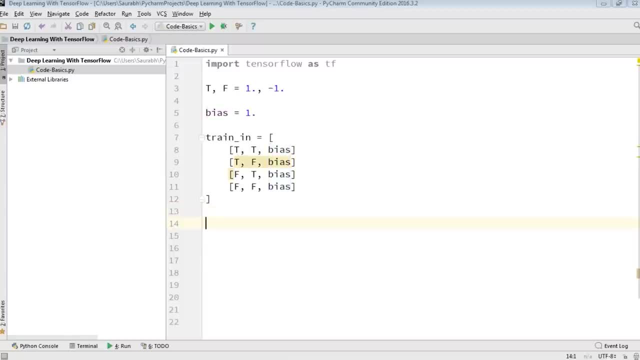 Then we have bias Right. This is our training data and the train out will type in here as the output, basically train underscore out, will be equal to. So yeah, if both the inputs are true or both the inputs are one, then output is true. 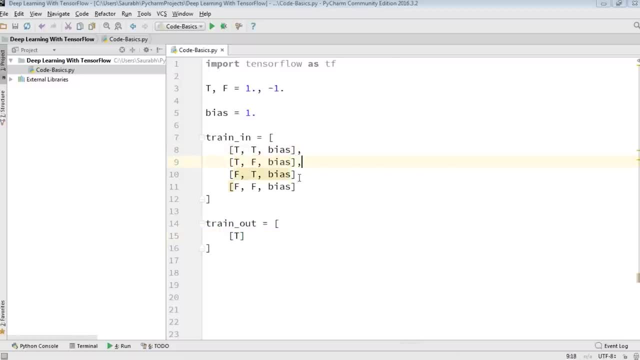 Oops, I forgot a comma everywhere. Let me just go ahead and do that. Yeah, so if both the inputs are true, the output will be true. If any of the input is false, output will be false. So I'm just going to type in here: falls everywhere, because there's only one condition in which we have the true output. 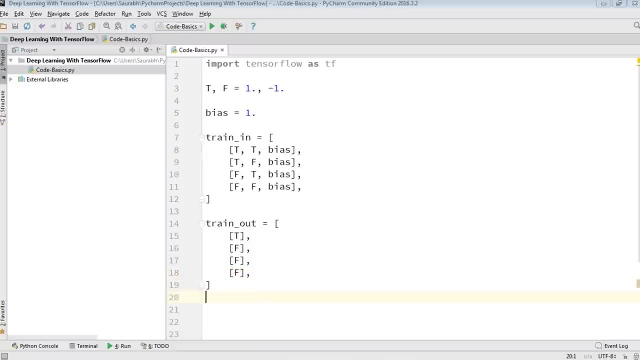 All right. so this is done now. Now, as we know that tensorflow works by building a model out of empty tensors, then plugging in known values and evaluating the model, like we have done in the previous video, This example, since the training data that we have provided, will remain constant. the only special tensorflow object. 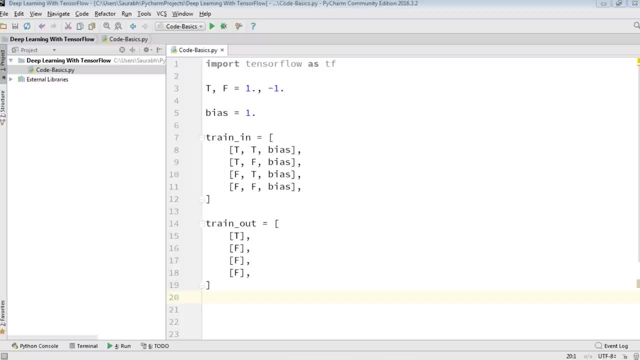 We have to worry about in this case is our 3 cross 1 tensors of vectors. And now what are we going to do? We're going to define a variable and we are going to put in some random values in it. So I'm just going to type in TF a dot variable. 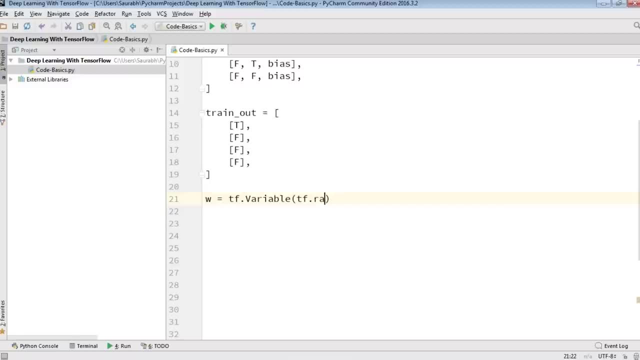 And generate the random function: TF dot, random underscore, normal 3 comma 1.. Now what it is? it is basically a variable, so its value may be changed on each evaluation of the model as we train, with all values initialized to normally distributed random numbers. 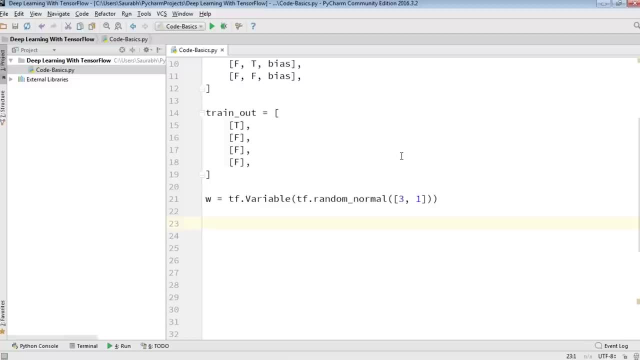 Now that we have our training data and weight tensor, we have everything needed to build a model using tensorflow. So what we need to do, we need to define an activation function and we are going to define a step activation function or step function. So for that, what I'm going to write here is: 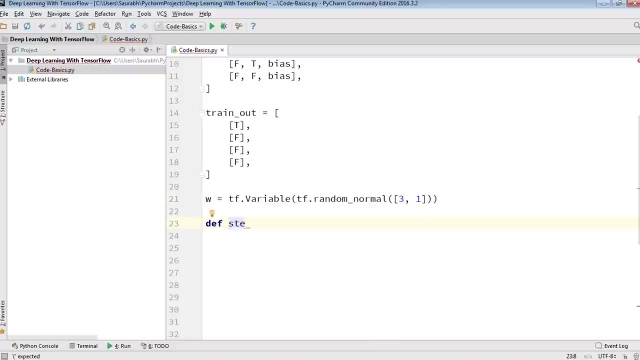 A function step. we're going to define our own step function, although you can use the predefined function as well. that totally depends on you. I'm going to type in here: is Greater equal to TF, dot, greater X, comma 0.. Then we're going to define one more variable as float. 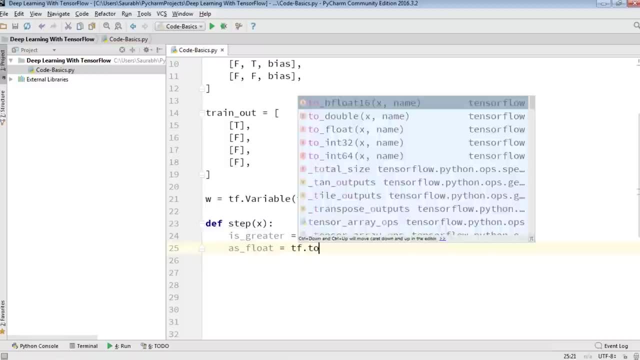 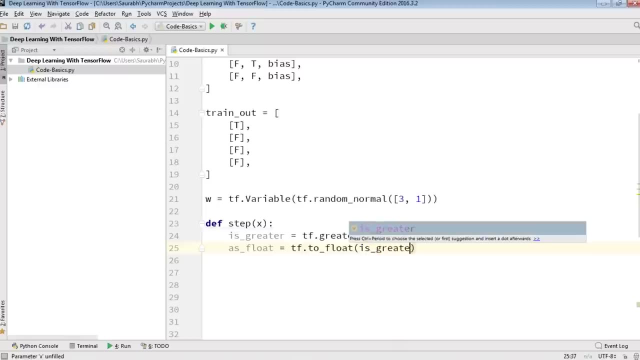 TF dot TO. Then we're going to define one more variable: a doubled equal to TF a dot multiply As underscore float Comma 2.. Then return TF dot Subtract As underscore float Comma 2.. Then return. 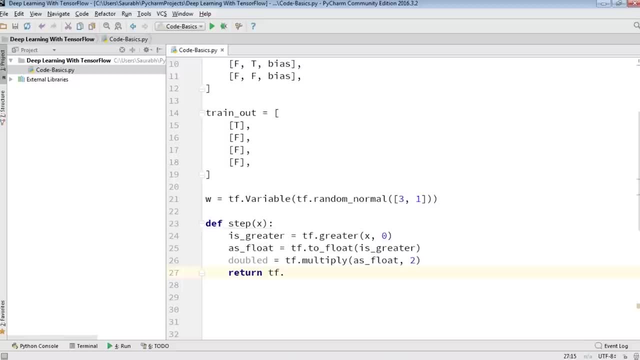 TF Dot Subtract, Double Comma 1.. So now, this is how we have defined our step function. So with the step function defined, the output error and the mean squared error of our model can be calculated in one short line each. 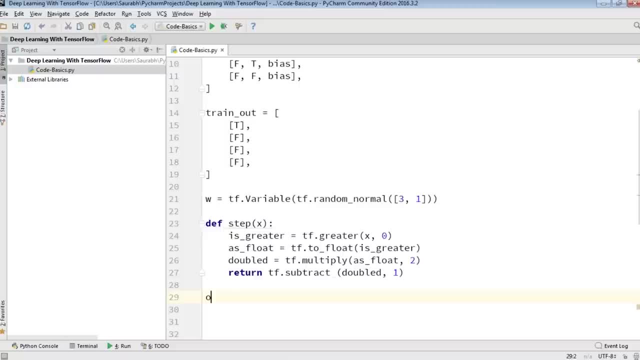 Let me show you how you can do that. So just type in here: output Equal to call that function. that is step TF. dot matrix multiplication: matmul Train- Underscore in Comma W. Now for error. we're going to type in here: 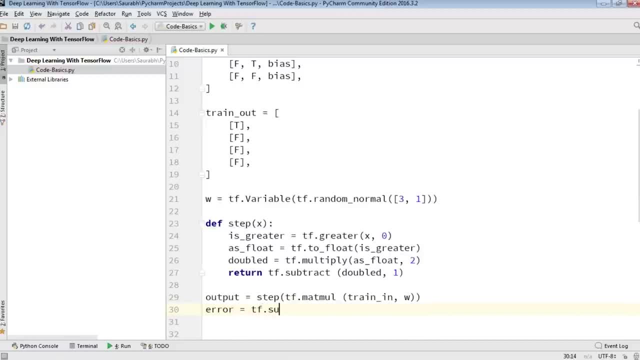 Error equals to TF dot subtract Train underscore out Comma output. And for mean squared error, I'm going to type in here: MSC Equals to TF dot reduce Underscore, mean, TF Dot Square And then error. Now the evaluation of certain tensor functions can also update the values of variables like 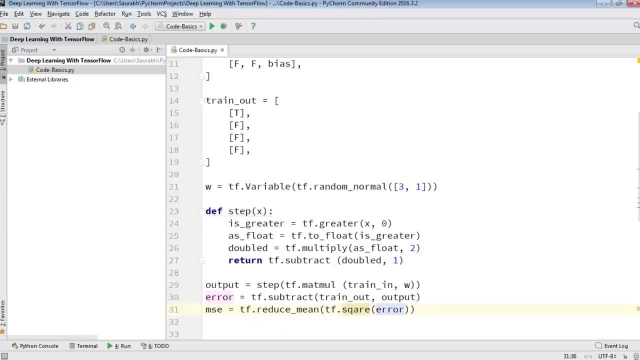 our tensor of weights W. So in our case, basically, we're going to update the weights W. So first we calculate the desired adjustment based on error, Then we add it to W. Now let me show you how we'll do that. So, if you can recall, we have done that in the previous example as well, where we were 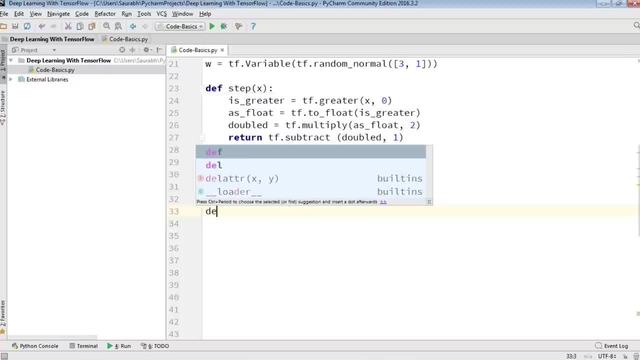 updating the weights and biases. So now I'm going to type in here: delta is equals to TF, dot, matmul, or you can say matrix multiplication. Train Underscore in Comma Error. Comma Transpose Underscore a. 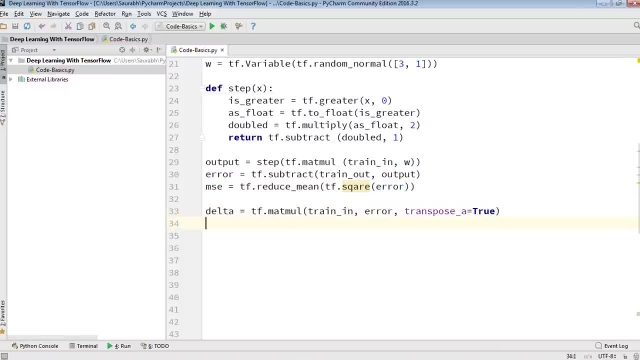 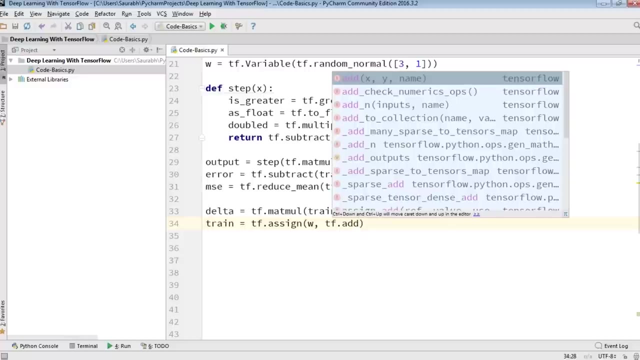 Equals to true, Then we're going to type in here: Train Equal to TF Dot. Assign W Comma TF Dot. Add W Comma Delta. So first matrix multiplication and then we're going to add it all. 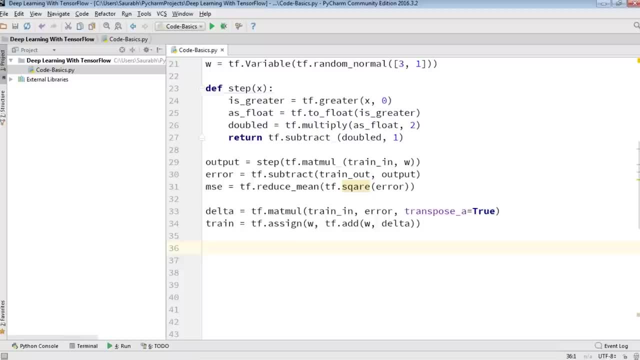 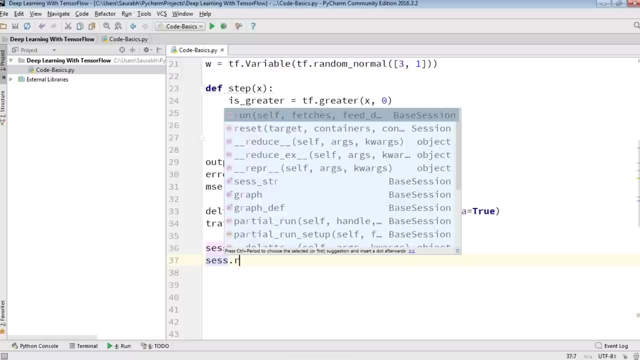 The model has to be evaluated by tensorflow session, which we have seen earlier as well. But before that we also need to initialize all the variables. So first let me just type in here: says equals to TF, Dot Session Add. And then I'm going to type in here: says dot run. 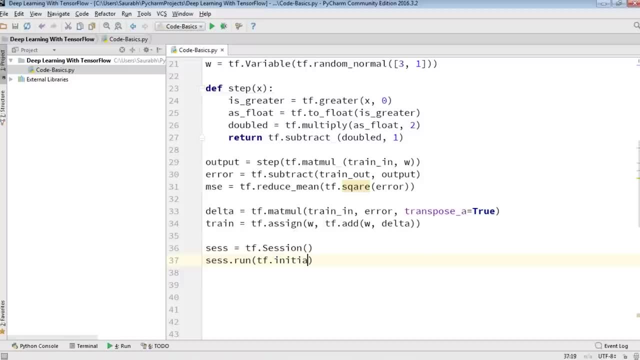 TF, Dot, Initialize, Underscore all Variables. So now what our next task is in order to perform various iterations so that we get zero error. So what we're going to do, we're going to define a variable, ERR and our target. 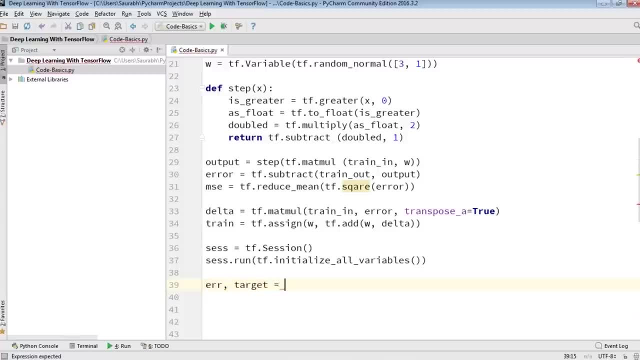 So, basically, our ERR Is nothing but error, which can be equal to 1 or 0, because we are using binary output. So our error can be 1 and our target is to make it as 0 right now. next, what we're going to do: 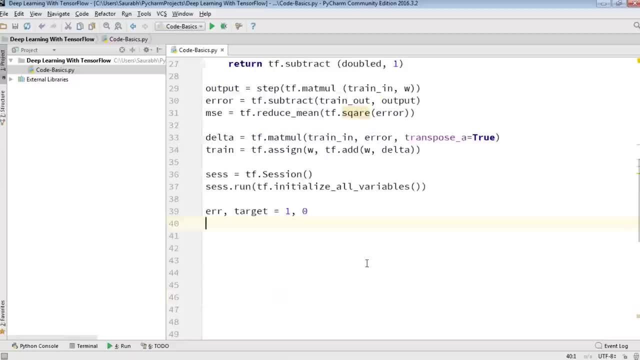 We're going to define a park Now. you can consider right now a park as nothing but the number of cycles, or you can say number of iterations that will be required in order to reach the desired output. or you can say, in order to reduce the error to 0. 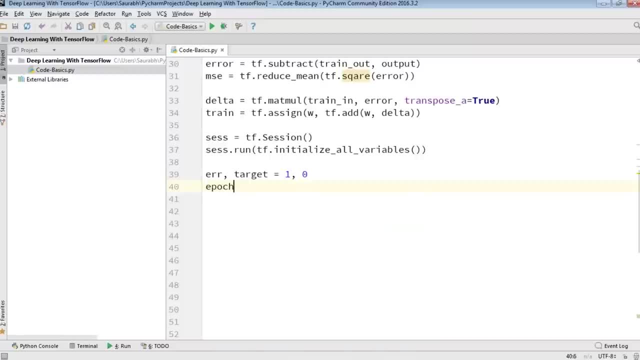 So I'm just going to define that. so I'm going to type in here a park, or you can give whatever variable name you want, And I'm going to type in here Max underscore a park Equal to 0 comma 10, which means that our it will start from the 0th a park and our maximum 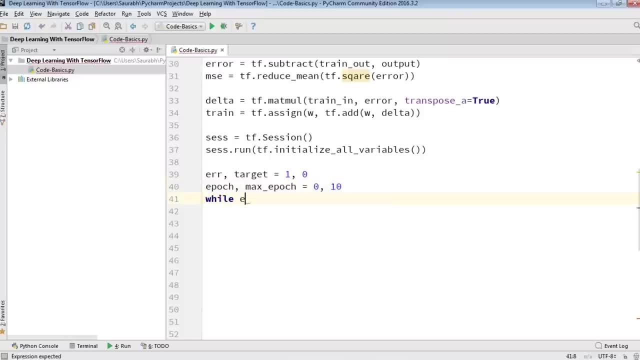 value of a park will be 10.. Now I'm going to define: while ERR should be is greater than target And a park is less than maximum a park: Increase the value of a park: Y1.. Then I'm going to type in: ERR says dot run. 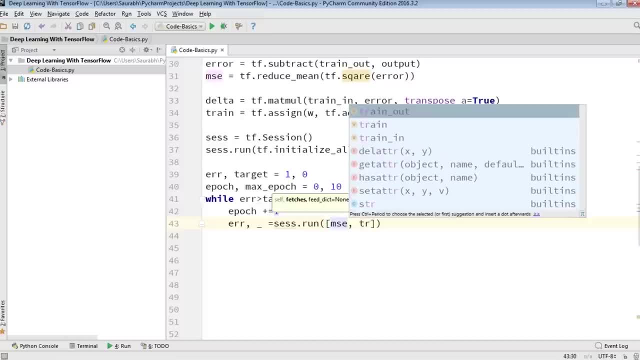 Mean squared error: comma train. And let's just finally print it and see what happens. print a park- Mean squared error, colon ERR. So basically what it will print? It will print the cycles or a park And the error with respect to that particular cycle. 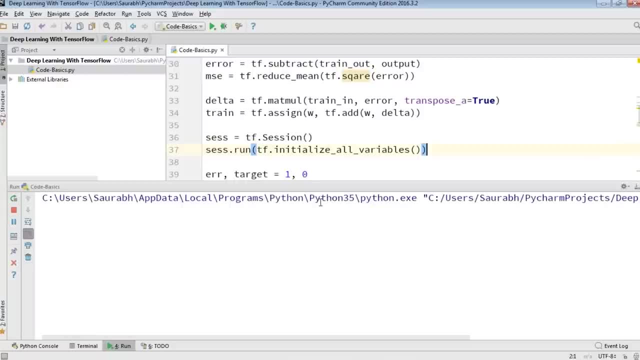 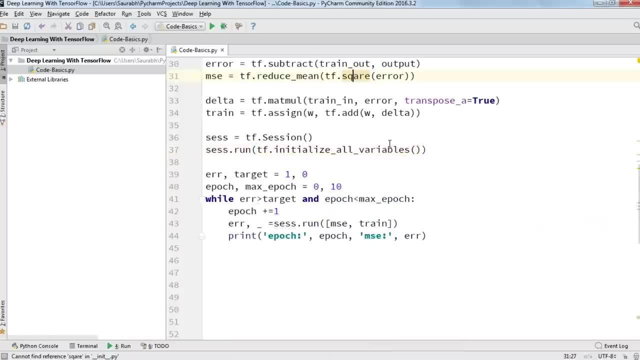 So let us go ahead and execute this and see what happens. Oops, I've typed the spelling of squared wrong. Pardon me for that. I'm just going to make it right now. SQ, you are E. All right, Let's go ahead and execute it once more. 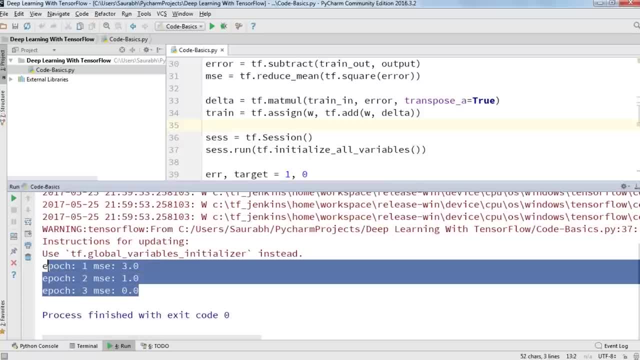 So yeah, in three epochs We got the value of mean squared error as 0. That means it took us three iterations in order to reduce the output to 0. So this is how you can actually implement a logic gate. or you can say: this is how you can actually classify the high and low outputs of a particular logic gate using single layer perceptron. 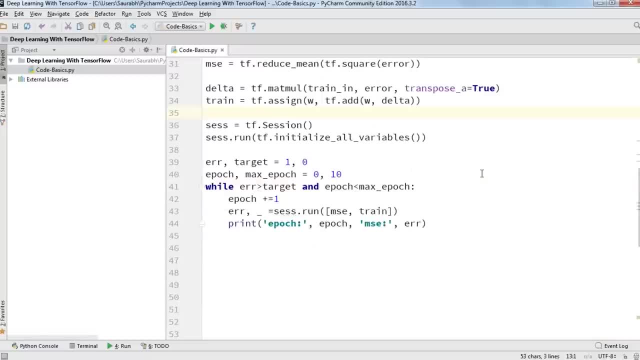 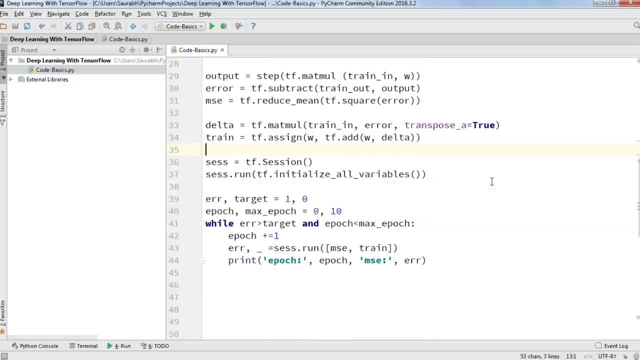 Similarly, you can do that for our gate as well. Consider this as an assignment. come up with a code that can actually classify the high and low outputs of an or gate. So any questions, any doubts, you can write it down in a chat box and I'll be happy to help you. any questions, guys? 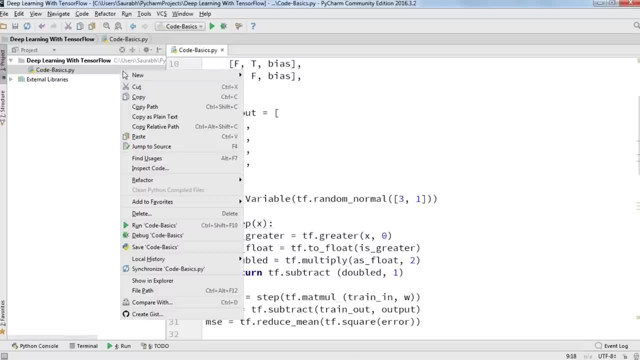 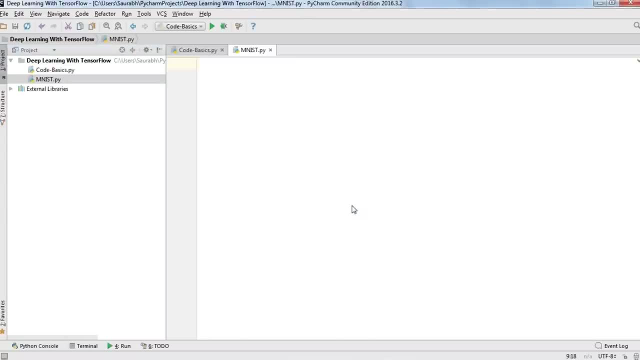 So we have no questions here, guys. So what I'm going to do, I'm going to create a new python file and I'm going to name it as MNIST, which is nothing but the data set on which we are going to perform the classification of handwritten digits. 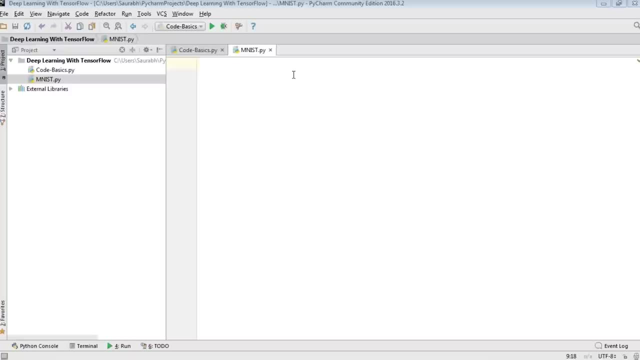 So we're going to execute a use case, and we have told you earlier as well. in this MNIST data set, We have handwritten digits between from 0 to 9, and it has 55,000 training sets as well as 10,000 test sets. 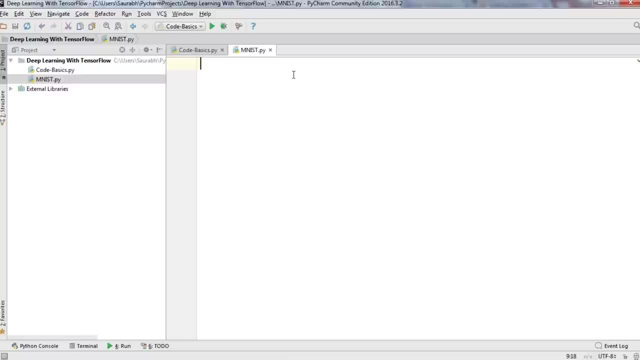 So let us go ahead with that. The first thing I'm going to do is download the data set, But before that let me just import TensorFlow library as TF. Okay, And yeah, now let us download the data set. So for that I'm going to type in from TensorFlow: dot examples, dot, tutorial, dot, MNIST. import input underscore data. 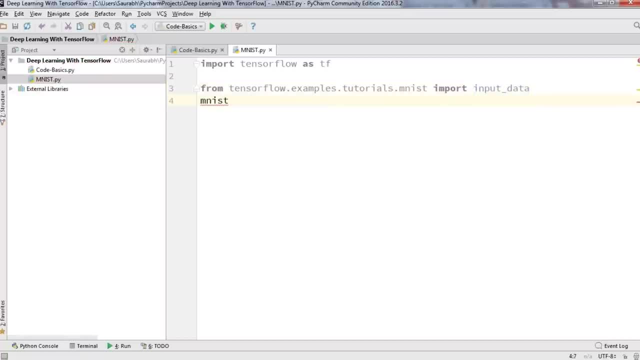 And now I'm going to type in here: MNIST is equals to input. underscore data. underscore data: dot read data sets And type in here: MNIST. underscore data: comma. one underscore hot equals to true. Now here, MNIST is nothing but a lightweight class which stores the training, validation and testing sets as a numpy array. 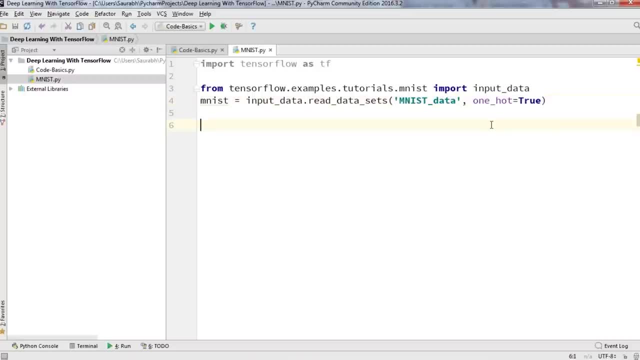 And when I talk about this, one hot equals to true, is nothing but one hot encoding. Now let me tell you what one hot encoding is. So for that, let me just comment few lines. So one hot encoding means that if I'm classifying something as a seven, 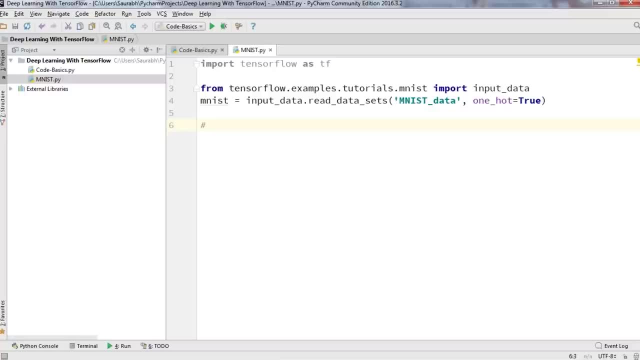 So if I classify that, my digit is seven. So how am I going to represent that? So I'm going to type in here: 0, 1, 2, 3, 4, 5, 6, 7.. The bit will be active. So I'm going to type in there one, then eight and then nine. 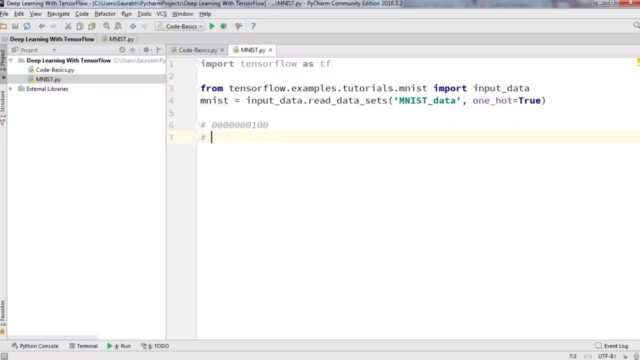 Similarly, if I want to represent, say that my digit is 2.. So I'm going to type in 0, 1.. On the second digit, I'm going to type in here as one and the rest all zeros. So I hope you got the concept of what exactly one hot encoding is. 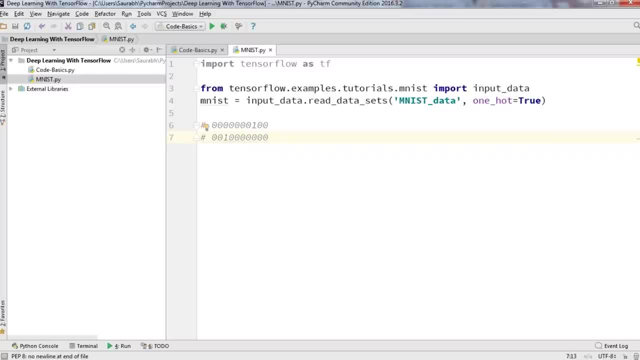 So it's like only one output is active at a time. That's all, And I'm telling it to you again and again. We are going to discuss everything in detail in upcoming sessions. So our next step is to start the session, like we do every time. 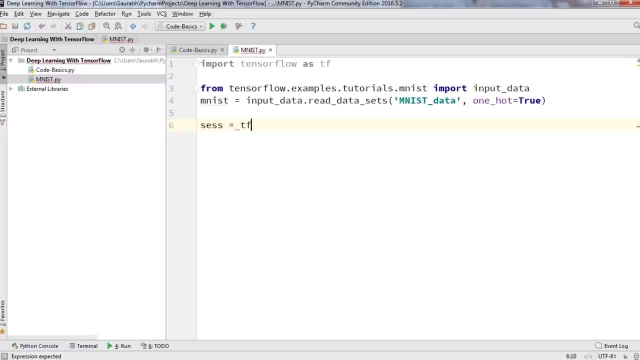 So I'm going to type in here: sets equals to TF dot interactive session. So I'm just going to type in here: Interactive session. Yeah, And now we are going to do, we're going to build the computation graph by creating nodes for the input images and target output classes. 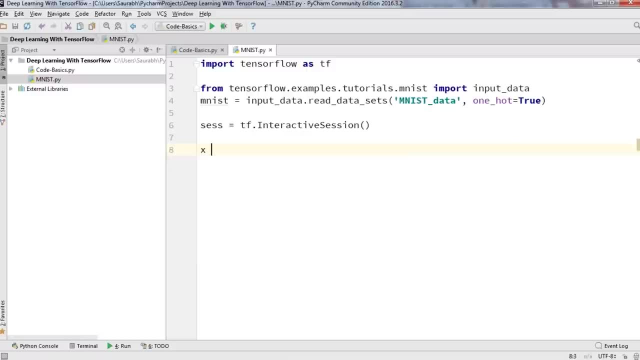 So for that I'm going to define some placeholders, For that I'm going to type in: X is equals to TF dot, placeholder TF dot, floor 32. 32. And the shape will be None comma 784.. Now the input images X will consist of 2D tensors of floating point numbers. 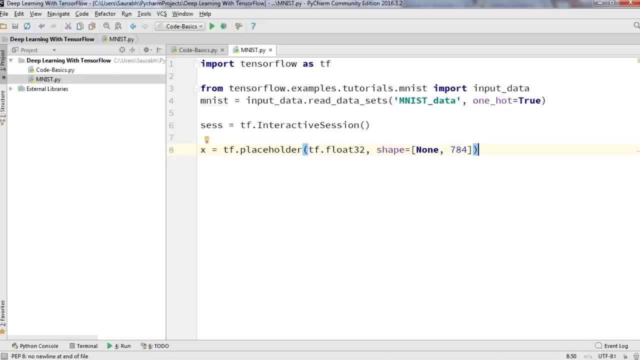 Here we assign it a shape of say none, comma 784, as you can see. So where 784 is the dimensionality of single flattened 28 by 28 pixel MNIST image of handwritten digits. And what none indicates? it indicates that the first dimension corresponding to the batch size, 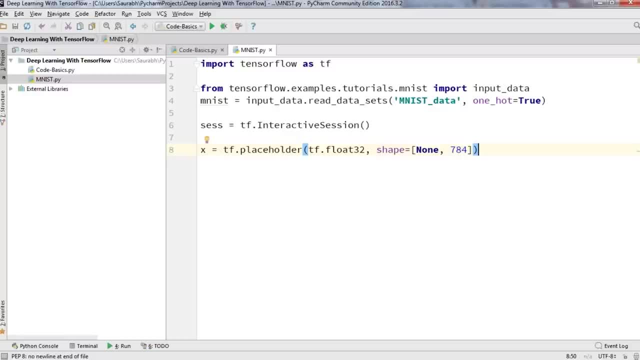 can be of any size means the first dimension can be of any size. We are not putting any restrictions on that. Now I'm going to define the variable Y, which will nothing, which will be nothing but our real labels, or you can say, the desired output placeholder. 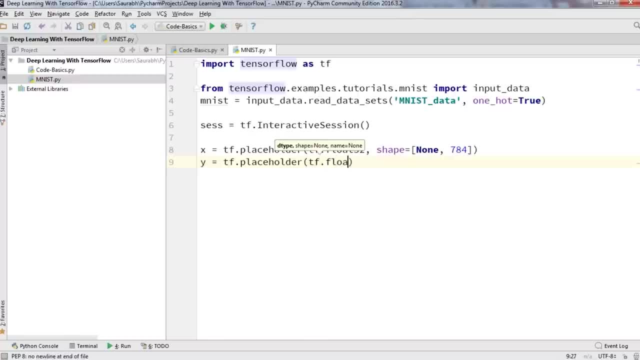 And I'm going to type in here: TF, dot, float 32.. And I'm going to define the shape, which will be none comma 10, because we have 10 classes. And similarly, Y is also a 2D array where each row is one hot 10 dimensional vector indicating which digit class. 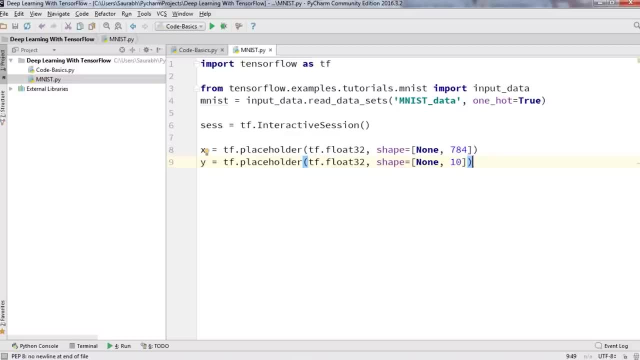 the corresponding MNIST image belongs to. And now next step is to define weight and biases for our model, like we have done in the previous example. So we could imagine treating these like additional inputs, but tensorflow has even a better way to handle them. 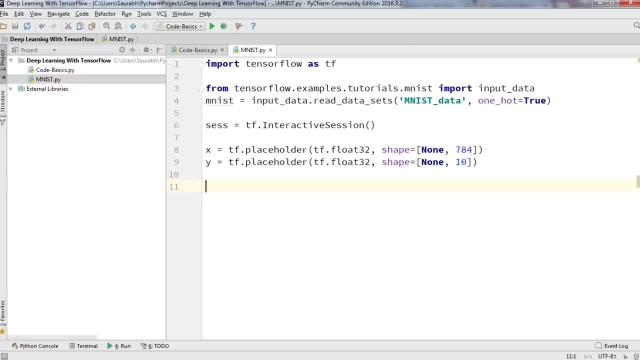 And what it is. it is nothing but variables. So let us go ahead and do that. I'm going to type in here W TF dot variable, TF dot zeros. I'm going to initialize it to zeros and the shape will be a 784 comma 10.. 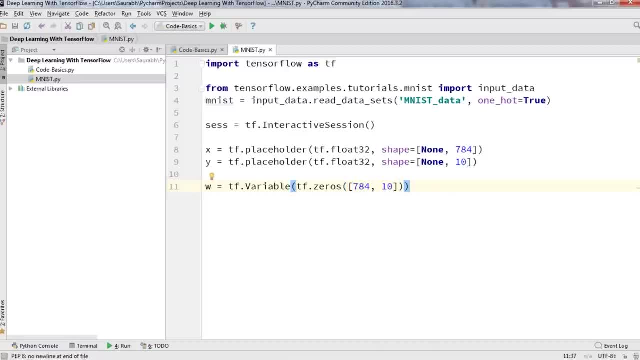 So it's like 28 cross, 28 pixels and a 10 classes. Similarly, when I talk about bias, so it will be TF dot variable, TF dot zeros. initialize it to zeros and the shape will be 10.. We pass the initial value for each parameter in the call to TF dot variable. 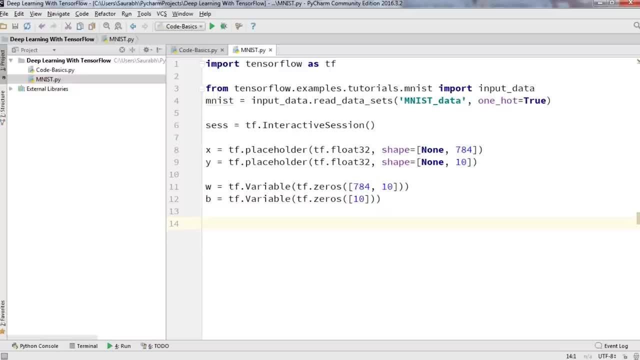 Now over here, as we can see that we initialize both W and B as tensors full of zeros, and W is a 784 cross 10 matrix because we have 784 input features and 10 outputs. And when I talk about bias B, it is a 10 dimensional vector because we have 10 classes. 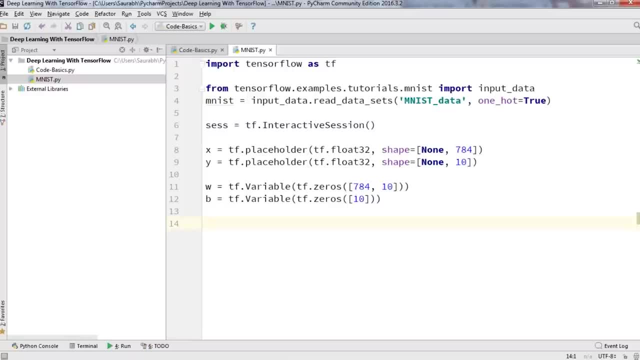 And we have learned that before we can use variables in a session, We need to first initialize it. So we're going to type it here: It says a dot run and after that I'm going to type in a TF- dot- global underscore variables- underscore initializer. 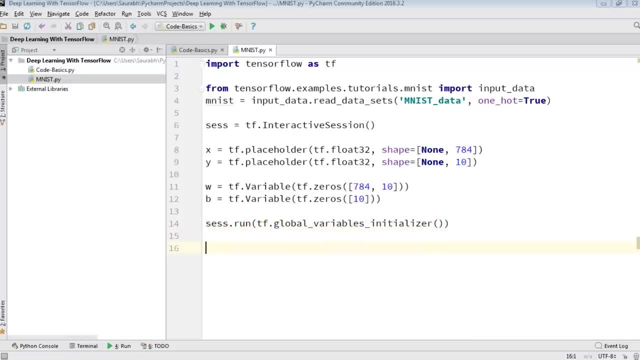 All right. so we have initialized all the variables. So our next task is to predict the class and the loss function. So we can now implement our regression model. It takes only one line. We multiply the vectorized input image X by the weight matrix W and add the bias. 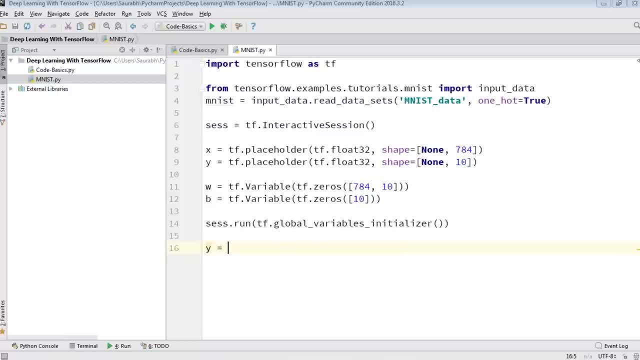 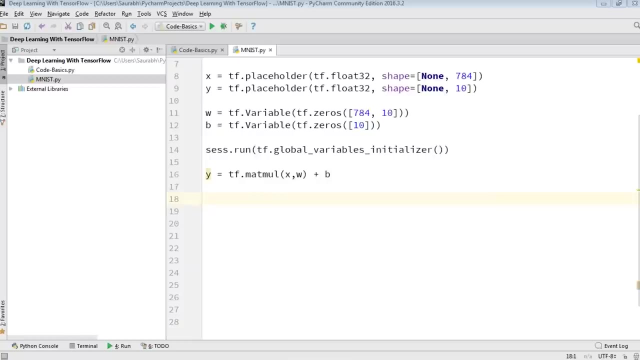 So for that I'm just going to type in here: Y equal to TF, dot matma, That is nothing but matrix multiplication X comma W plus B. All right, So now we can specify a loss function very easily. So the loss indicates how bad the models prediction was. on single example. 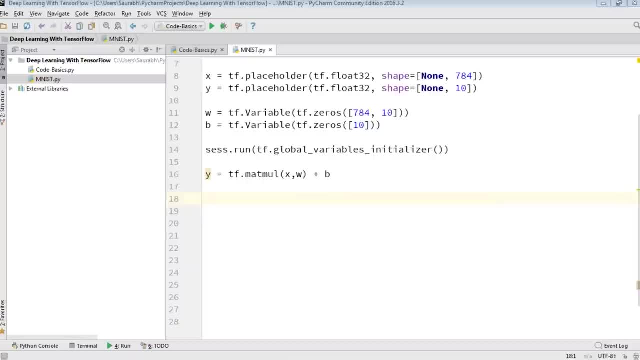 We try to minimize that while training across all the examples. So now we can specify a loss function. Now, loss indicates how bad the models prediction was on a single example And we try to minimize that while training across all the examples. Now, here our loss function will be cross entropy, or you can say the difference between the actual output and the predicted output. 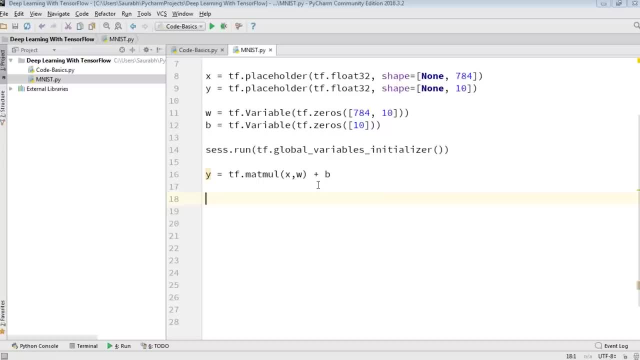 So for that, what I'm going to do, I'm going to make use of softmax cross entropy function. So here the loss will be the difference between the target output and the actual output. So for that, what I'm going to do is I'm just going to type in here a variable name. 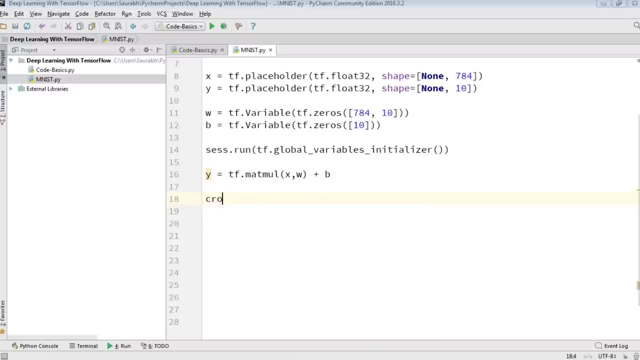 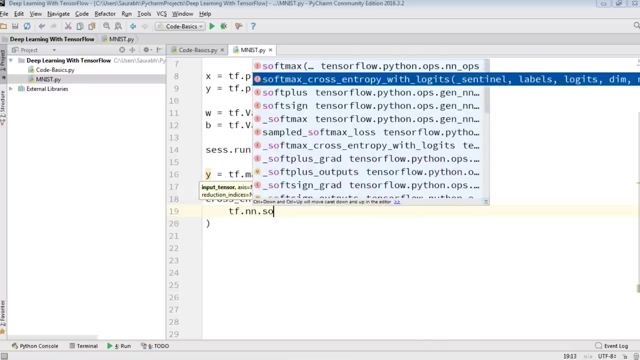 I'm going to name it as cross entropy. And yeah, entropy equals to Y, equal to TF dot W plus B, Entropy equals to TF dot reduce, underscore mean. And then just type in here. Let me just enter the next line: TF dot, NN, dot, softmax, underscore, cross entropy with logits. 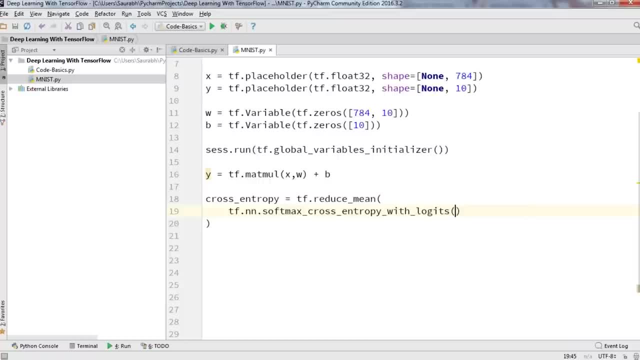 And now over here, I'm going to type in first our target output, which will be labels, equals to Y comma. our actual output, So it'll be logits, is equals to Y. That's all So over here. let me just give you a brief idea of what is happening. 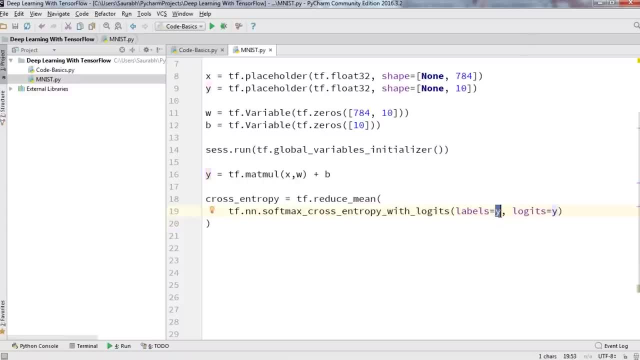 So labels is equals to Y means that this is our target output and this is the actual output. So it will be. will name it as Y underscore, And so what exactly is happening? It will calculate the difference between the target output and for the actual output. for all the examples: 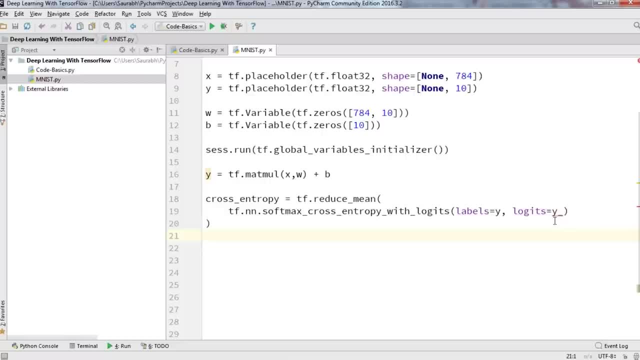 Then it is going to sum all of them and then find out the mean. So this is what, basically, this cross entropy variable will do, Now that we have defined our model and training loss function. it is straightforward to train using this, So we're going to train using TensorFlow. 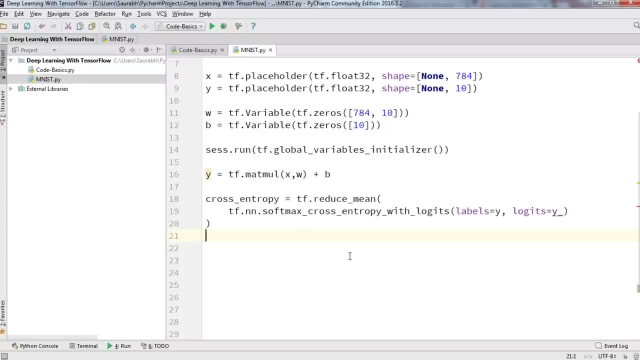 Now we need to train our model, So TensorFlow has a wide variety of built-in optimization algorithms, as I've told you earlier as well, And for this example, we'll use steepest gradient descent with a length of about 0.5 to descend the cross entropy. 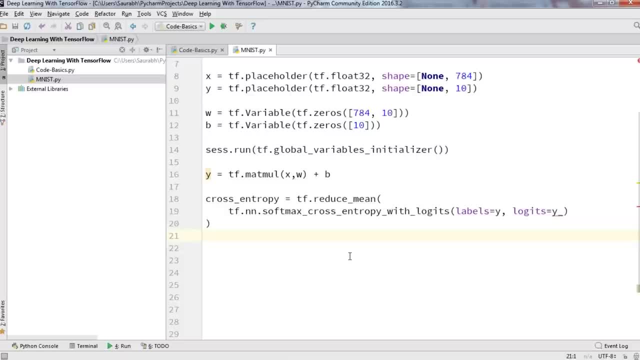 So basically we're going to use a 0.5 learning rate or you can say the step length. So for that I'm going to type in here: train underscore. step equals to TF, dot, train Dot, Gradient descent optimizer and the step will be 0.5 and minimize the loss. 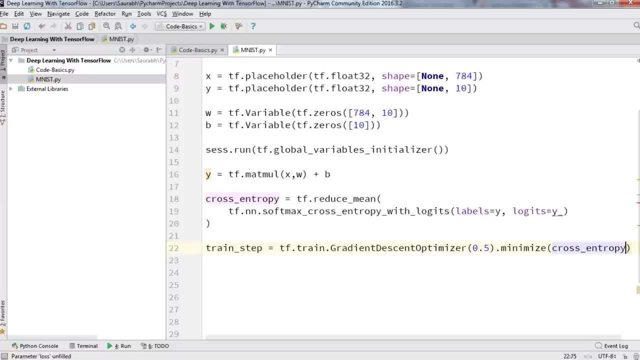 So minimize cross entropy, That's it. So what this one line basically will do, it will minimize the cross entropy, which is nothing but the loss function that we have defined. Now, in the next step, what we are going to do, we are going to load hundred training examples in each training iteration. 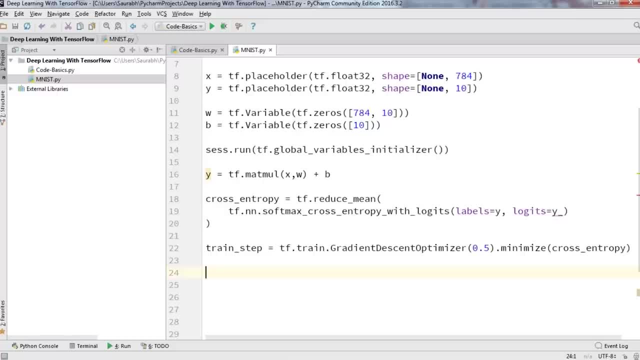 So each time the training iteration happens, it will take hundred examples. We then run the train underscore step Operation, which is nothing, but to reduce the error using feed underscore dict, which is nothing, but we are going to feed the real values to our placeholder Y. 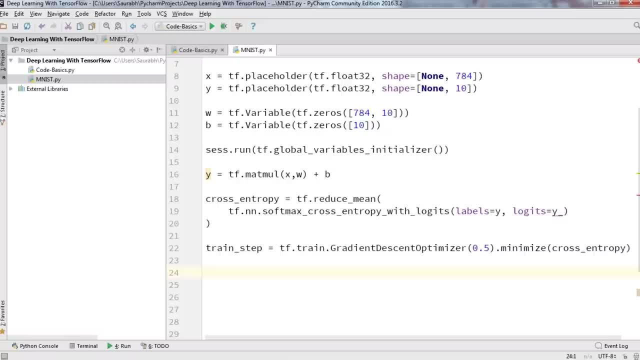 Now, next, what we are going to do. we're going to load a hundred training examples in each training iterations, which means that for each iteration will take hundred training examples and will run the train underscore step operation, which is nothing but the optimizer here. 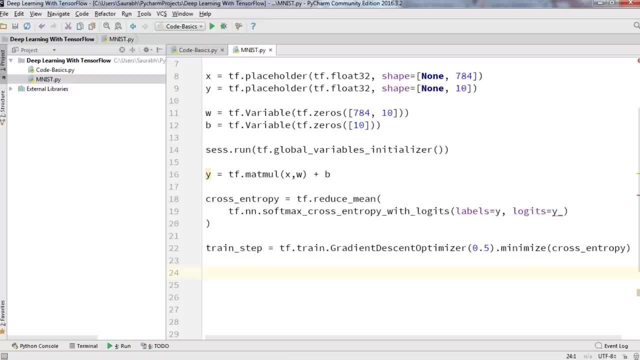 And after that we're going to use a feed underscore dict to replace the placeholder tensors X and Y with the training examples. So basically, X will contain the input images and Y will contain the actual outputs, or you can say the desired outputs. 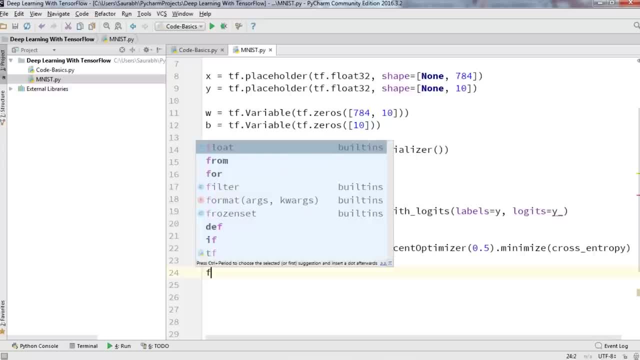 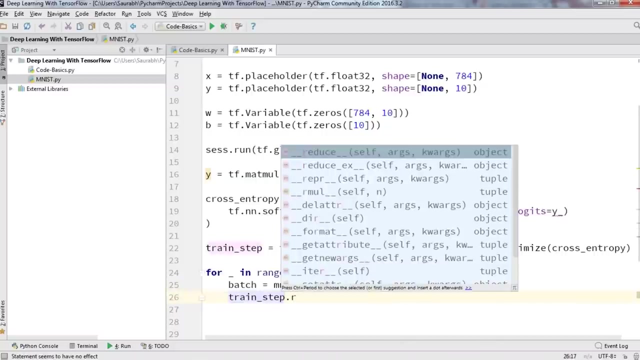 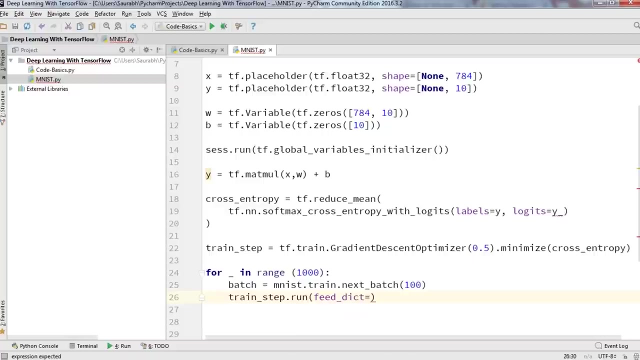 For that I'm going to type in here for underscore in range: thousand batch equals to MNIST dot, train dot. next underscore batch: hundred train. underscore step dot run. And I'm going to feed in the values, The values to X and Y variable feed underscore dict equal to X colon batch zero comma. Y colon batch one. 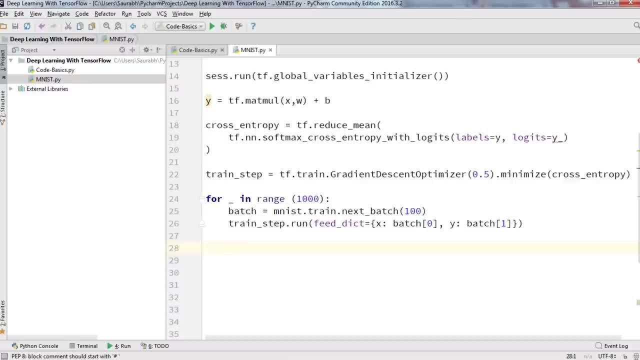 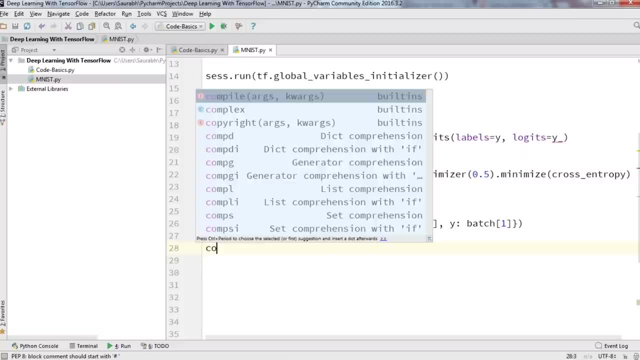 That's it. Now we need to evaluate our model. We need to figure out how well our model is doing, And for that I'm going to make use of TF dot argmax function. Now, this TF dot argmax function, let me tell you how it works. 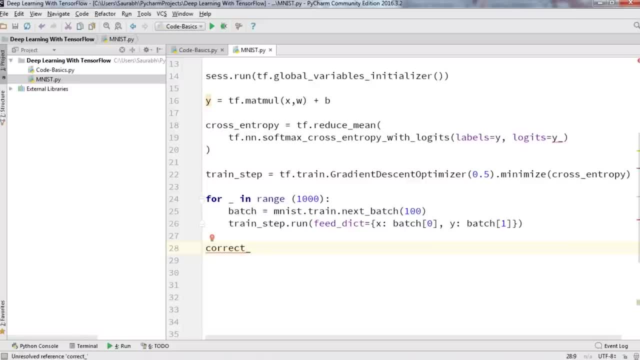 First correct underscore prediction equals to: TF dot. equal TF dot argmax Y underscore comma one, comma TF dot argmax Y, comma one. So basically this TF dot argmax Y underscore comma one is a label Our model thinks is most likely for each input. 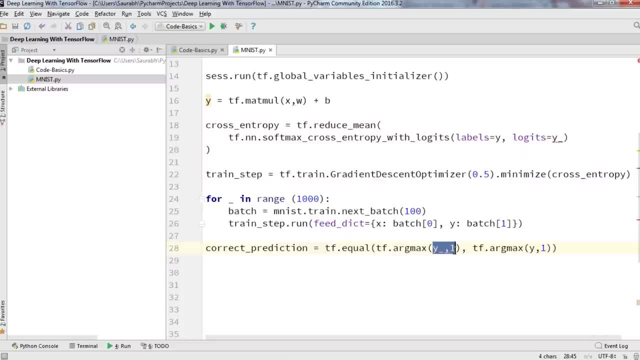 That means it is a predicted value, While TF dot argmax Y, comma one is a true label. It is there in our data set present already, and we know that it is true. So what we are doing, we're using TF dot equal function to check if our actual prediction matches the desired prediction. 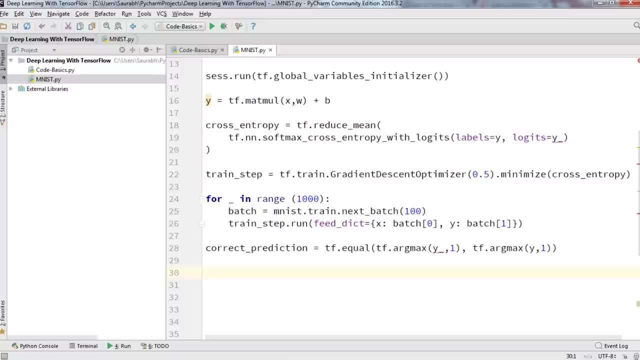 This is how it is working. So now, what we're going to do? we're going to calculate the accuracy to determine what fraction are correct. We cast a floating point numbers and then take the mean. So now I'm going to define a variable for accuracy. 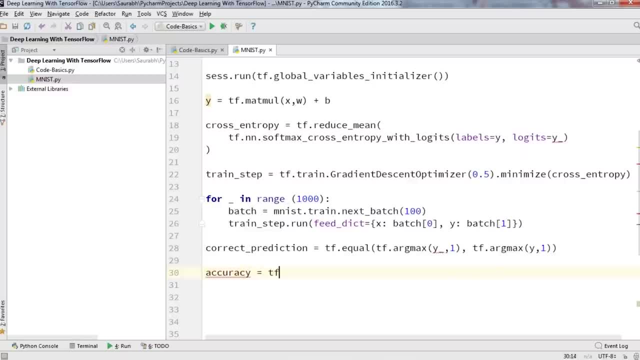 So I'm just going to type in: accuracy equals to: TF dot reduce underscore mean: TF dot cast correct underscore prediction comma: TF dot float 32.. And what we can do? finally, we can evaluate our accuracy on the test data, And this should give us accuracy of about 90%. 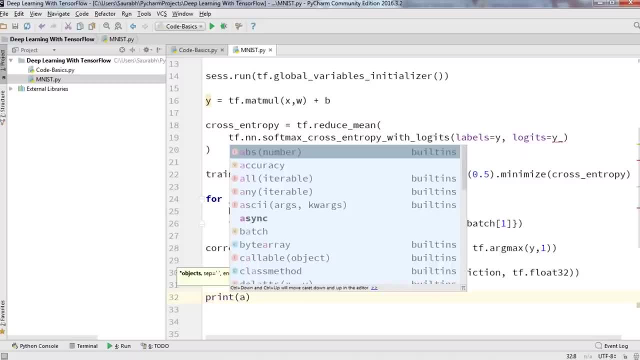 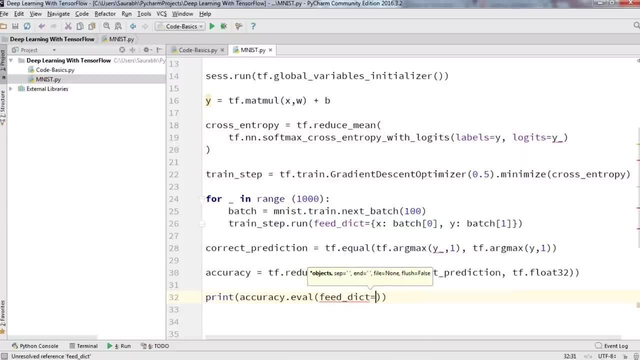 So let us see if that happens. I'm going to type in here: print accuracy dot- evaluate eval feed. underscore dict equal to X colon mnist dot- test dot. images comma Y colon mnist dot- test dot labels. That's it, guys, And I've done a mistake here. 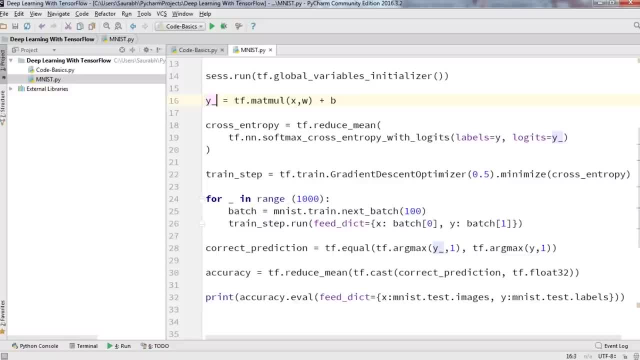 So instead of Y, it will be Y underscore, because this is our predicted value, not the actual value, and why we have considered as actual value And this Y underscore will be our predicted values. This is the mistake that I made, So yeah, 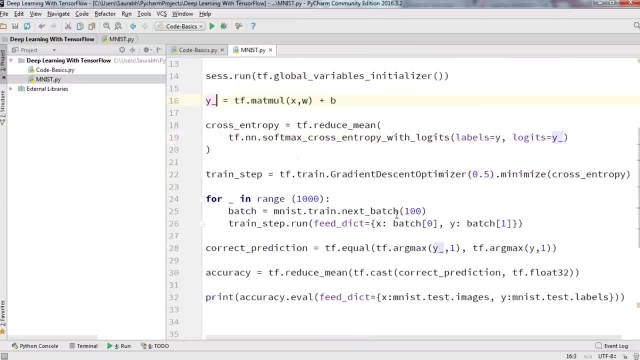 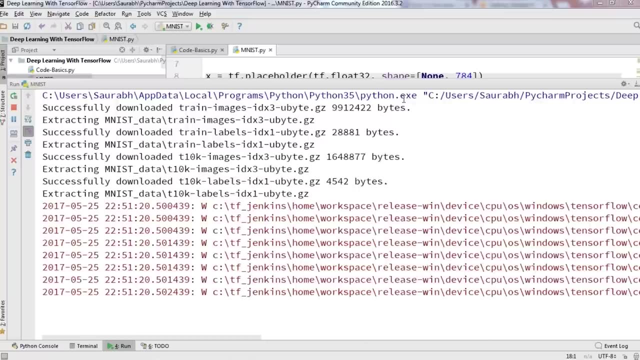 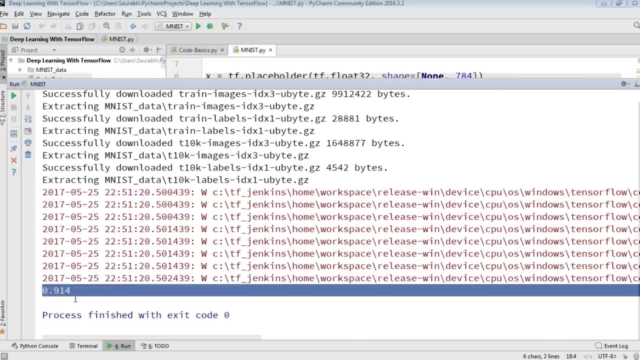 now I think the code looks pretty fine to me and we can go ahead and run this. Let us see what happens when we run this. So, guys, it is complete now, And this is the accuracy of a model which is 91.4%, and which is pretty bad when you talk about a data set like mnist. 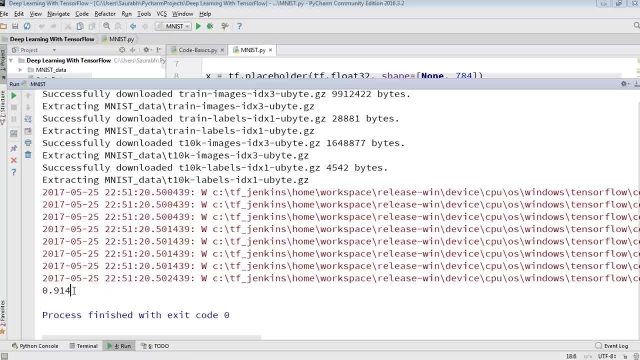 But yeah, with a single layer, which is very, very good. So we have got an accuracy of around 92% on the mnist data set, which means that whatever the test data sets were there, that is like 10,000 test images. 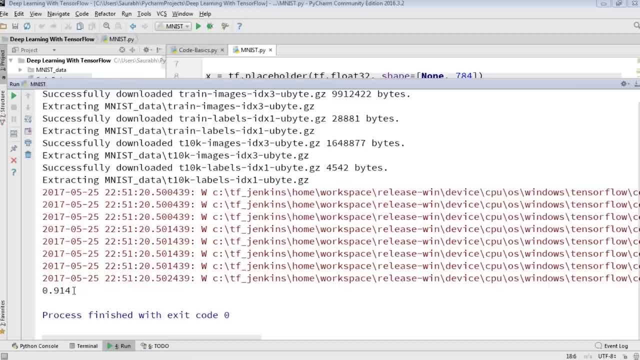 So on those test images, whatever the prediction our model has made, are 91.4% correct. So, guys, let me just give you a quick recap of all the things we have discussed. So first we saw what exactly is deep learning and how it is different from the traditional machine learning. 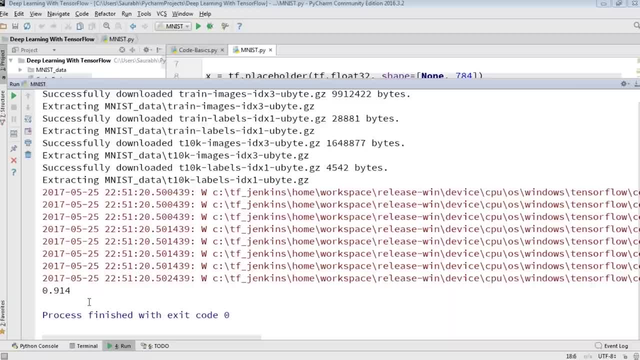 Then we understood the motivation behind deep learning, which is nothing but your brain cells, which are called neuron. Then we understood the importance of why we need artificial neurons. And then we took the example of artificial neuron which is called a perceptron. 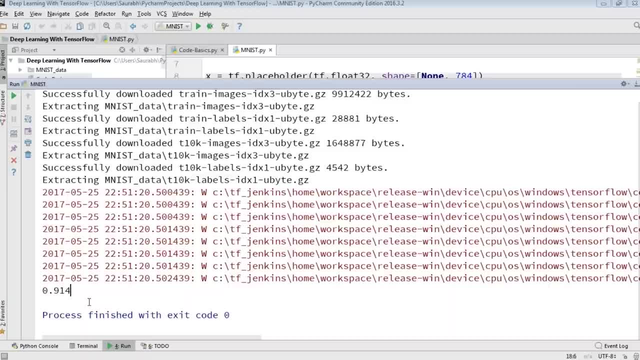 And we looked at a couple of examples in which we implemented the AND gate. We performed image classification on the mnist data sets, which is nothing but handwritten images between 0 to 9.. And we also implemented a couple of examples in order to 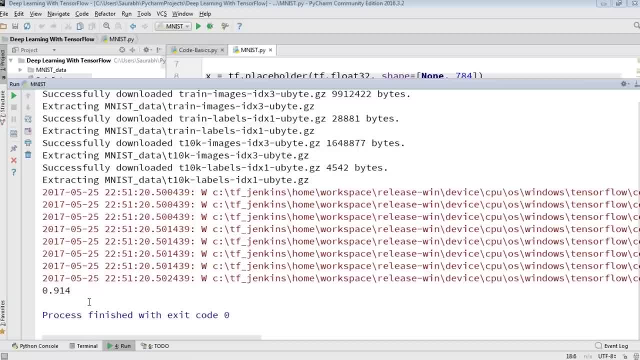 understand what are placeholders, variables and constants. So till now, guys, any questions, any doubts? you can write it down in your chat box Any questions? So we have a question from Imran and he's asking: why is the desired output and why underscore is the actual output? 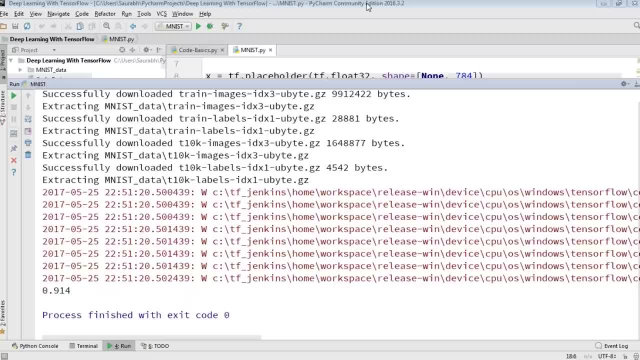 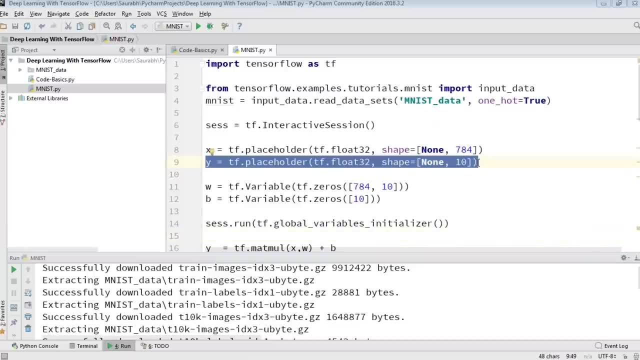 which is exactly correct, Imran. This is how the case is. Let me just explain it to you with the code as well. Yeah, this is our why, which is nothing but the classes, the 10 classes which are already defined, or, you can say, the desired output. 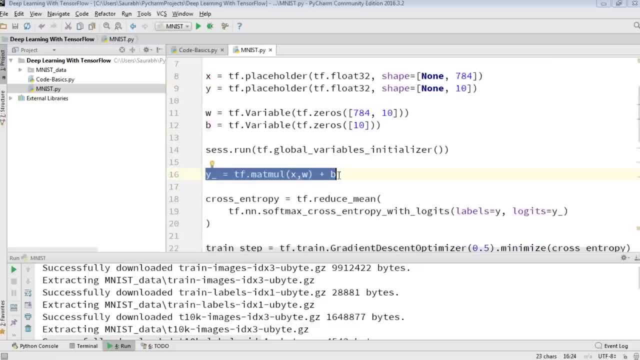 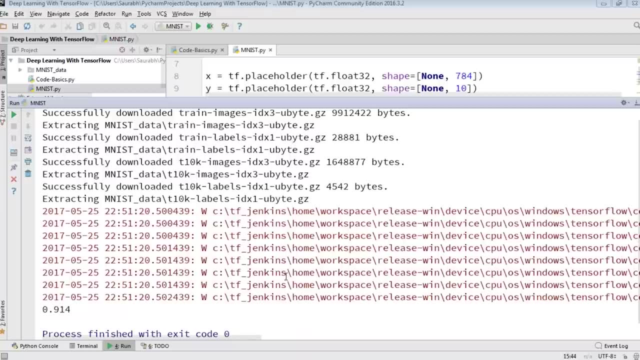 And this is our why underscore, which is the predicted output. So I hope this answers your question. All right, he's pretty fine with it. Any other questions, any other doubts, guys, you can write it down in your chat box. I'll be happy to help you find no questions. 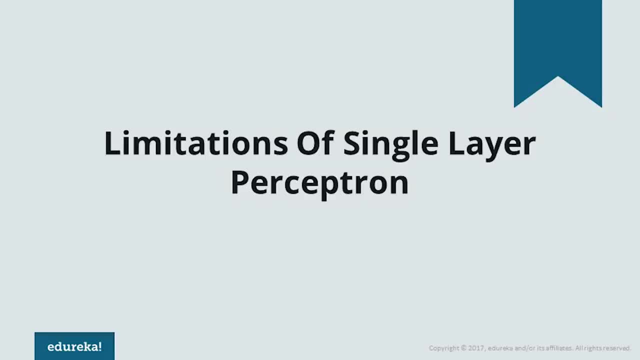 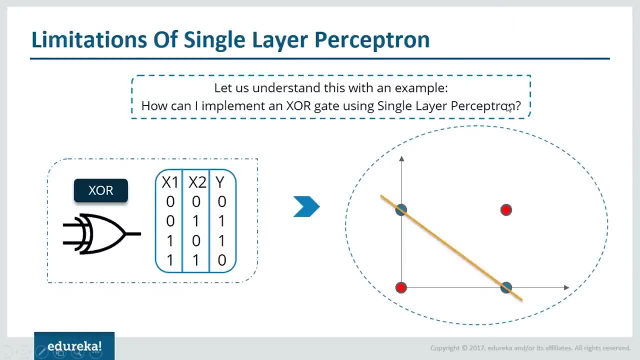 We'll move forward with the slides. So now there are certain limitations of single layer perceptron. Let us understand that. So, in order to understand that, we'll take an example. And yeah, if I can recall somebody asked that question: how can we implement XOR gate using single layer perceptron? 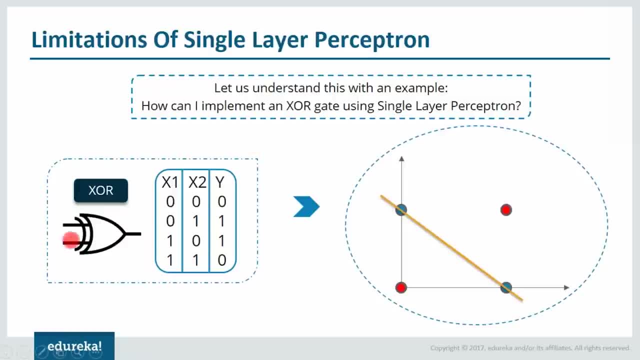 So let us see if we can do that or not. So we have an XOR gate here and this is a truth table. So according to this truth table, if any one of the input is high, then the output is high, And if both the inputs are low, 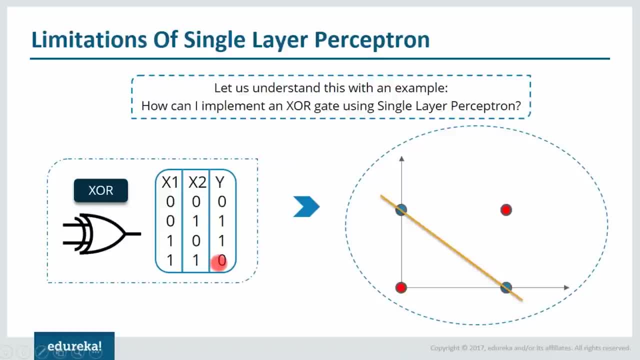 output is low, And if both the inputs are high, output is low. So how can you classify the high and the low outputs with a single line? Definitely you can't, If you see the points. so one point is here, one is here. 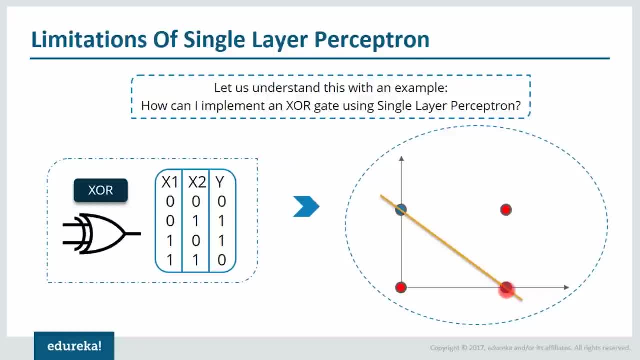 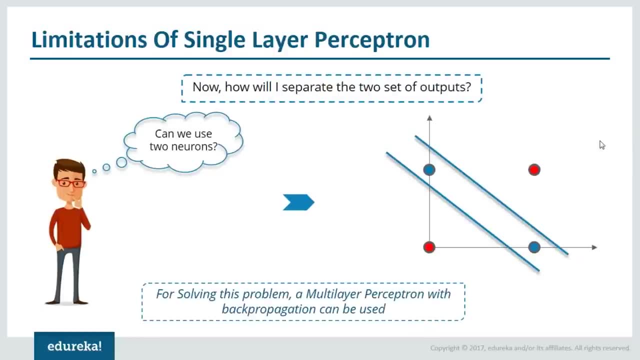 here and here, in which these two points are high outputs and these two are low. So how can you classify with a single line? Definitely you can't. So now, what's the answer to this? What if we use multiple neurons? Using multiple neurons? 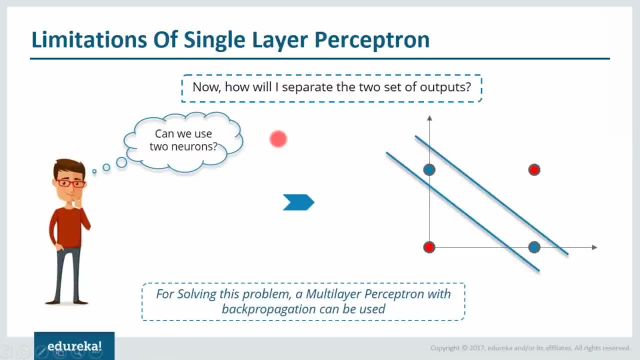 we can have two lines that can separate it. Now we can solve this problem if we have multiple neurons. So if we use two neurons, we can have two lines and that can actually separate the high outputs as well as the low outputs. So this is where we use multilayer perceptron with back propagation. 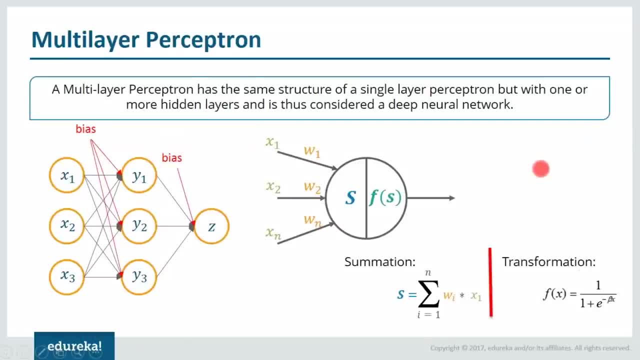 So what are multilayer perceptron? Multilayer perceptrons? they have the same structure like the single layer perceptron. The only difference is that they have more than one hidden layer. So let me explain it to you with an example. 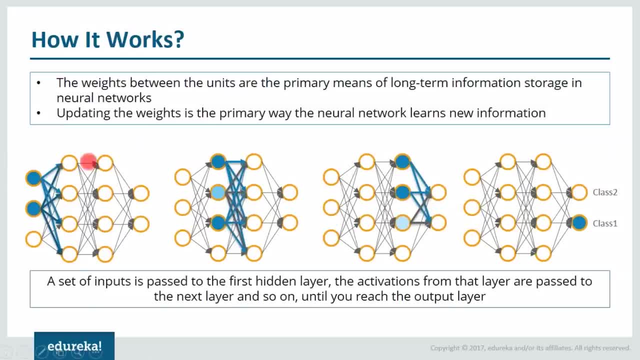 So this is how a typical multilayer perceptron looks like. So we have input layer, we have two hidden layers and we have one output layer as well. Now, typically, each of these input layers are connected to the next hidden layer. Each neuron is connected to the next neuron present at the adjacent layer. 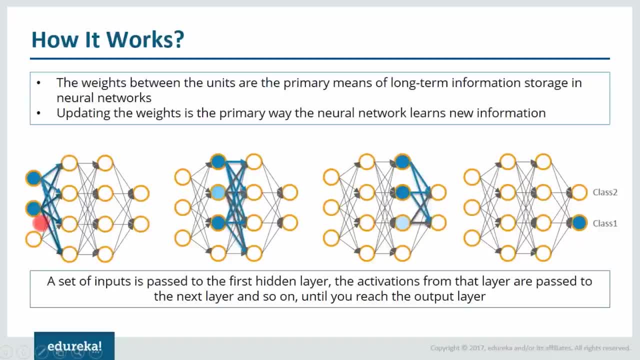 But the neurons of the same layer are not connected to each other. Now what happens? A set of inputs are passed to these input layers and the output of this input layer will be passed to the first hidden layer. Then, after activation, function of the first hidden layer. 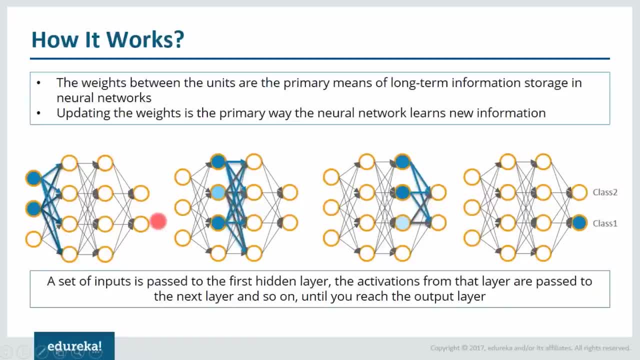 the output will be passed to the next hidden layer as the input and similarly, finally, we get the output. Now you must be thinking how the model learns from here. So, basically, the model learns by updating the weights, and the algorithm that it uses is called back propagation. 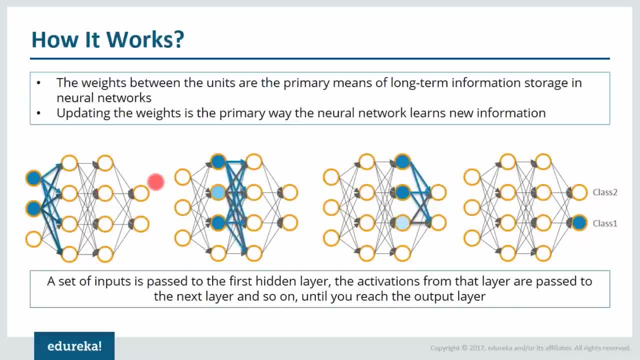 So the back propagation algorithm helps the model to learn and update the weights in order to increase the efficiency. So, basically, this process from input layer to the output layer is called a feed forward process And then, when we back, propagate it in order to increase the efficiency. 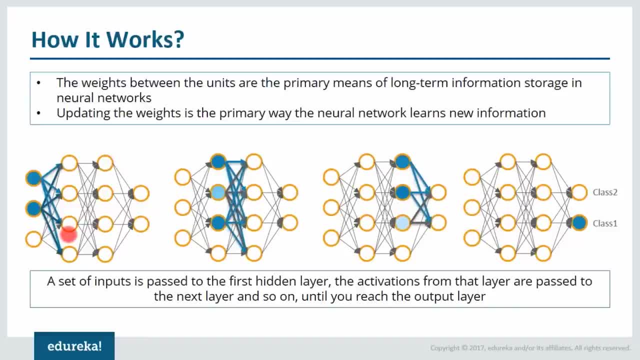 or accuracy, so that we can update the weights. that is called as a back propagation. We'll understand back propagation in more detail. So any questions, guys, apart from this? Fine, so we have no questions. So let us move forward and understand what exactly is back propagation. 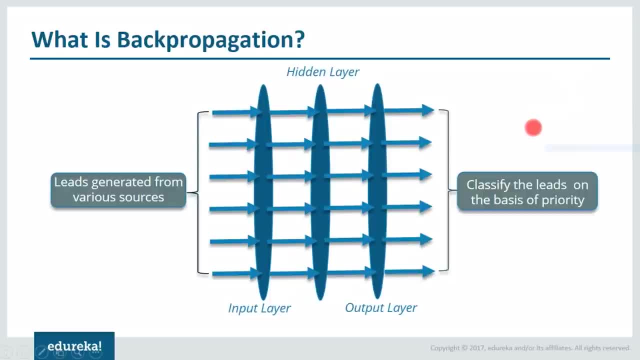 So what is back propagation? Now let us understand this with an example. So we'll take the inputs as the leads generated from various sources, And my aim is to classify the leads on the basis of the priority, So there might be certain leads which won't make it that much difference. 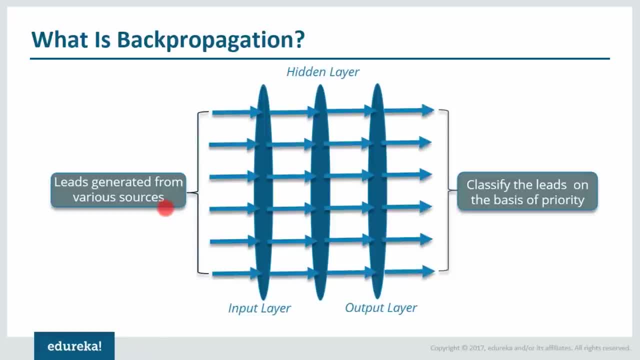 to me, whereas compared to the other leads. So in that case, I need to make sure the leads which are important gets the highest amount of weight. How am I going to do that? First we'll see the output, then, accordingly, we'll calculate the error. 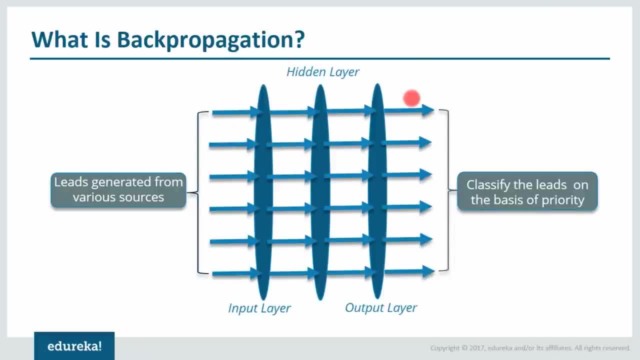 and, based on that error, we are going to update the weight, And this process is nothing but your back propagation. in a nutshell, I can say: right, Although the algorithm is pretty complex, but yeah, this is basically what happens. So, in order to classify the leads in the basis of priorities, 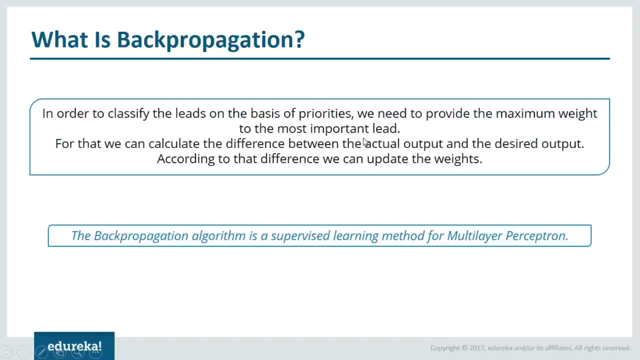 we need to provide the maximum weight to the most important lead. And how are we going to do that? We're going to compare the actual output and the desired output and, according to the difference, we're going to update the weights. So what is back propagation? 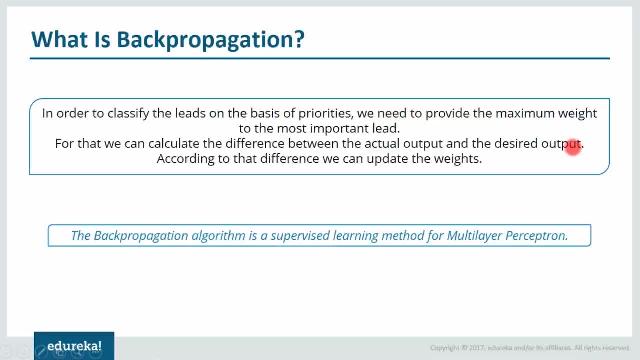 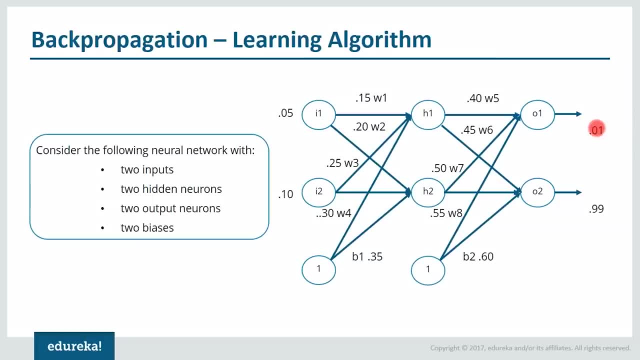 So back propagation is nothing but a supervised learning algorithm for multi-layer perceptron. Now let us understand what exactly is this algorithm. Let us understand this with an example that is there in front of your screen. So these two are our input neurons, these two are our hidden neurons. 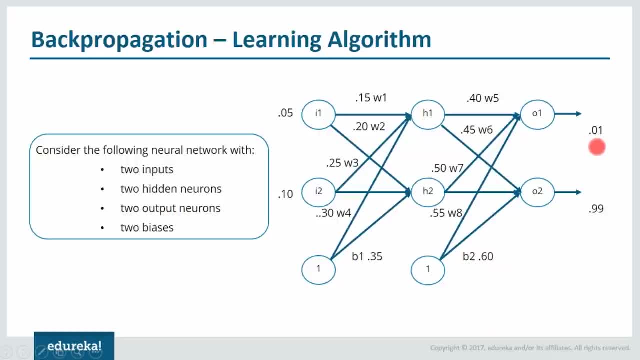 and these two are our output neurons. Now our aim is to get 0.01 and 0.99 as our output and at the same time we have inputs as 0.05 and 0.10.. Initially, we take the weights as we can see it here. 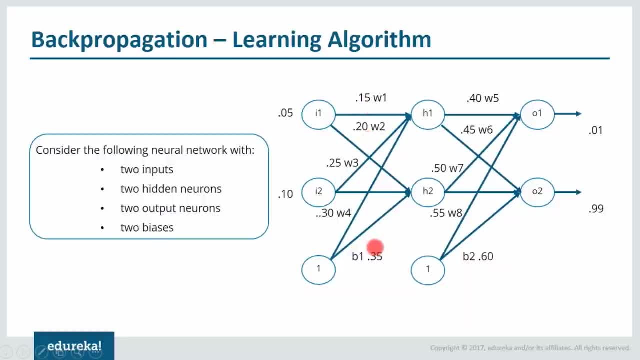 So 0.15w1, 0.20w2.. So these are the weights, Plus we have two biases as well. Now what we need to do is we need to make sure that we have weights in such a way that we get output as 0.01 and 0.99.. 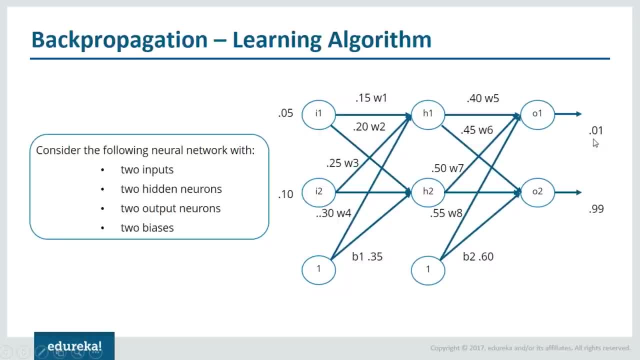 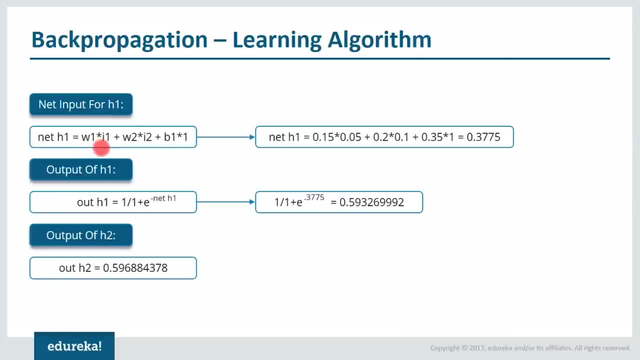 But let us see if we get that same output. when we provide these kind of weights, The net input for this particular h1 will be what It will be: w1 into i1. that is the first input. plus w2 into i2, plus b1 into 1. 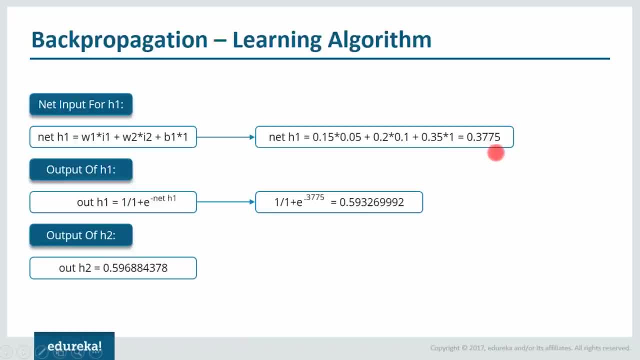 which gives us the answer as 0.3775.. Similarly, the output for h1 will be nothing but the activation function, the output after the activation function, And we are using here sigmoid function, because our brain also uses a sigmoid function. that is what we believe in. 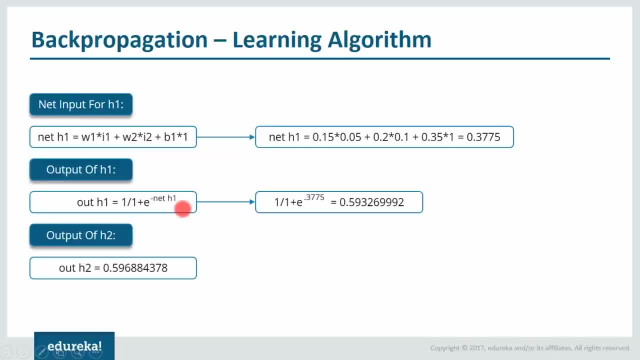 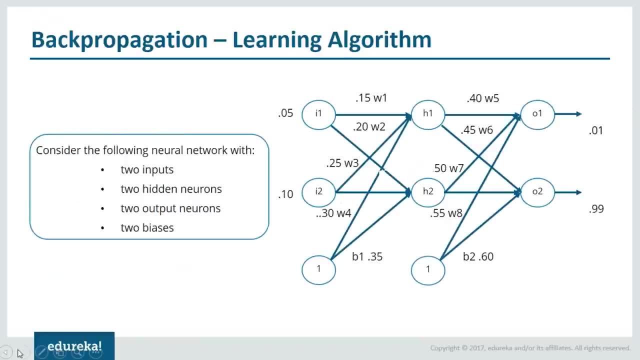 And at the same time it is easily differentiable. and if you differentiate it like this, if you do it twice, you get the same number. So the output of h1 will be 0.59 something. So let me go back. So the output of this particular h1 will be 0.59 something. 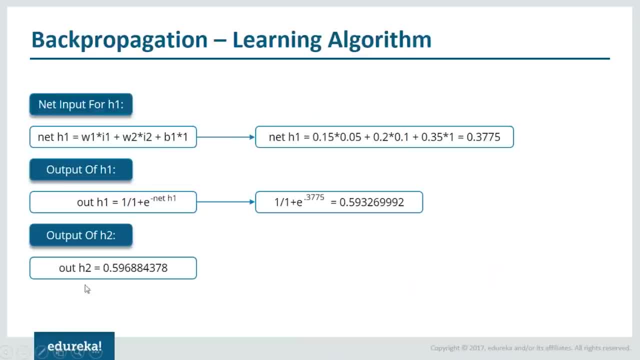 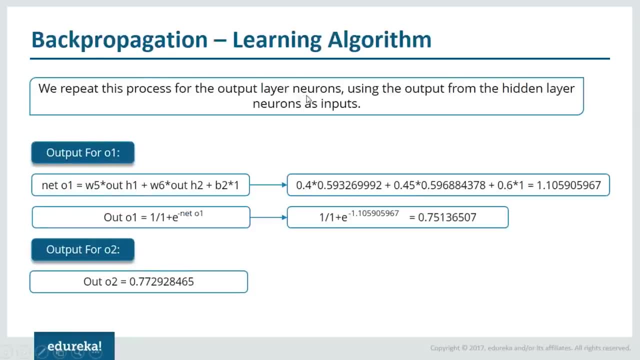 Then we are going to calculate the output of h2 as well, similarly, And we get the output as 0.596884378.. Next up, we are going to repeat the process for the output layer neurons as well. So for the output layer, the net input. 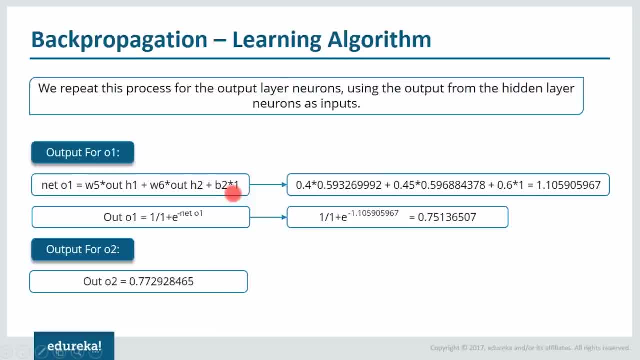 will be w5 into out of h1, w6 into out of h2 plus b2. that is the bias, So we get the output somewhere like this, And then the net output for out o1 will be after the activation function, which will be 0.751.. 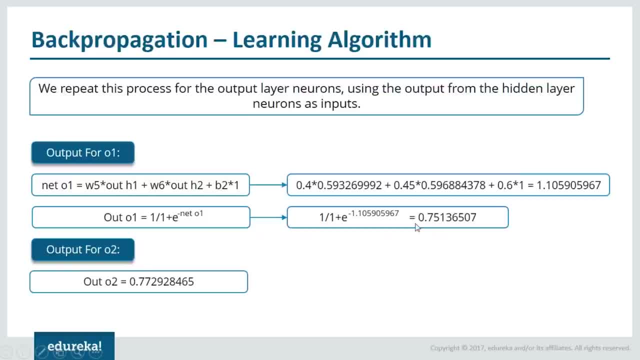 Similarly, the output for o2 will be 0.77.. Now, if you notice that this is not the desired output, Our desired output was 0.01 and 0.99.. What we got instead? we got 0.75 and 0.77.. 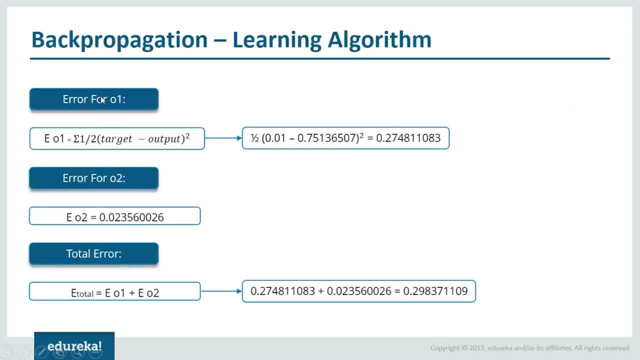 So what we need to do, we need to update the weight. So for that we are going to calculate the error Now. error for output: o1 is nothing but the sigma of 1 by 2. target minus output. whole square Target is nothing but your desired output. 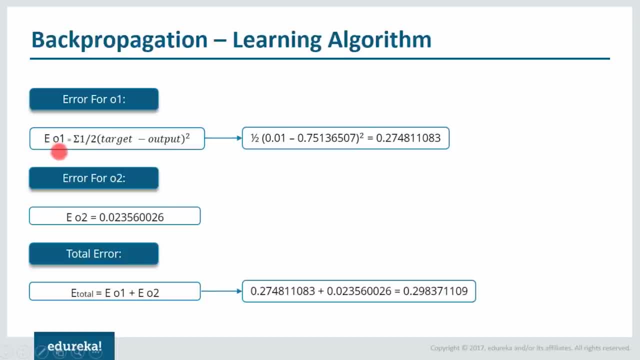 and output is your actual output. So your error of output of o1 neuron will be 0.278.. Similarly, for o2 will be 0.023.. So the total error comes down to 0.29. something Next up. we need to update the weight. 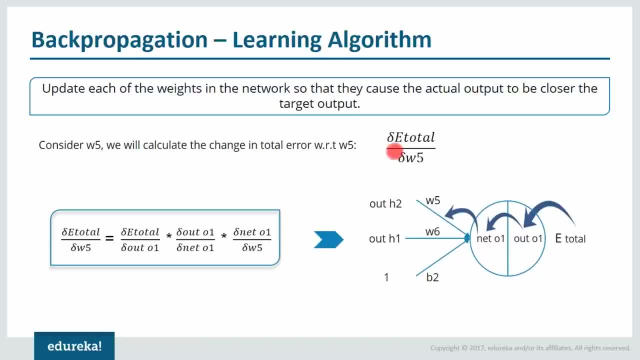 so as to decrease this error. Now, what we got to do? we got to first calculate the change in total error with respect to any of the random weight. we'll take w5, for example, Just to show you. so we're going to calculate the change in the total error when we change. 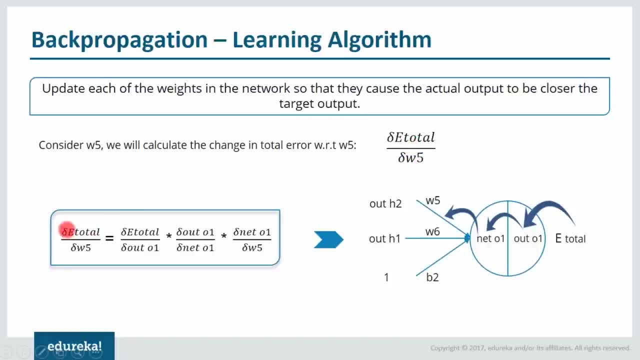 with respect to the weight w5.. So we're going to apply a chain rule here. So using partial derivative, We're going to calculate e total by delta of out o1 into delta of out o1 by delta of net o1, and then delta of net o1 by delta of w5. 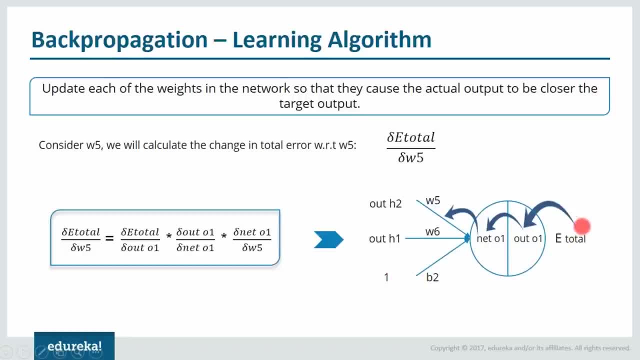 as you can see it from this particular example as well: E total, change in e total with respect to out o1, change in out o1 with respect to net o1 and change in net o1 with respect to w5.. We're going to multiply that and we're going to get this. 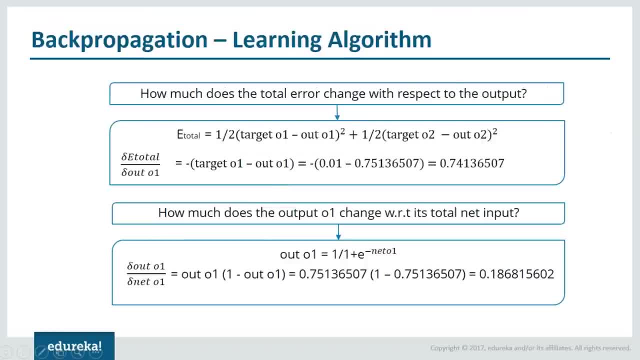 particular term and let us see how we do that. So how much the total error change with respect to the output, e total by e out o1.. We're going to calculate it. It came around 0.741.. Similarly, we're going to calculate how much does. 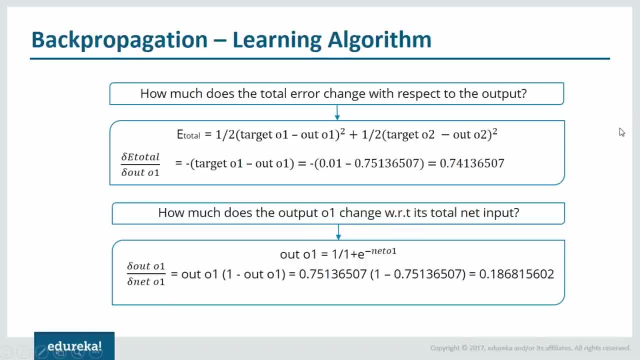 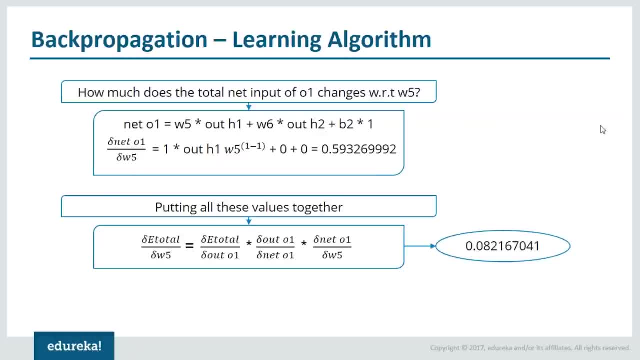 the output, o1 change with respect to the net output, and we get this. after that we're going to calculate it for net output change with respect to w5 also. We got this and then, finally, what we did: we put all these values together and we found out. 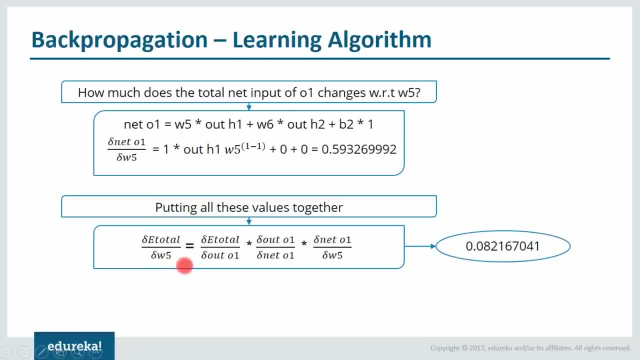 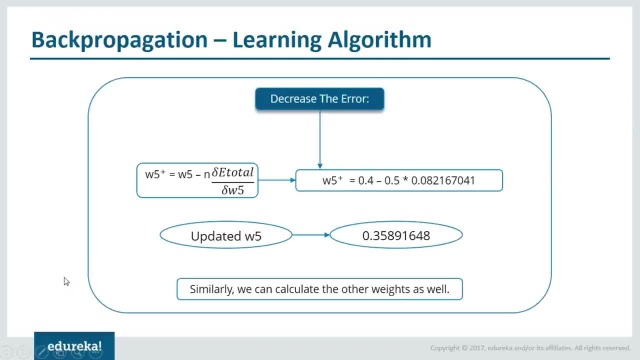 the change in the error with respect to the change in weight w5, which came to around 0.082167041.. Now is the time to update the weight. So how are we going to update the weight? First thing we need to do is we need to follow this formula. 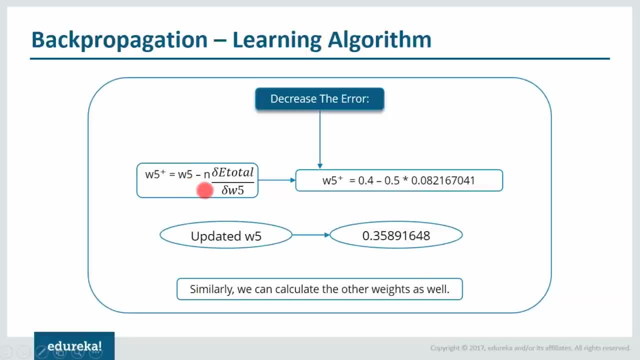 So w5 plus is nothing but the updated weight, which is equal to w5, minus the learning rate into delta of e, total by delta of w5. So which came to around 0.35891648.. Similarly, we can calculate the other weights as well. 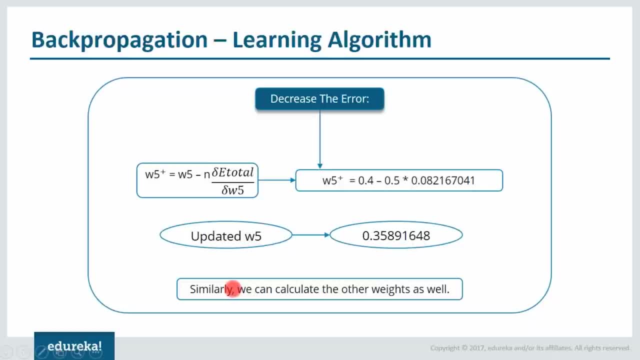 So we're going to repeat the same process and we're going to calculate the other weights as well. Then again we're going to see how much is the loss. If still the loss prevails, then we're going to repeat the same back propagation learning algorithm again. 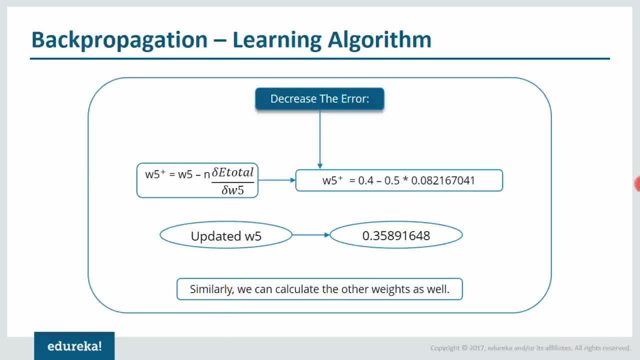 for all the weights. So this process will keep on repeating. So this is how back propagation actually works. So we'll actually have a separate module in which we'll discuss back propagation in much more detail. So now what I'm going to do: I'm going to make use. 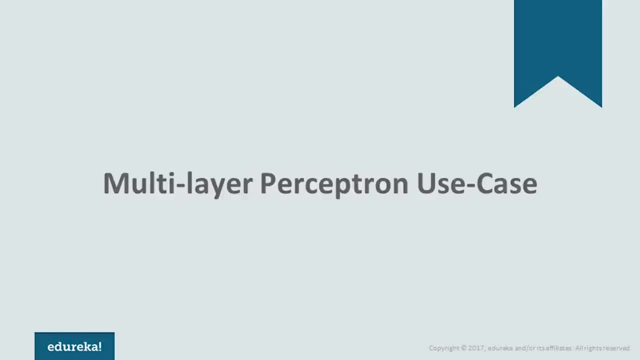 of the same MNIST data set and I'm going to increase the efficiency of that data set by 97 to 99% with the help of multi-layer perceptron. So, guys, let us go ahead with that. So guys, as I've told you earlier, is where we are going. 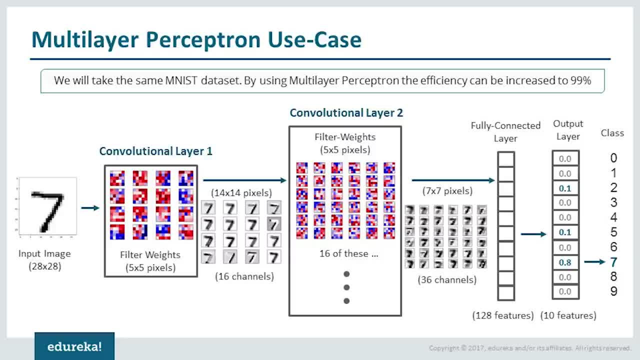 to use the same MNIST data set which we have used in the single layer perceptron. So I'm going to perform a classification using multi-layer convolutional networks. Now, what are convolutional networks? Basically, these networks are used in order to classify images. 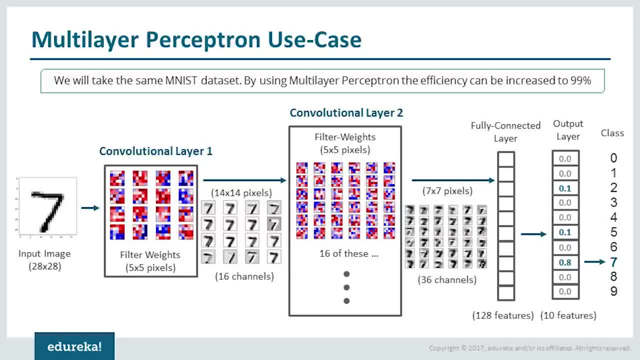 We have a separate module on convolutional networks, So you don't need to worry about it right now. So basically, what I'm doing is I'm just trying to show you that how we can increase the efficiency using the convolutional neural networks. You don't have to go in much detail. 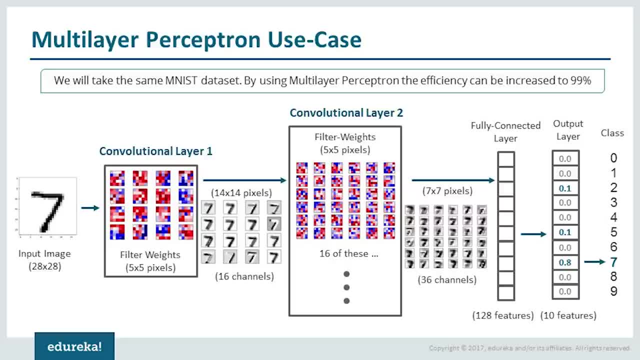 about it because we'll be learning about it in the upcoming modules. I'm just giving you a general overview, or you can say a taste, of how things work in convolutional neural networks. So we give an input image to this convolutional network, Then this input image is processed. 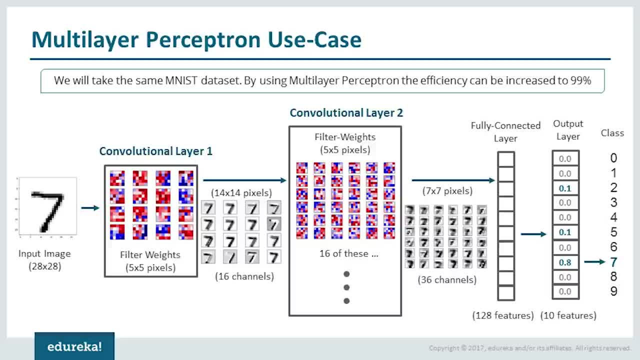 in the first convolutional layer using the filter weights. Now this result in 16 new images, one for each filter in the convolutional layer. The images are also down sampled, So the image resolution is decreased from 28 cross 28 to 14 cross 14.. 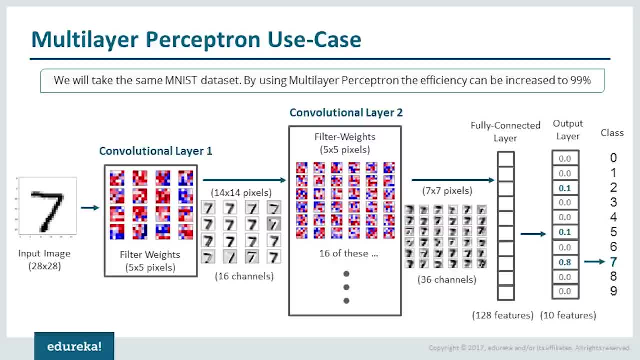 Now these 16 smaller images and from the first convolutional layer are then processed in the second convolutional layer. We need filter weights for each of these 16 channels and we need filter weights for each output channel of this layer. Now there are total 36 output channels. 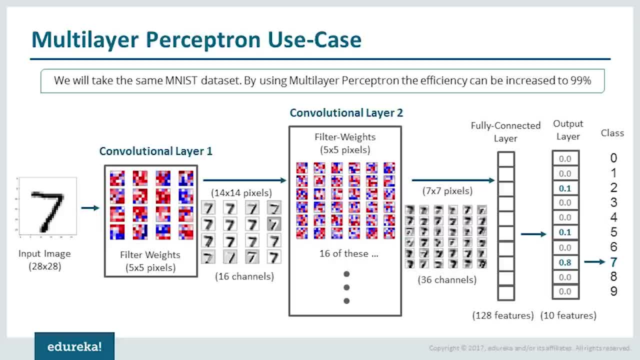 So there are total of 16 cross 36, equal to around 576 filters in the second convolutional layer. Now the resulting images are down sampled again to 7 cross 7 pixels. The output of the second convolutional layer is 36 images of 7 cross 7 pixels. 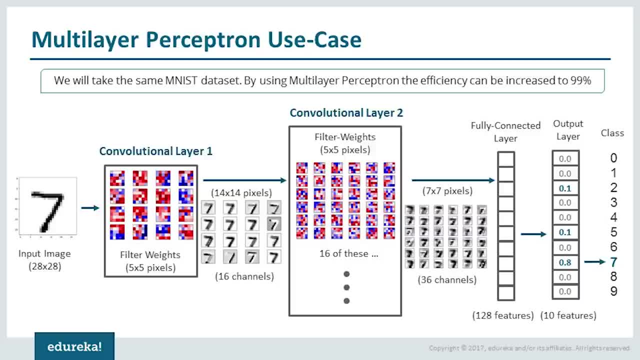 Now these are then flattened to a single vector of length 7 cross 7 cross 36, which is 1764, which is used as the input to a fully connected layer with 128 neurons And this feeds into another fully connected layer with 10 neurons. 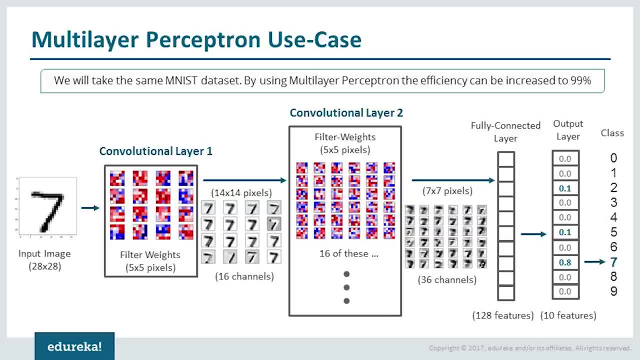 One for each of the classes which is used to determine the class of the image, that is, which number is depicted in the image. So whatever number that we provide in. so basically, the output layer, or you can say the last layer, or the fully connected layer with 10 neurons. 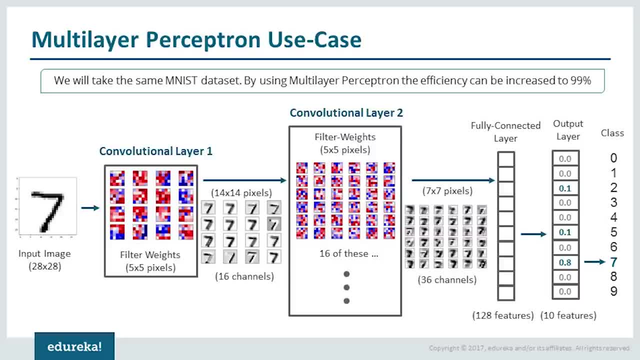 is used to determine the class or which digit is the input image of. Now, the input image depicts the number 7, and the 4 copies of the images are shown here. So basically what happens? whatever filter we have in each layer, it will be present on the image pixels. 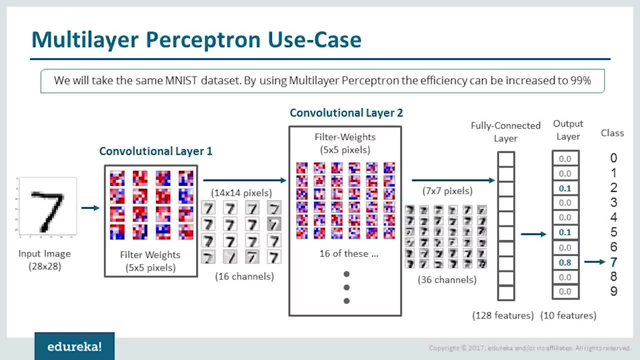 So there'll be a dot product of the filter and the image pixel behind that, So we'll get a dot product there. We are going to repeat that same process in each of these layers and for each of these layers and for each of these images. 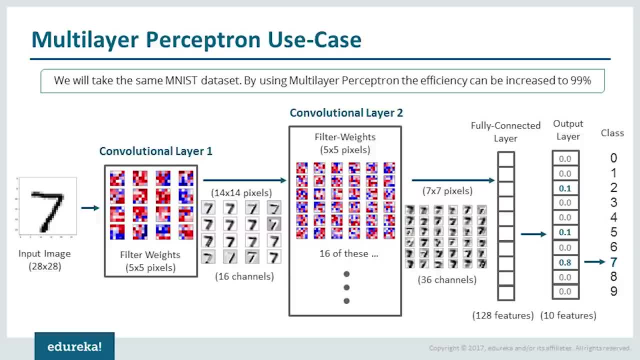 and we are calculating the dot product. So I hope you get the point and you don't need to worry about it If you're not able to understand this concept right now, because we haven't talked about convolutional neural networks at all, So I'm going to discuss convolutional networks. 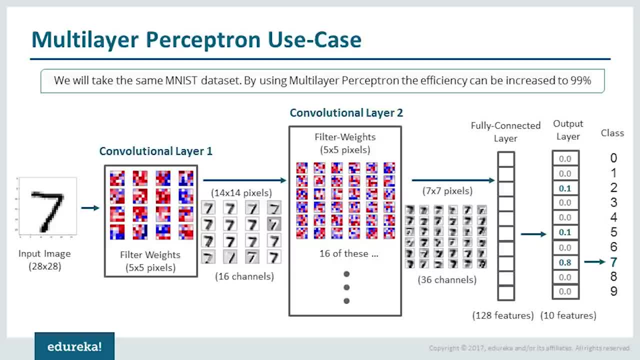 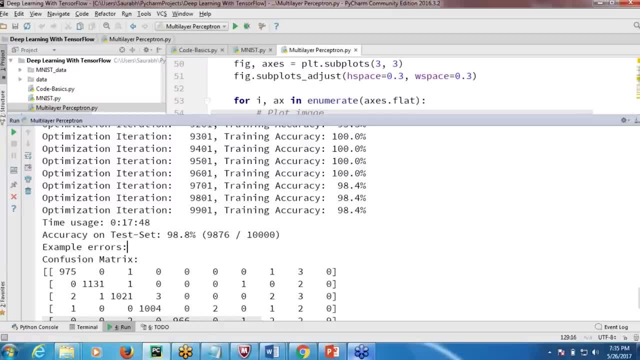 in the upcoming modules, as I'm telling you to you again and again. So let me just show you that we can increase the efficiencies. So I have already done the code and it will take time if I do it right now. So this is what the efficiency we ended up with. 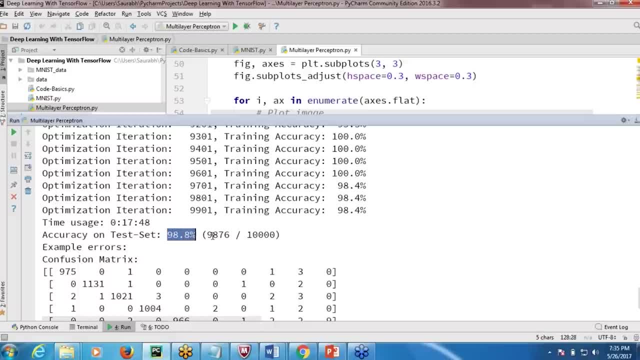 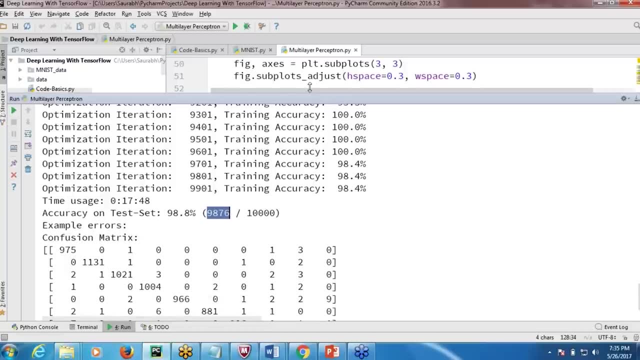 So it is 98.8%. So on the test sets, we had around 10,000 test samples, out of which we predicted 9876 correctly. So it is pretty good actually. if you see so it because in the single layer perceptron example. 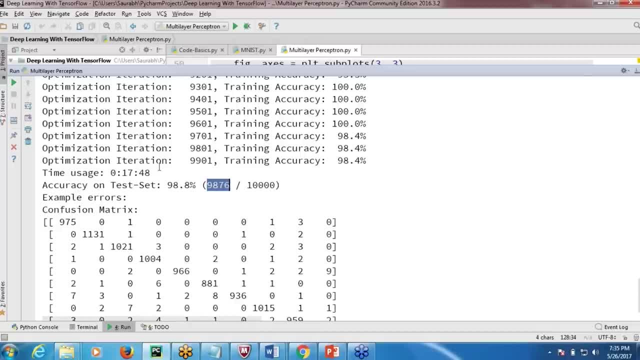 that we took, we were getting accuracy of around 92%, but here we are getting around 99%, which is actually very good. All right, So this is all for today's session, guys, and if you have any questions or any doubts, you can write it down in your chat box. 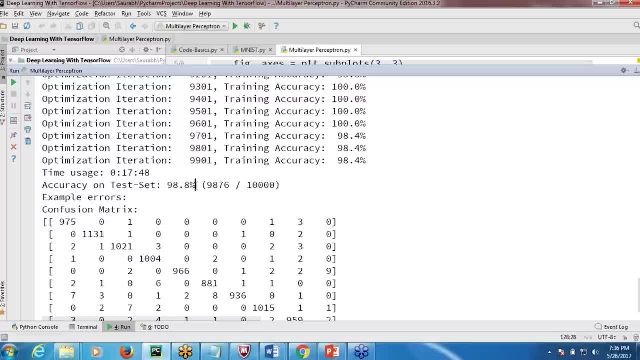 I'll be happy to help you. Pooja says: nice introduction. Thank you, Pooja. Siddharth says: amazing session. Thank you, Siddharth, for those kind words. All right, fine, So we have no questions here. So let me just give you a brief summary. 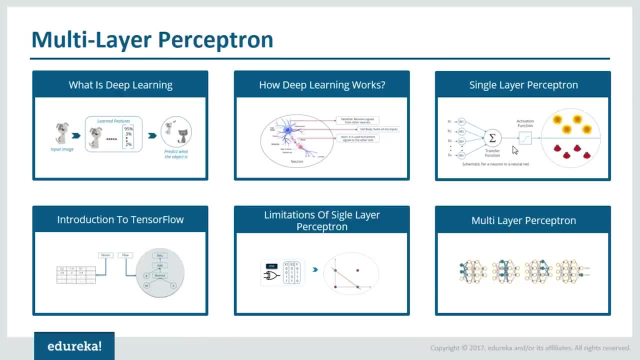 of what all things we have discussed till now. So these are the topics that we have covered in today's session. We started with what exactly is deep learning? We took an analogy of classification of cats and dogs. We understood how humans identify the difference. 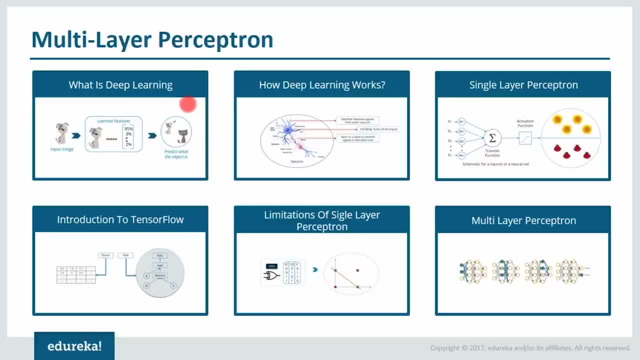 between a cat and a dog and similarly how we can train a machine to do that. So we first looked at a machine learning model and then we focused on certain limitations of that machine learning model and then we understood that what exactly is deep learning? Then we saw how deep learning works. 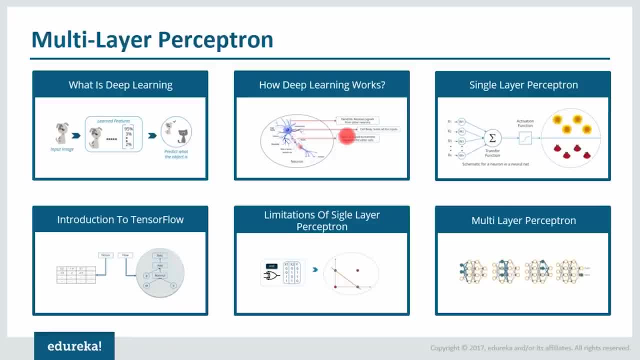 The motivation behind deep learning is your brain cells. So we understood how our brain cells or neurons work. Then we focused on single layer perception, which are nothing but the early deep learning models, or you can say, an artificial neuron, a single artificial neuron. We saw various examples of single layer perception. 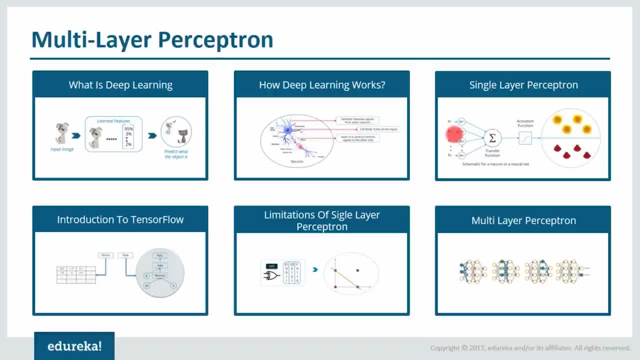 as well as, for example, how to implement AND gate and how to perform classification on the MNIST data set. Then I introduced you to TensorFlow. We understood various code basics of TensorFlow. We understood what exactly are tensors as well. Then we focused on various limitations.